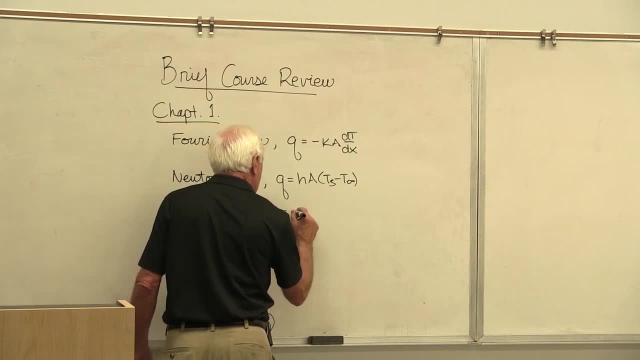 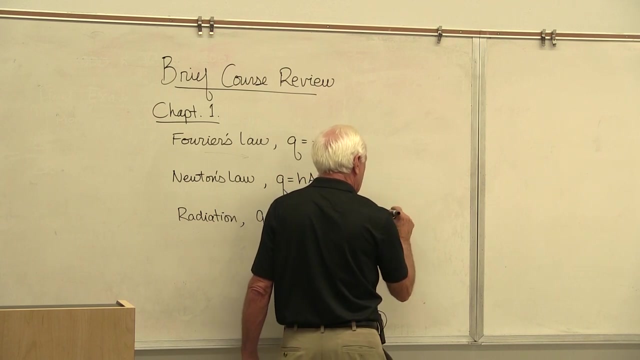 we had Q equal epsilon A sigma T surface minus T free stream, which is the fluid temperature going over the surface T surface to the fourth, minus T of the surroundings to the fourth. That equation is only valid for a small object in a large enclosure. 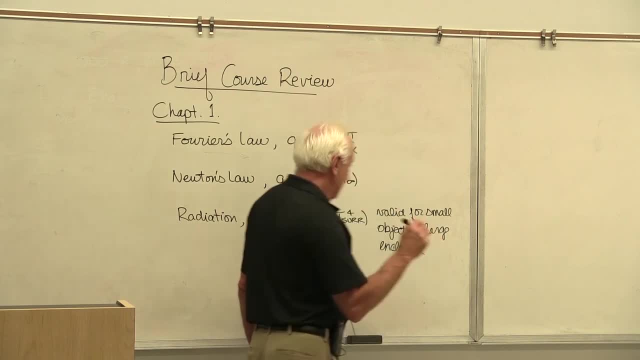 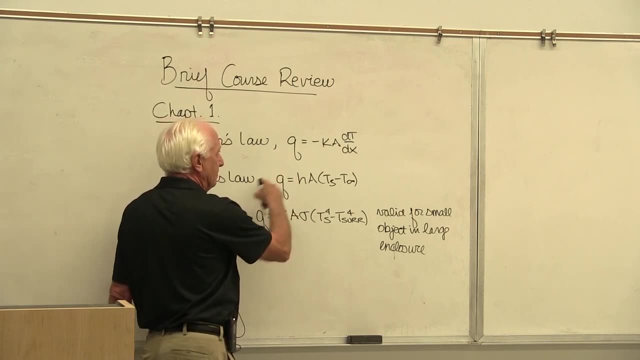 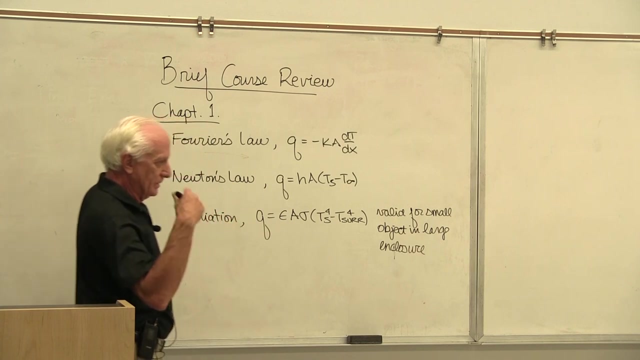 By the way, these temperatures have to be absolute. now, Any time radiation absolute temperatures- These guys in Fourier's or Newton's can mean either absolute or relative. The surrounding temperature is typically the temperature of the walls in the enclosure surrounding the object. Like I said, a small object in a large enclosure might be, if this, 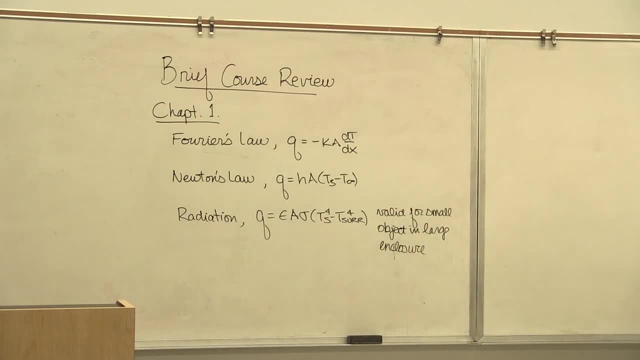 thing was a, a copper disk, and you put it here and its temperature is 650 degrees Celsius. This transfer here is zero. If you want a gender. firefighters to WrestleMania, don'tรleakolund. MRIECT Services before this activity are gentle from FARELO Powers to TESTP in much concern. And I don't want communication to be sandwiched off toofar. That system is Está Intrées, but I'm here today, So in addition to Brearley's data, you need to eat a eaten one with three inspired by sonomkind's. 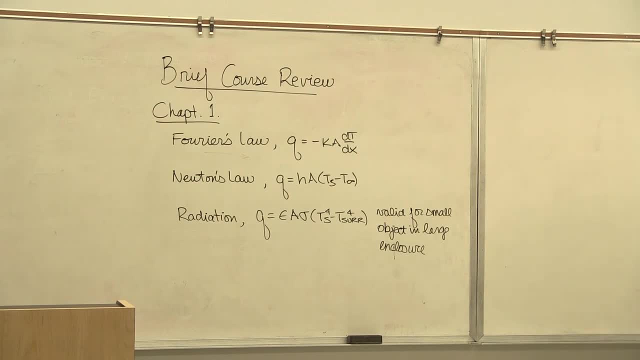 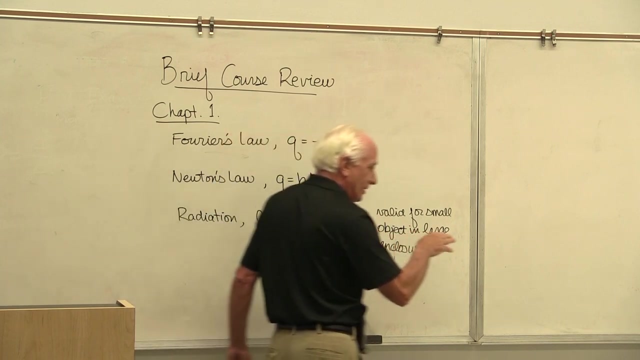 is 600 degrees kelvin and the room walls are 300 degrees kelvin. this is 600 degrees kelvin. the room walls over here at 300 degrees kelvin. we said this is only valid for a small object in a large enclosure and then later on in chapter 13 we proved it so. 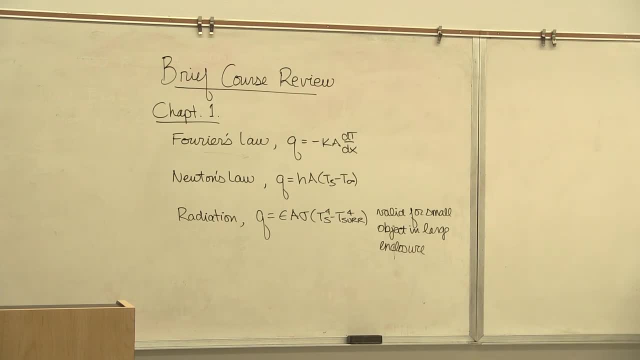 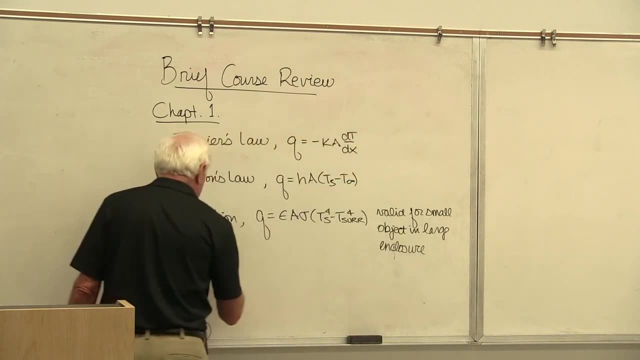 we waited until chapter 13 to prove that statement. in chapter one we just said: believe it right now, but only use it with these conditions. there was also an equation in there which said: g absorb. the incident radiation was alpha times g, so we use that in a problem for homework to. the absorbed radiation is the. 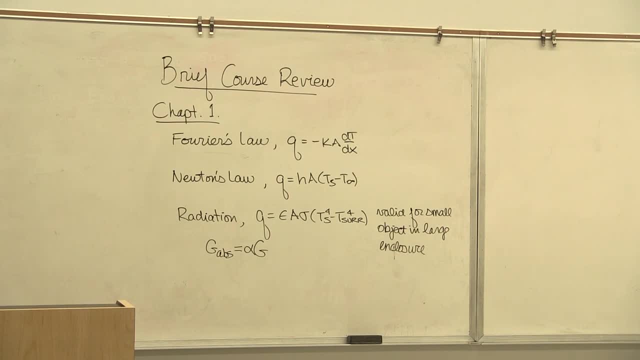 absorptivity times. the irradiation g is called the irradiation. it's also the incident radiation. that's the only term they they talked about in chapter one. they didn't mention the term radiosity or emissive power. capital e, capital j. they only mentioned capital g in chapter one. 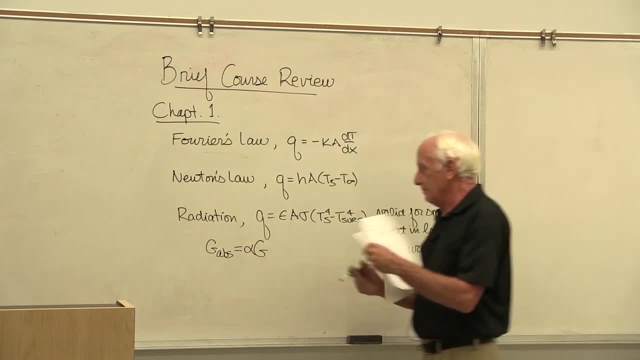 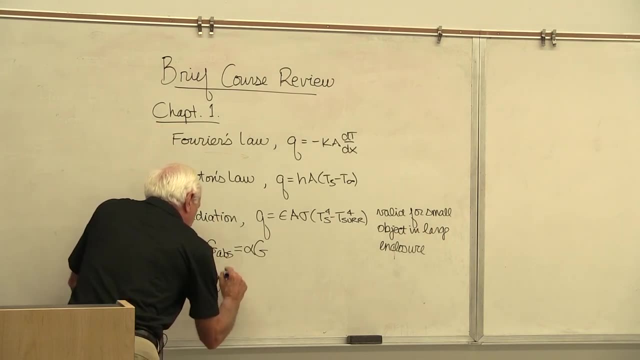 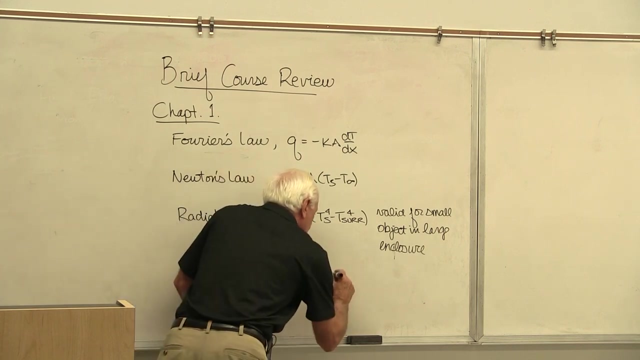 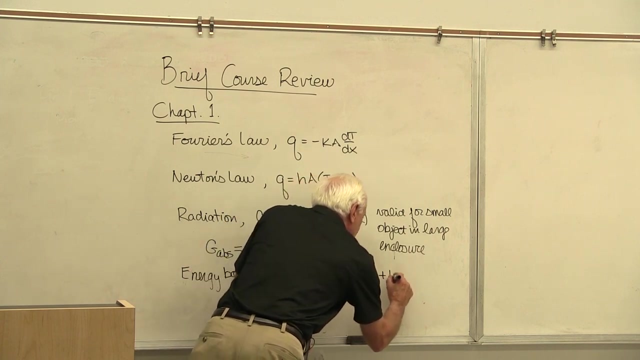 uh, let's see what else we have. oh yeah, and the last part of chapter one was um energy balance for a control volume which was e dot in, e dot out plus e dot gen equal e plus e dot. this is e dot gen equal e dot storage. 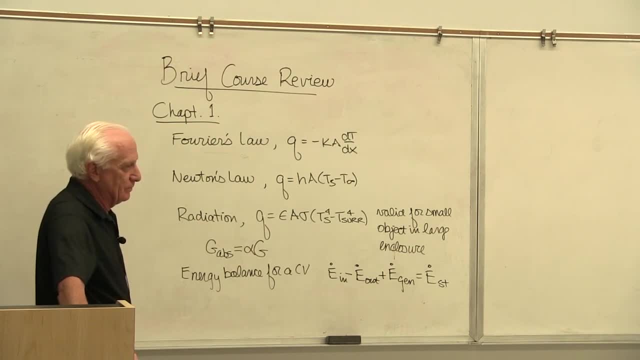 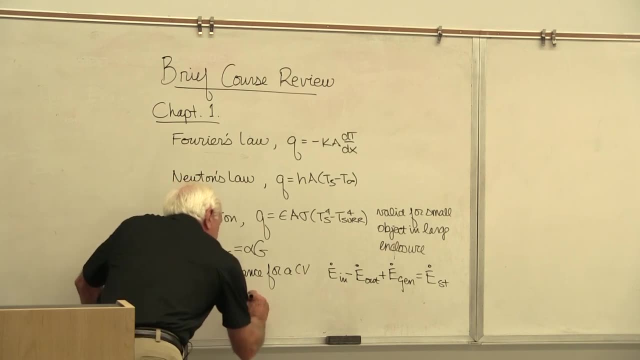 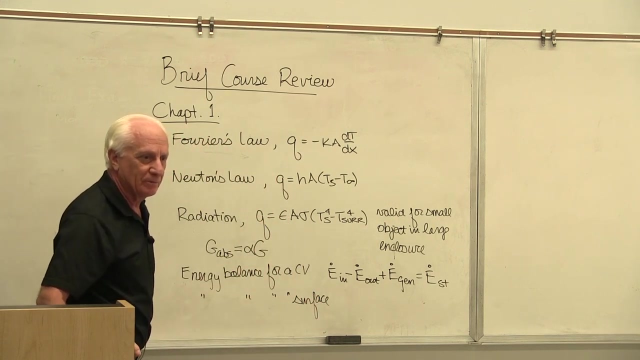 e stands for energy joules. the dot means per time, joules per second watts. those guys are in watts. uh, energy balance for a surface, a surface we assume to be infinitesimally thin. its volume approaches zero, its mass approach is zero. so it can't store energy because storage is m times c, sub e. 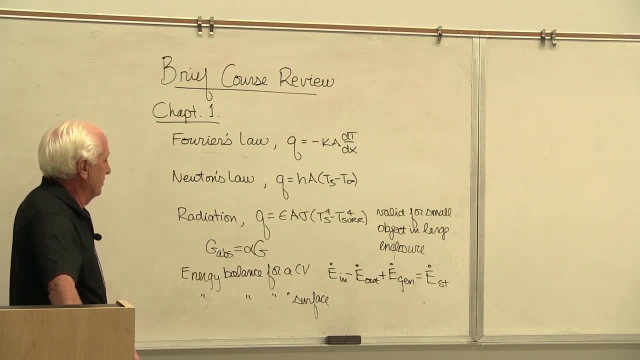 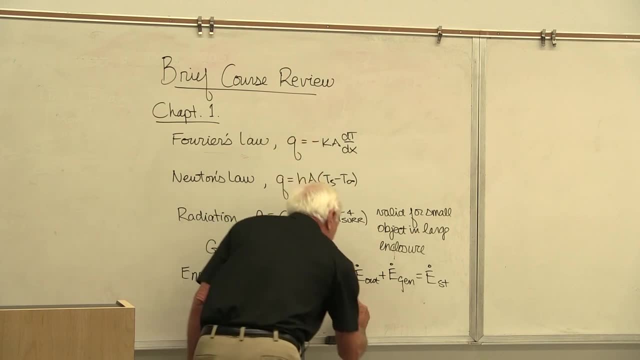 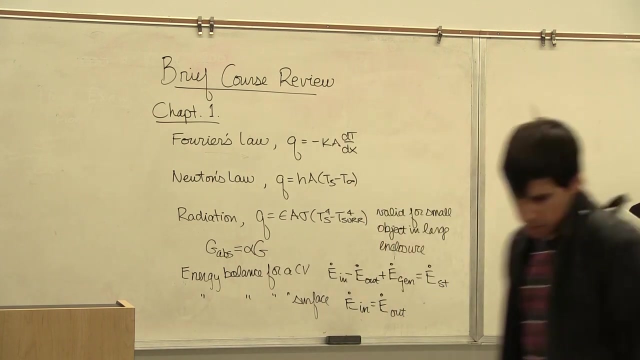 if there's no mass, there's no storage. so for a surface, then the e dot storage term goes to zero, the e dot gen term goes to zero. we're left with then e dot n equal e dot out. okay, so that industrialized chapter one and we work problems which involve all. 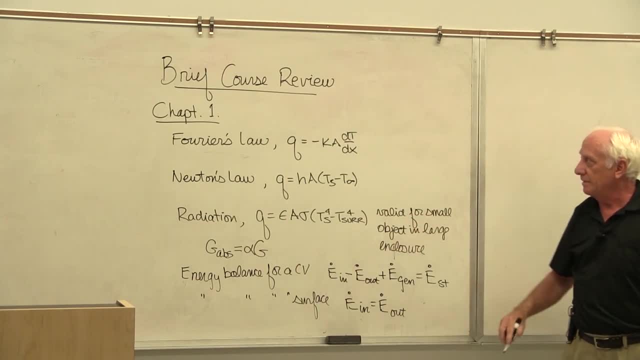 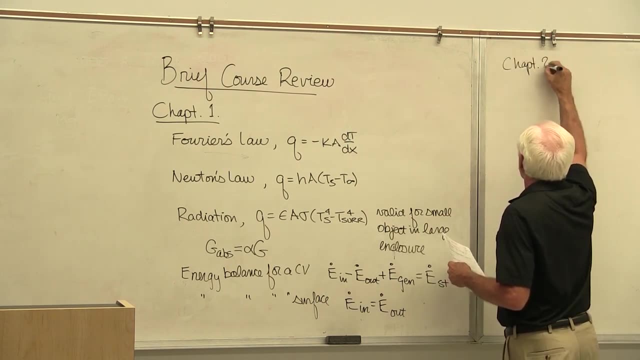 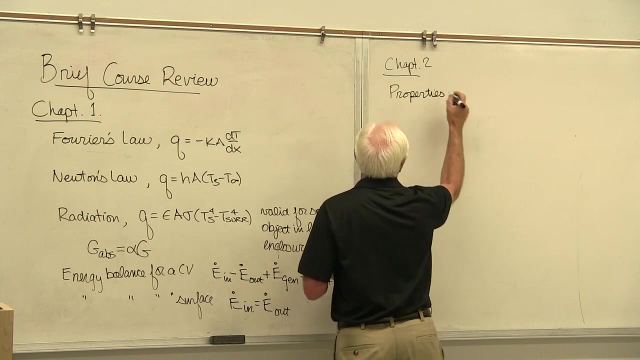 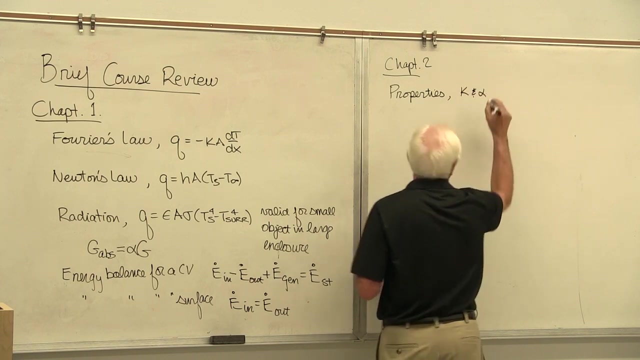 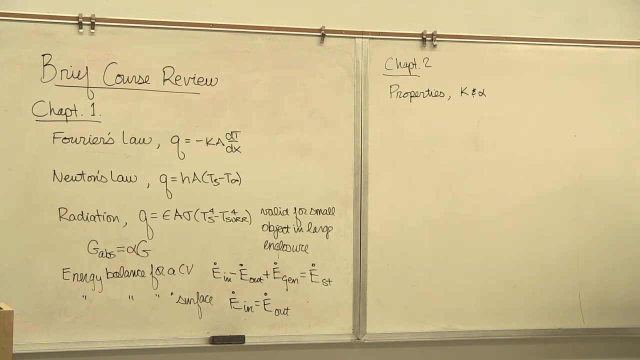 three of these equations- fourier's law and luther's law- and radiation, uh, chapter two. we started off talking about properties and uh, especially k and alpha thermal diffusivity, alpha thermal conductivity, k. there were a lot of other properties but they weren't, um the most important ones in the heat. 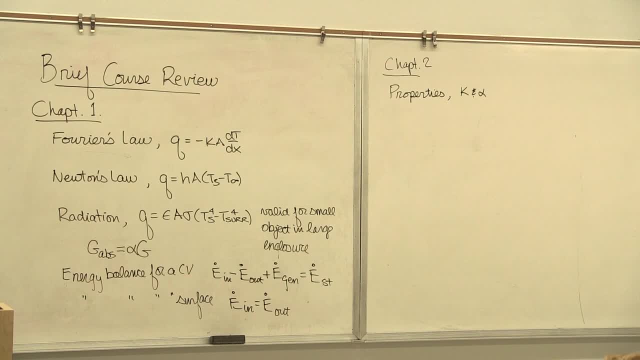 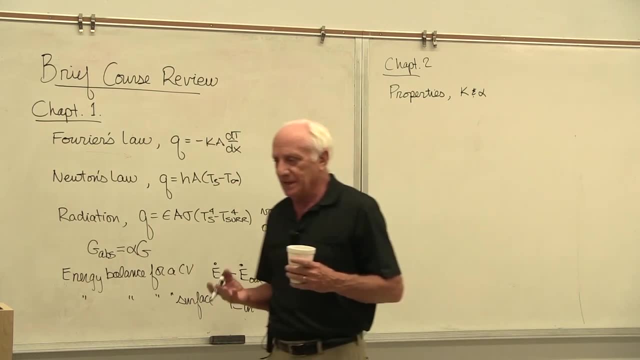 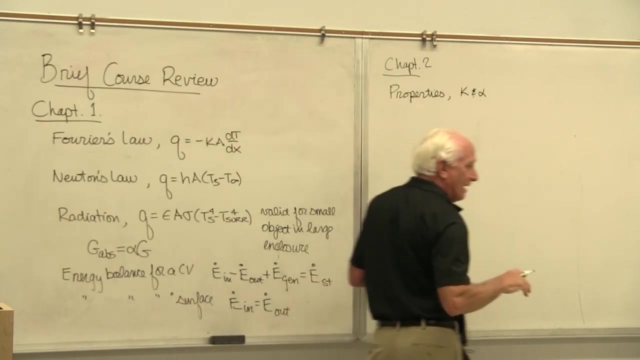 transfer group are k and alpha. there's other properties that are important, for instance mu and nu viscosity, but that's blue mechanics. then we have c sub p, that's thermal. so there's other properties, but we focused on these two in m415. we looked at graphs of those properties, how they vary with temperature. 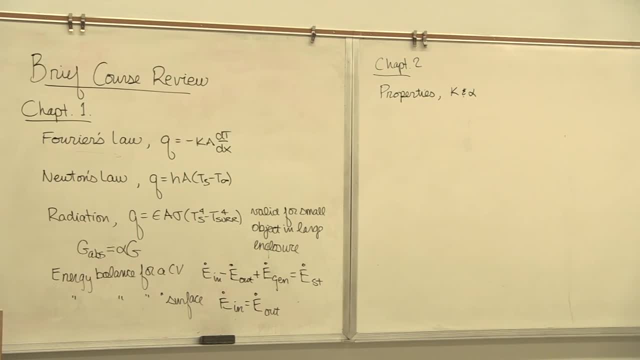 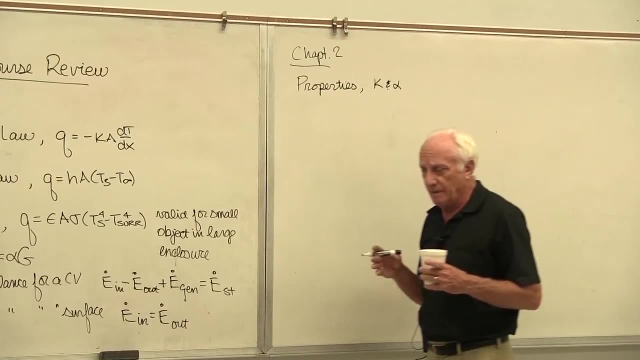 for solids, for liquids and for gases. we went to the back of the book. in the appendices, we found out how to find the properties, how to interpolate the values as a function of temperature, and the one table which was the most difficult to read was for water. 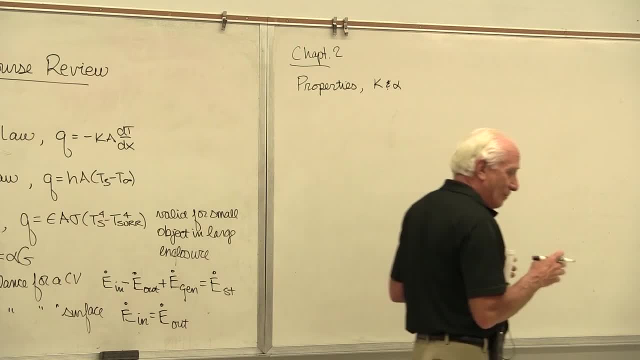 because in the water table there are properties with the subscript f and properties with the subscript g, u, sub f, muc of g, k, sub f, k, sub g, bb. f stands for saturated liquid, and now we're going to look at the properties in the toutes, and so that is. 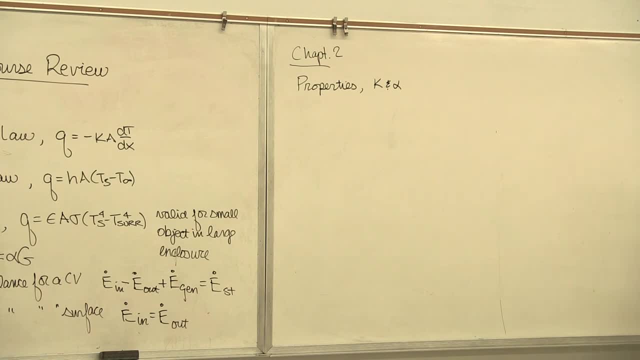 up. another side of the equation is- and we'll take one more step on the usual example and maybe you'll come back to that and take a second look- and says: yeah, look, if you lost это. The G stands for saturated vapor. We assume water behaves as a saturated liquid. okay, 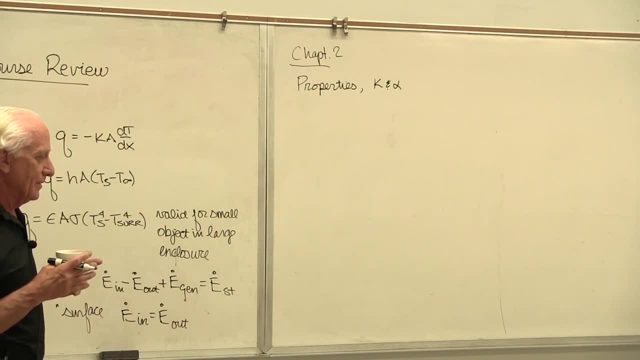 So we use all the properties with the subscript F in that table. There's a little v in that table. Little v stands for specific volume, the reciprocal of density. So if you want density, take the reciprocal of little v in the table for water in the 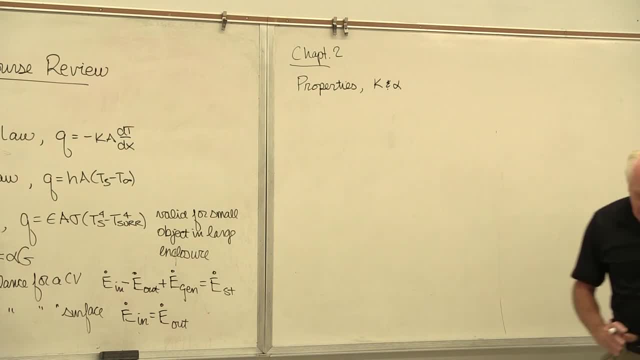 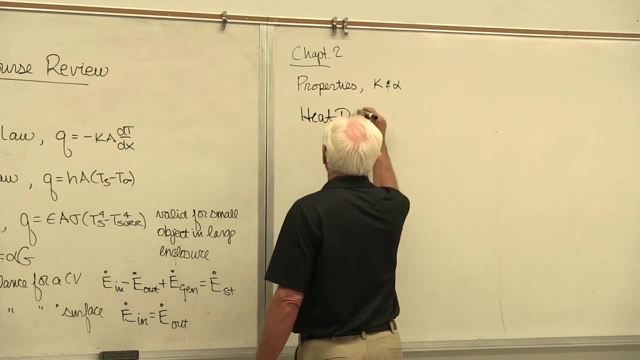 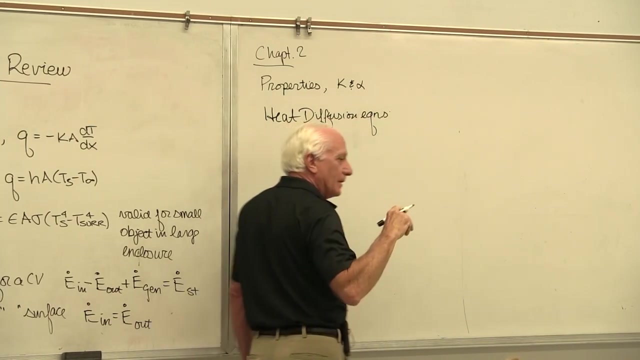 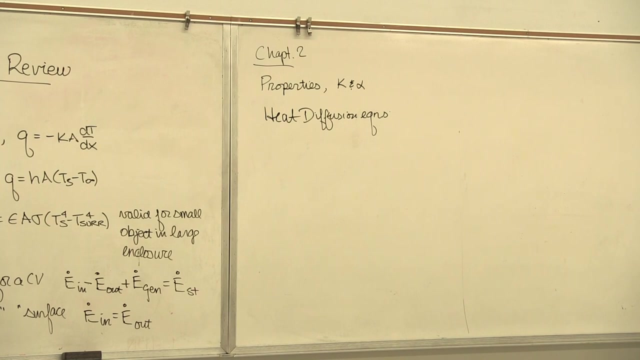 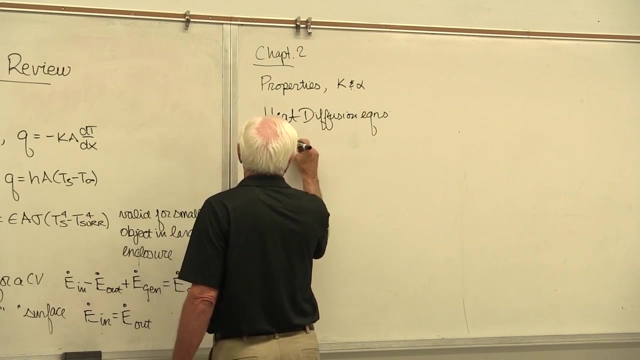 back of the book. Then we had the heat diffusion equations. Now they're the governing partial differential equation or temperature as a function of, typically, the coordinates. We had one of these for a rectangular system: x, y and z. Okay, 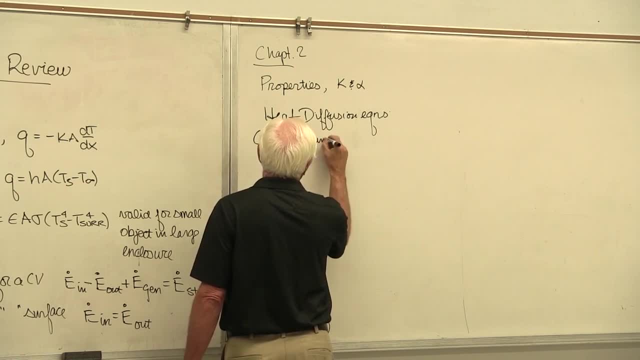 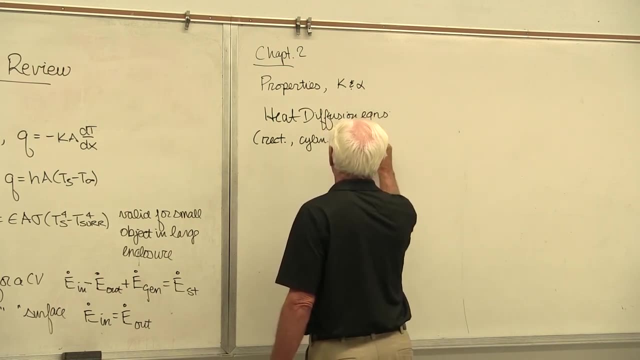 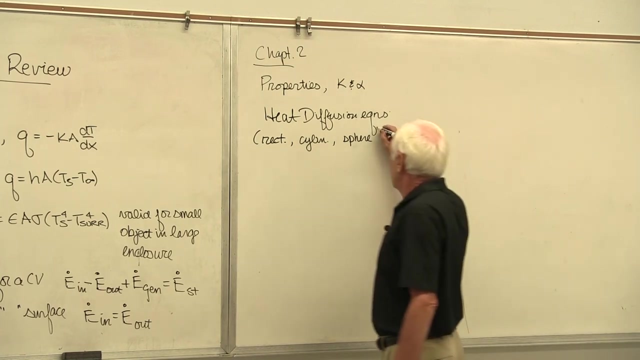 We had one of them for a cylindrical function of radius angle and length, And then we had one for a sphere. So there were three different heat diffusion equations, depending on the geometry. Okay, Let's see. Yeah, Then to solve that we needed to apply boundary conditions and possibly initial conditions. 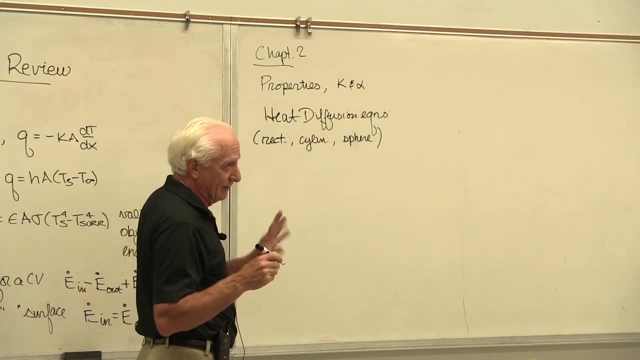 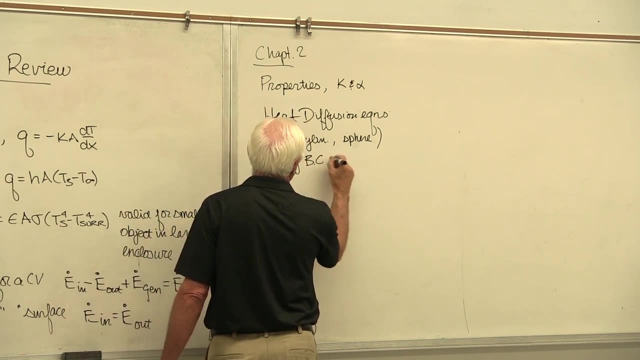 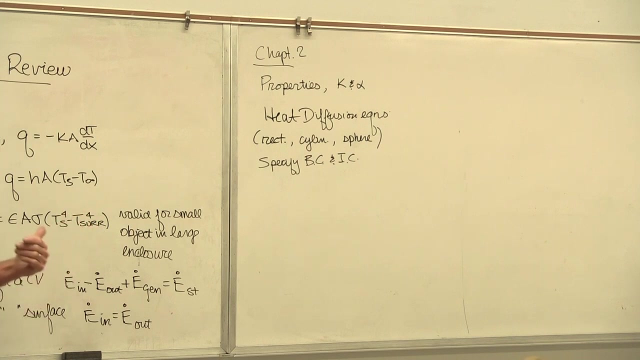 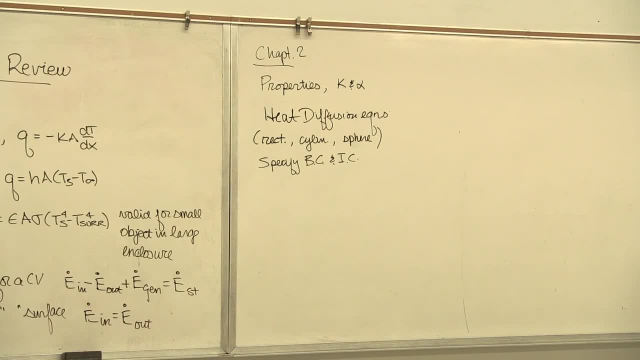 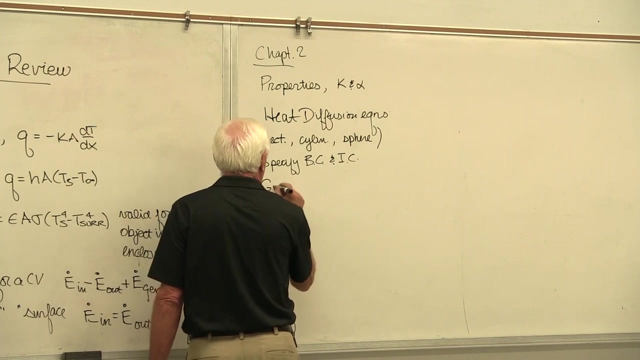 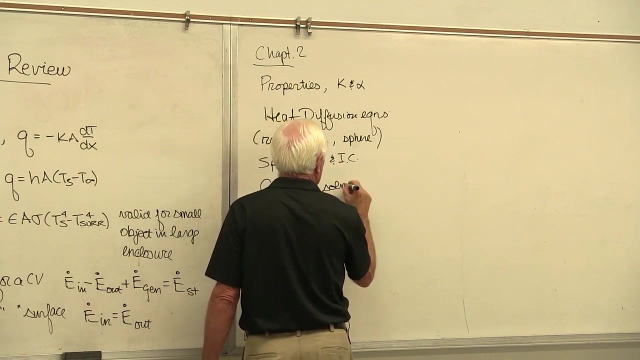 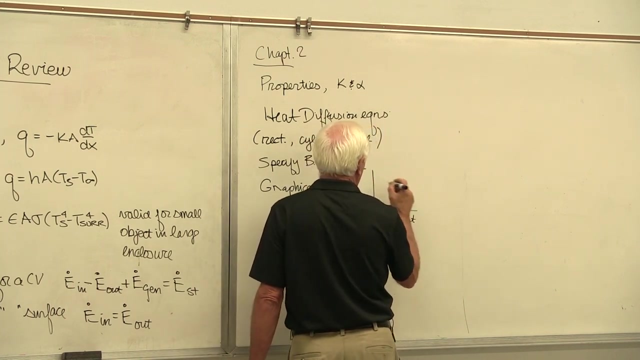 wall temperature if it's convection at the wall, whatever the boundary condition might be if it's adiabatic wall. and then we did some graphical solutions. they weren't really solutions, they were things like plot temperature as a function of time and they might vary. 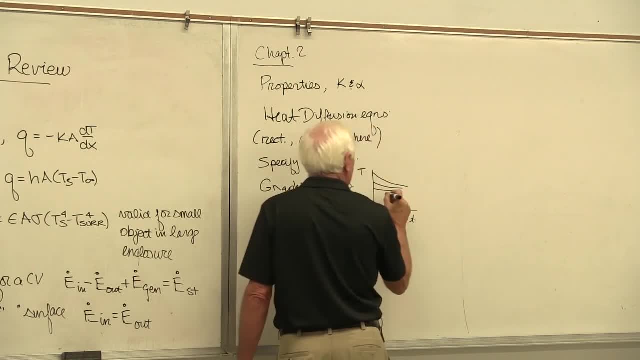 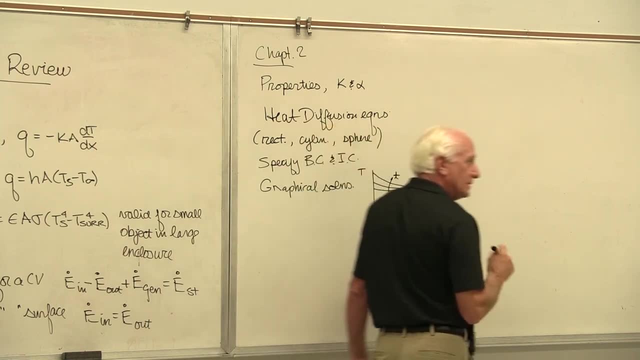 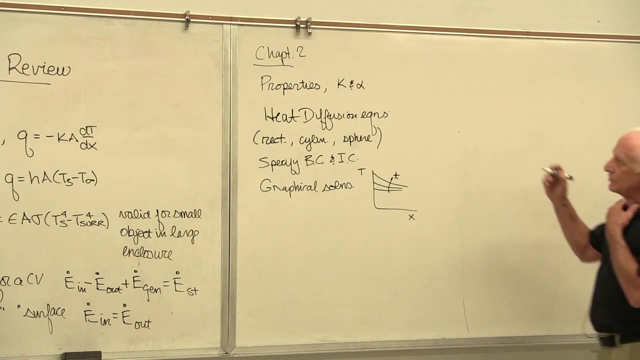 something like this and it was a function of X or different times. so we did some plots like that. it's a class of examples. you work some problems. so chapter 2 is relatively short and that was all pretty much the high points in chapter 2. now we go to chapter 3, a much more lengthy chapter. 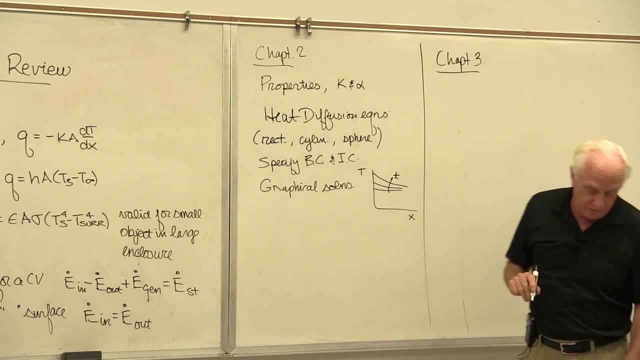 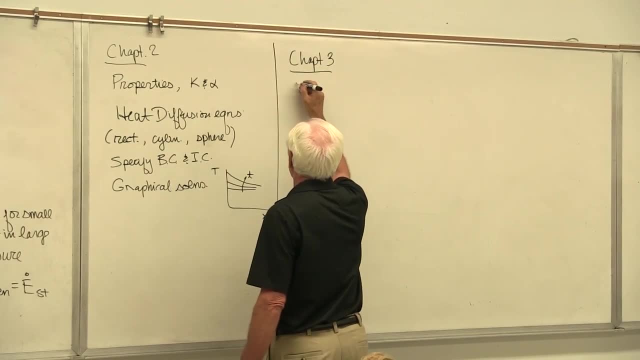 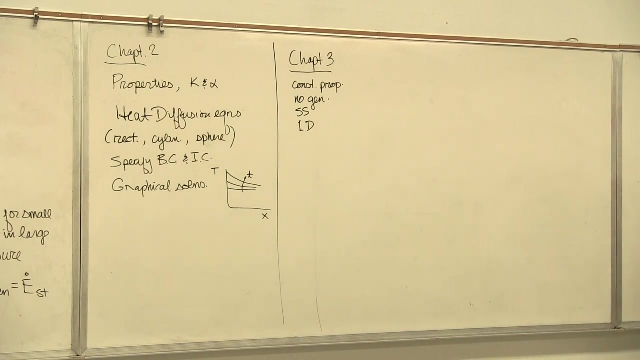 okay, chapter 3. we start out with a few assumptions. we pretty much assumed constant properties, no generation, steady state and 1d heat conduction. those are the four main properties we use to derive some important equations in chapter 3. the equation we derived from chapter 3 is that we have a constant temperature. 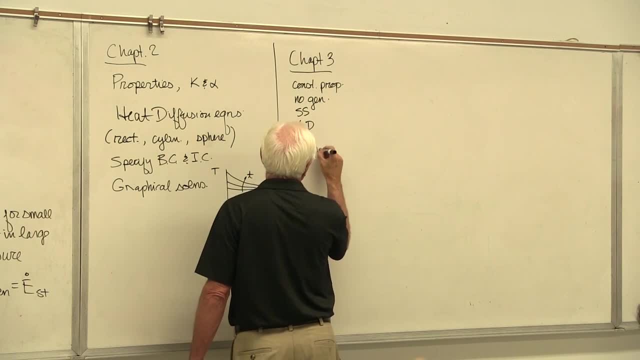 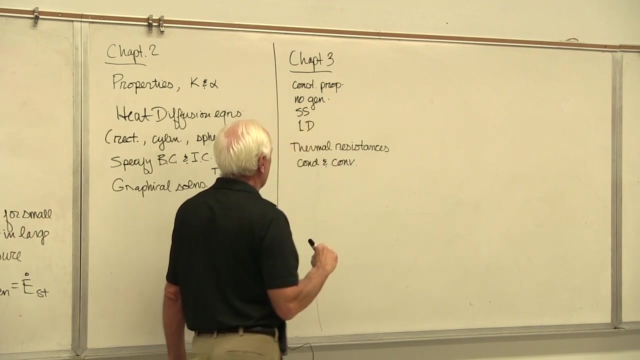 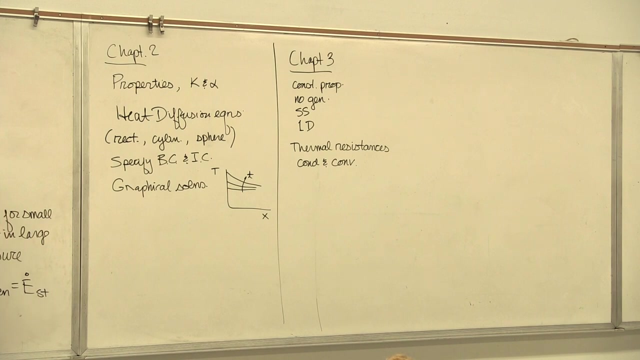 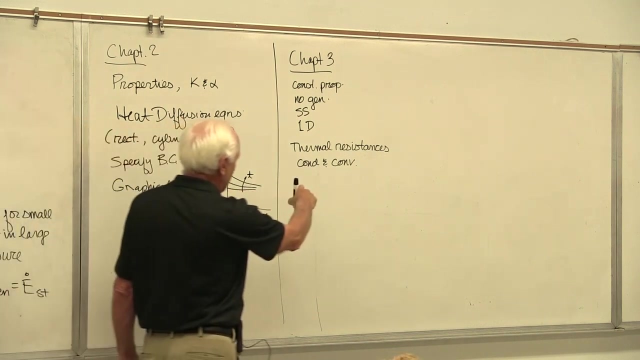 the equation we derived from chapter 3 is that we have a constant temperature, resistances or resistances. we have those for conduction and convection. this guy here, if it's 1b because assumptions over there, this guy becomes delta T over Delta X. So the resistance then was L over KA. for conduction There's also one. 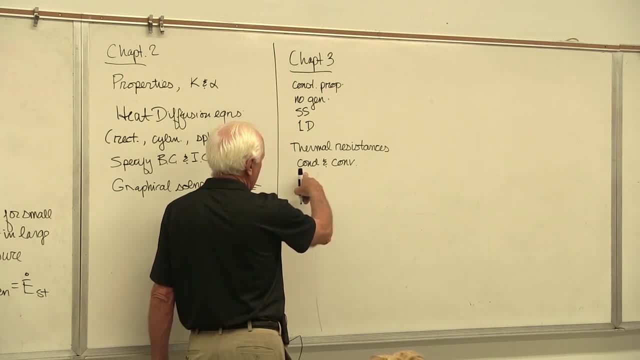 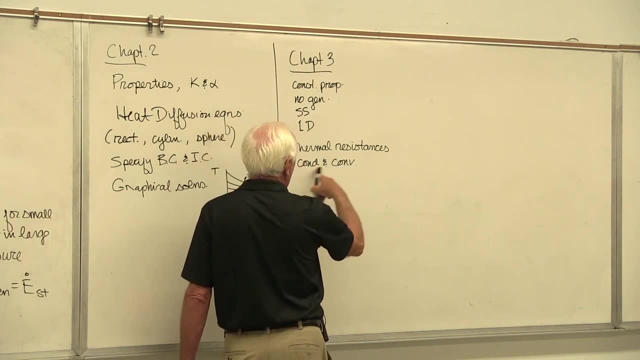 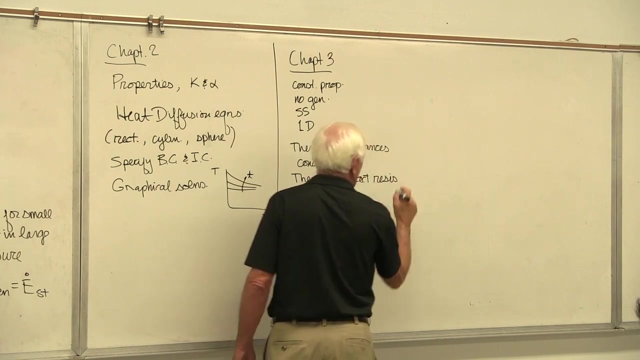 for spherical and one for cylindrical Convection, one over HA, one over HA. So we have a number of different resistances And we also have thermal contact resistance. If two materials are brought together, there's going to be some air pockets in there. You can't press. 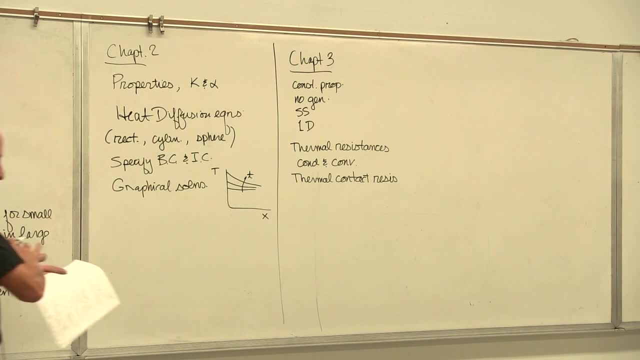 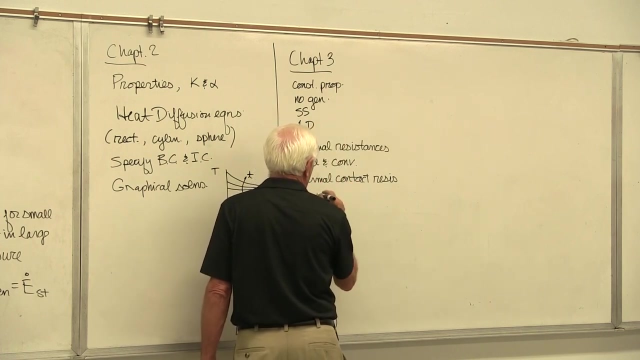 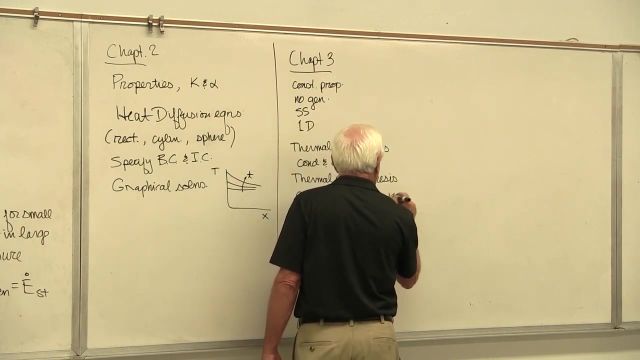 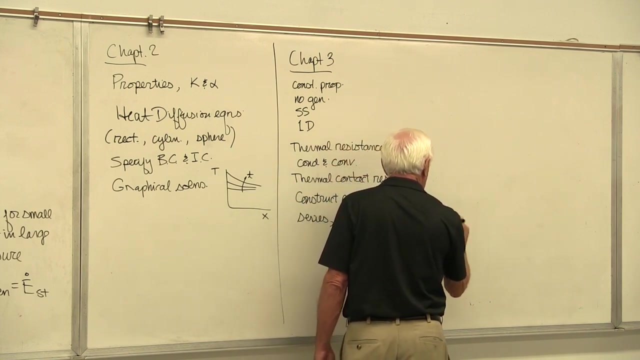 them together, perfectly Roughened surfaces for instance. So those trapped air pockets create more resistance and we call that the thermal contact resistance, And then we freeze all together and we construct a network. It may be a series, combination of resistances, or it may be parallel, or it may be series, parallel, Classic series. 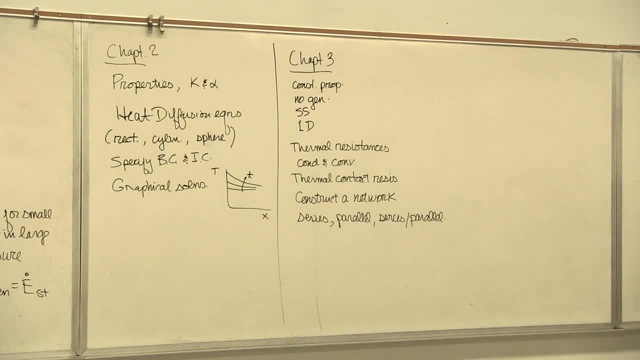 parallel is the wall. The outside might be stucco and chicken wire. Then you go into the wall where there's the studs and the insulation between the studs. They're in parallel. Then you go in series out through the interior walls of the room. So yeah, construct a network of that. 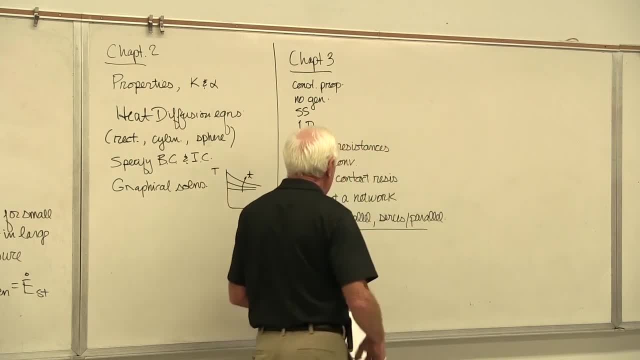 And I think, yeah, that was pretty much the first part of Chapter 3.. Now, what that leads to, we have Part 3.. Okay, Part 1 is: what's done here is an extension of these two things. Now we're going to look at this first. 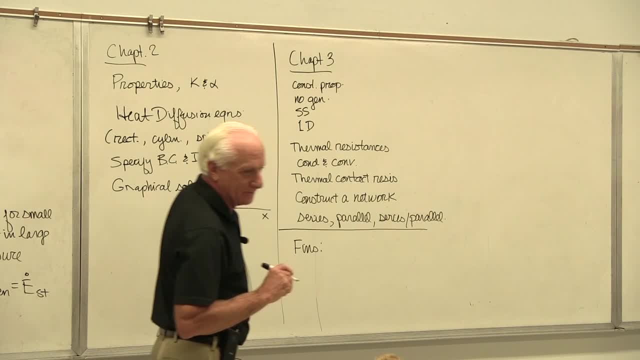 The second part is: how do we tackle fins. The third part is how do we tackle fins. We're going to run one of these out, and the first part is how do we tackle fins, So I'll show you how to do it. 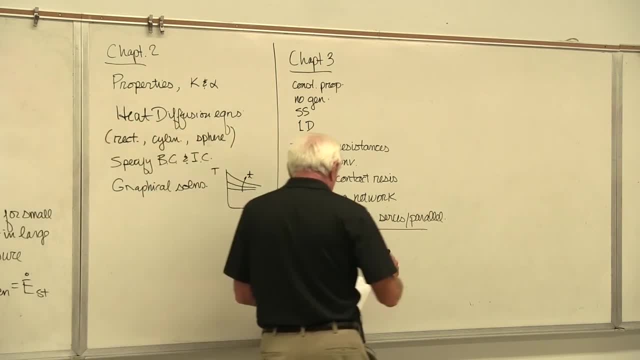 What we do here. the first thing is: how do we tackle fins? They're called extended surfaces, Fins. First of all we have Table 3-4. Then we have Figure 3-18 and 3-19.. So we have these two. 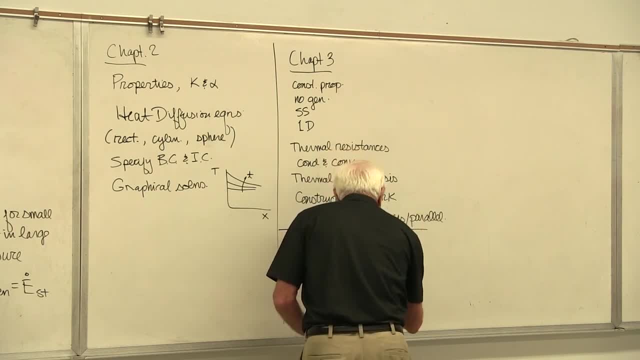 Then we have Table 3-5,, then we have Table 3-5,, then we have Table 1-2, and okay, So that's how we tackle. So we have the pieces and we can noodle this down. 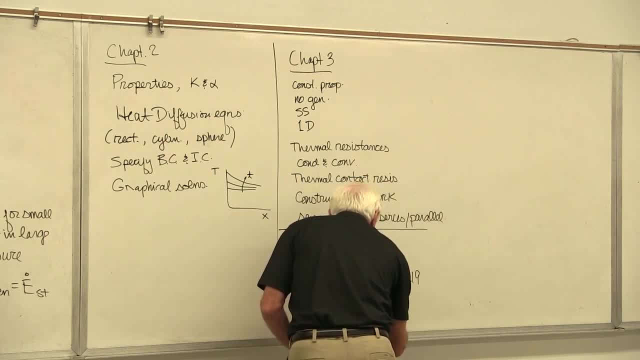 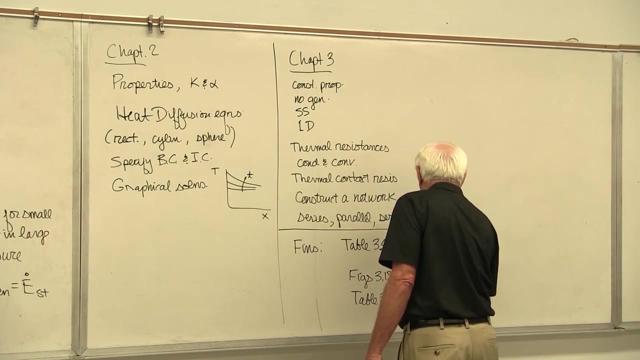 Then we have Table 3-5.. Okay, Now, Table 3-4 will give you two things. It'll give you, if you want, the temperature, and it'll also give you the heat transfer from the bend Q, So it'll give you the temperature as a function. 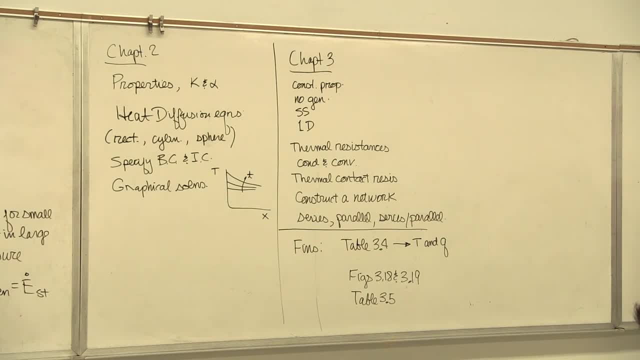 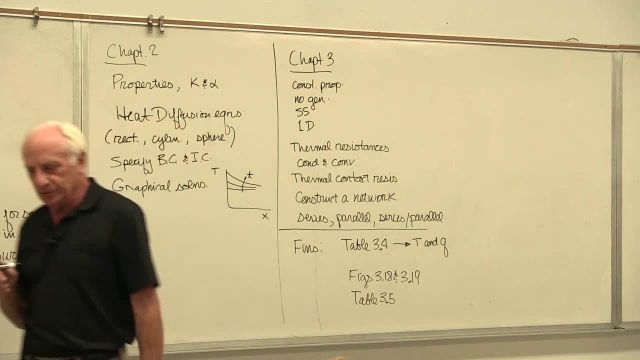 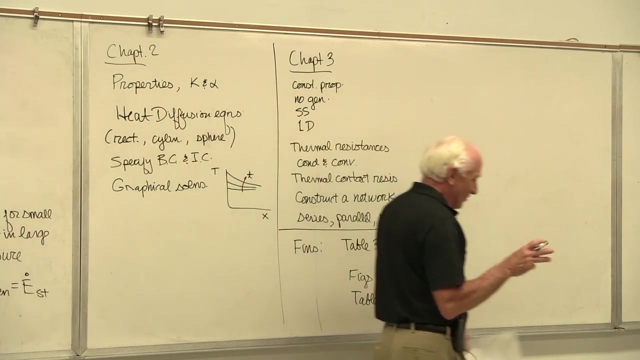 of X or radius and Q. There's four cases in that table: One, convection at the tip. Number two, adiabatic fin tip. Number three, prescribed temperature at the fin tip And number four, which is a model for an infinite fin. 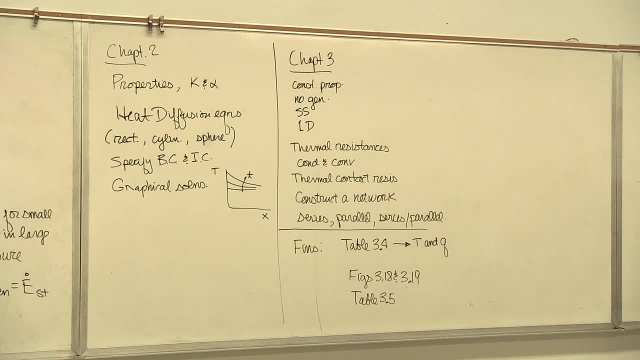 if ML is greater than or equal to 2.65.. If you want to use Figure 318 and 319, or Table 3-5,, then these guys will give you the fin efficiency, not Q. The fin efficiency. If you want Q, then 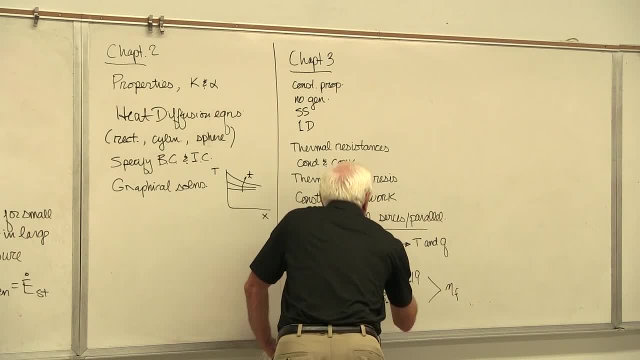 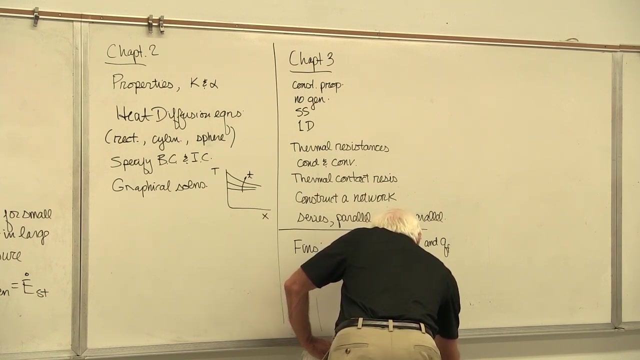 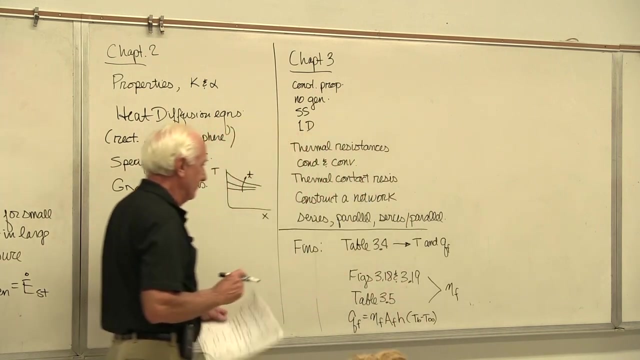 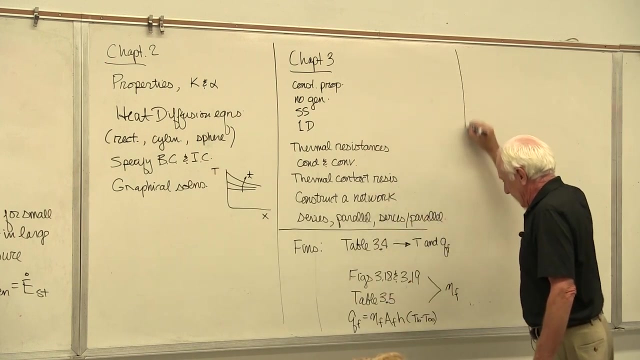 put efficiency in this equation, Q-fin is equal to the fin efficiency times the area of the fin times, T base minus T-infinite. That's how you get Q-fin, And the last thing about this is we have fin arrays, For instance, 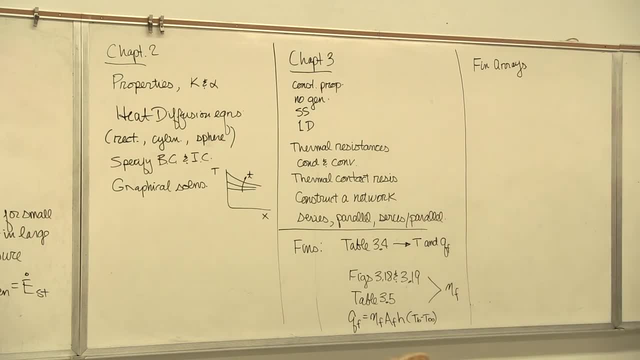 there's a. let's see. I put 100 pin fins, Each one two millimeters in diameter. They're five millimeters long on a one by one square meter base. How much heat's lost by the whole fin array, including the fins plus the base? 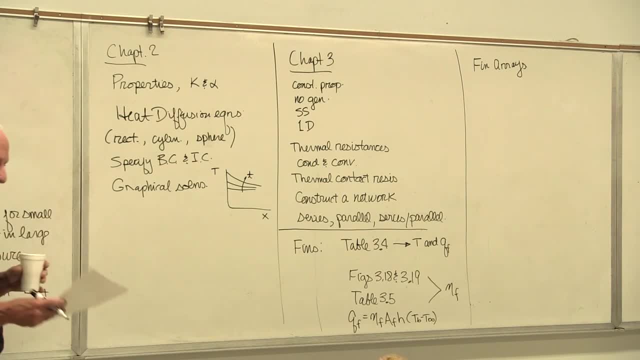 100 fins plus the base area. So that's a fin array. I've got a tube with fins spaced at 10 millimeters apart. There's 50 fins on that tube. How much heat's lost by that tube? That's a fin array. There's some tube wall area. 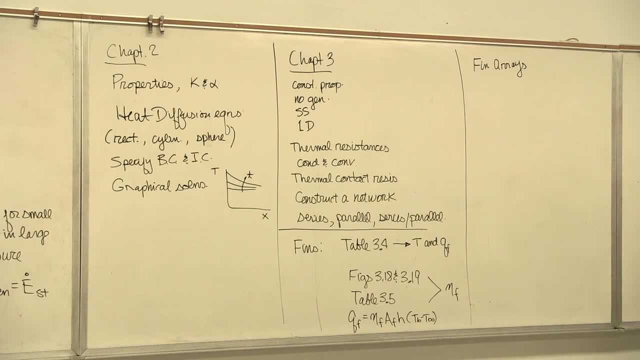 and there's some fin wall area or fin area. Okay, And know how those temperatures look, Exponential in appearance, Exponential with X, Not linear. Know how the temperatures look here. Okay, If you're here, if you're here with these assumptions, don't forget. 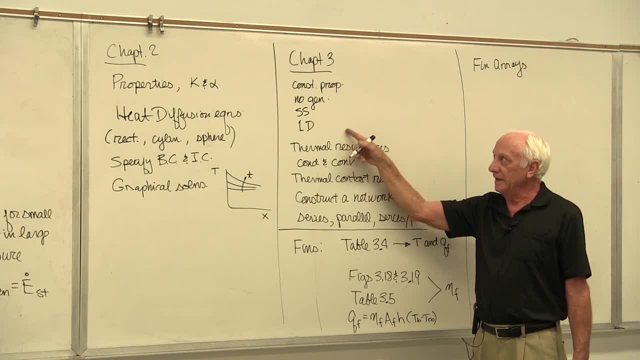 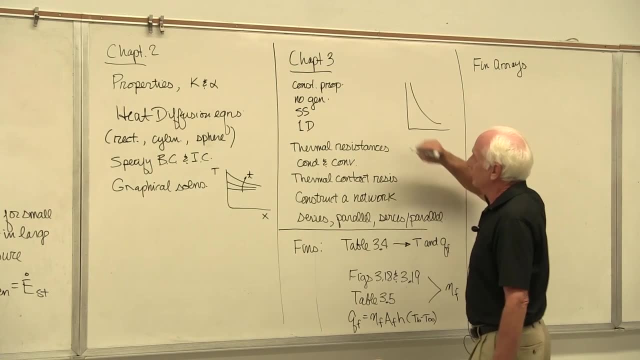 the temperature gradient is linear in X. If it's radius, then we have those graphs Like that. If it's radial, it looks like that If it's rectangular, So know the shape of the temperature profiles of the material too. It's important. Fin array. that wraps up chapter. 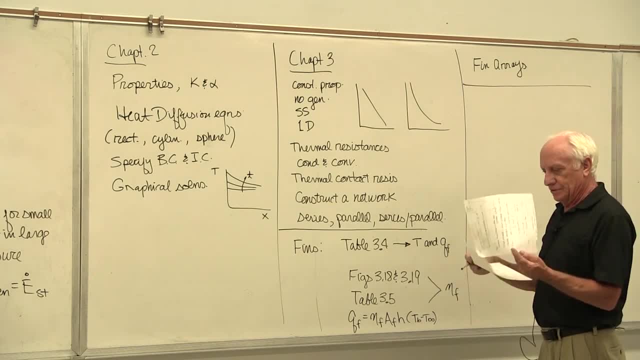 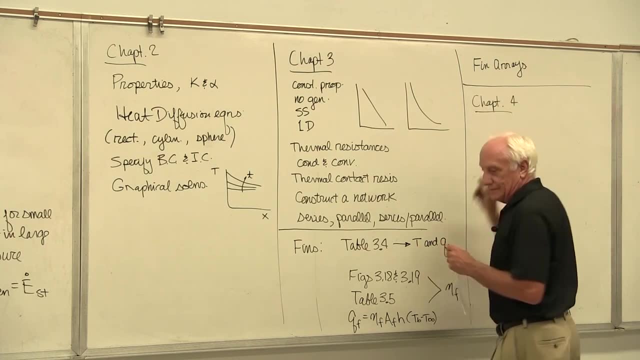 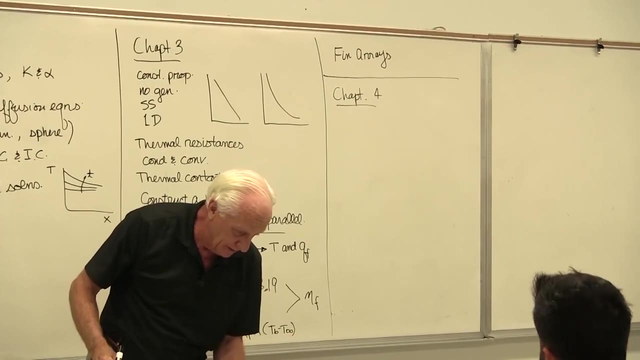 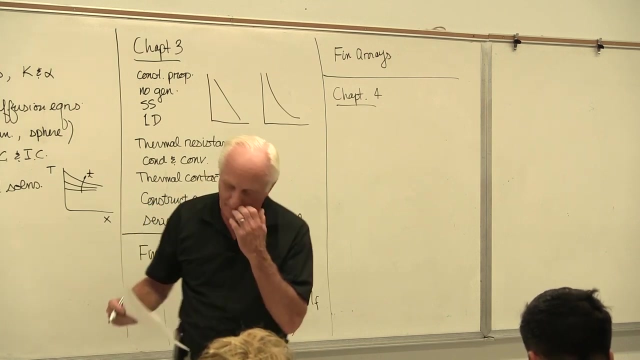 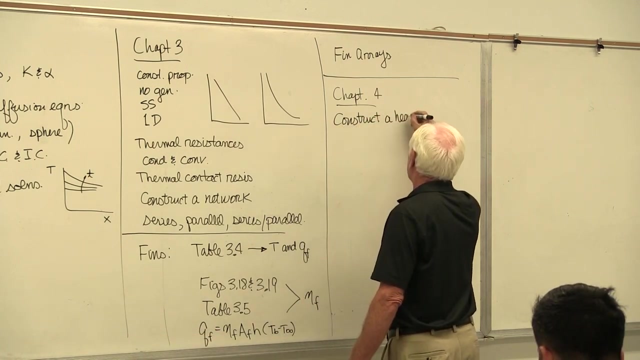 three then. Okay, let's go on to chapter four. Now let's see, I don't have my notes on that, but I can find out from four here. It's a really short chapter. Okay, first thing is construct a heat flux plot. 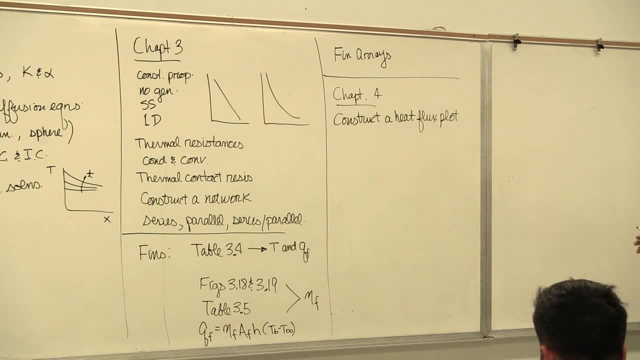 A heat flux plot is a plot that shows a solid material and on that plot there are lines. Some are called isotherms, they're constant temperature. Some are called adiabats. They're the way heat flows. Adiabats are heat flow lines, Isotherms are constant. 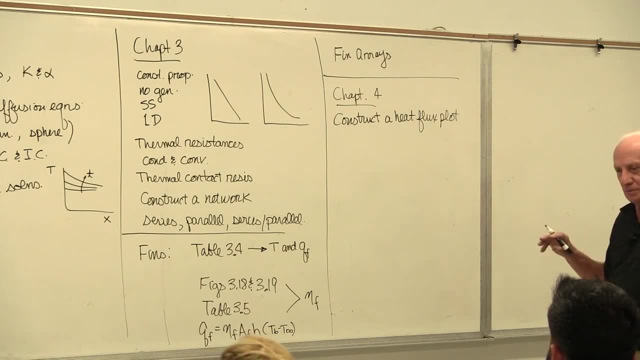 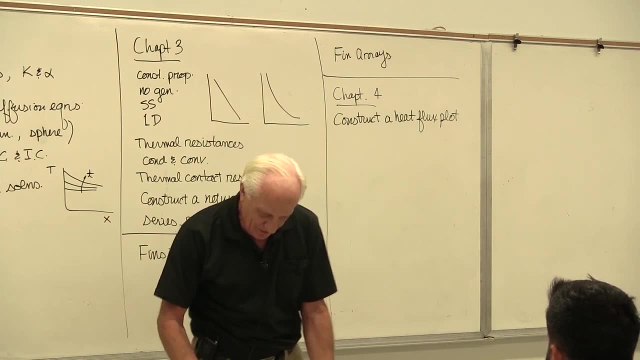 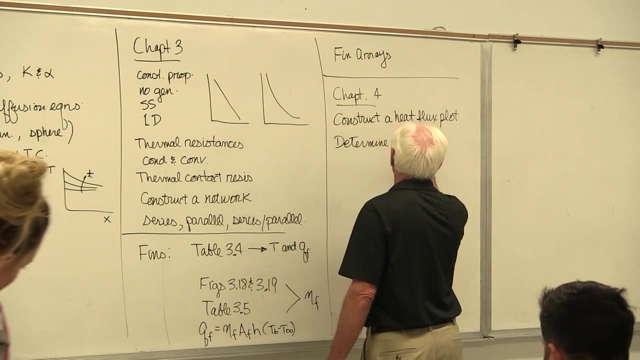 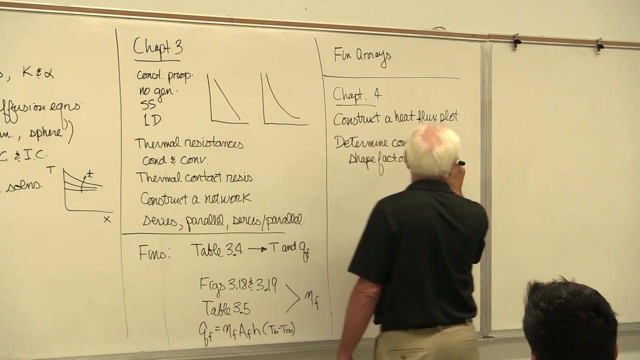 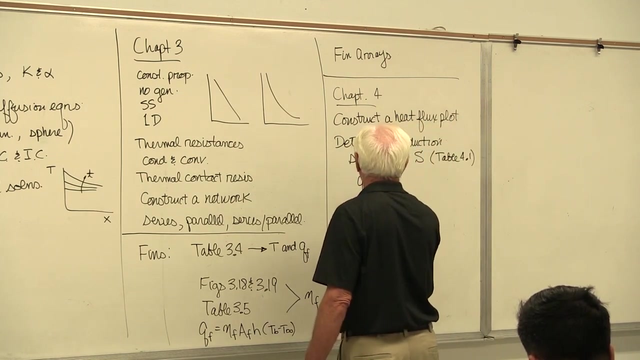 temperature lines, Construct a plot- We've done that multiple times, Okay- And second, determine the conduction shape factor And those conduction shape factors in table 4-1, which we've got in the package. Then use that S to get Q. 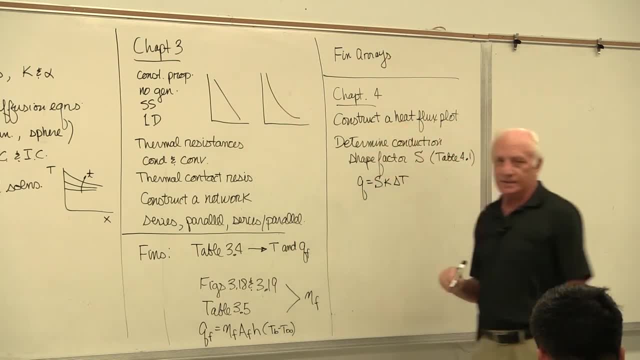 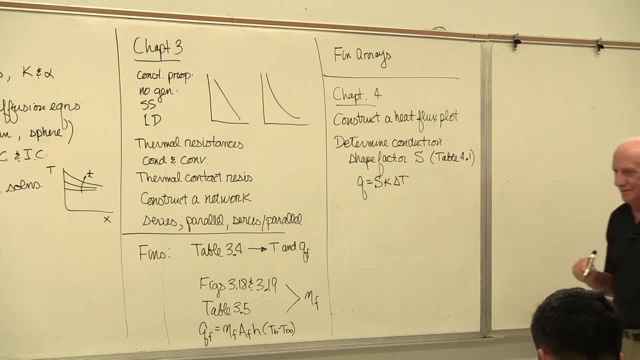 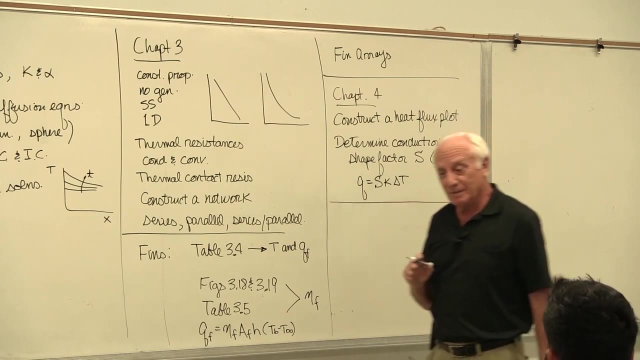 SK delta T, SK delta T. Really straightforward, Very simplistic, Minimal math. Find the picture in the table, Get the S value, Play the equation, You've got it. That ends chapter four. On the final, nothing to do with numerical methods. 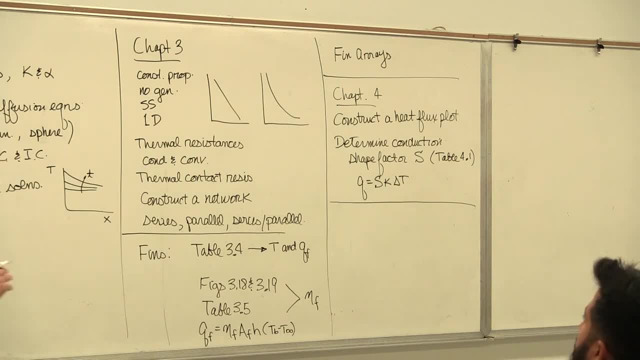 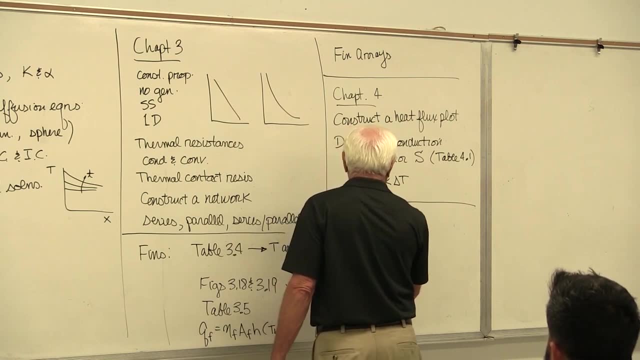 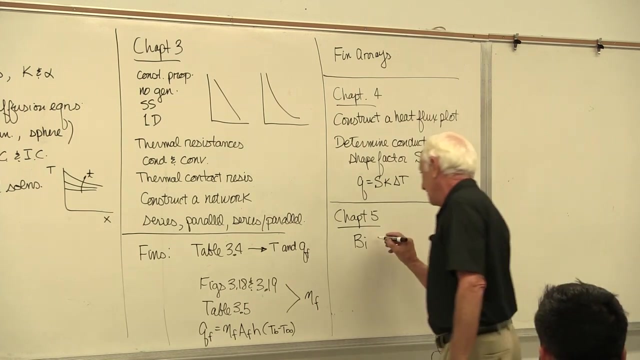 So don't worry about that part. for the final, Nothing on the numerical methods, part Okay. Chapter five, Transient chapter. We know what the first step is: The B-O number. If the B-O number is less than one-tenth, use lump. 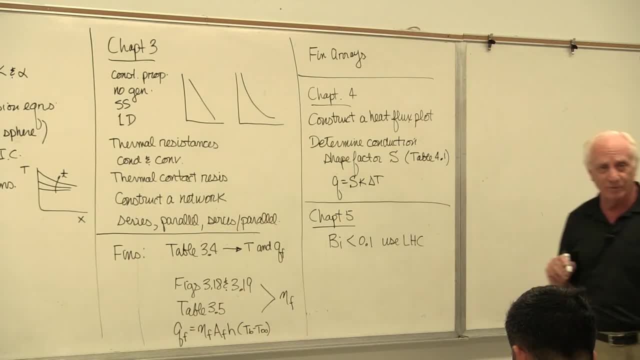 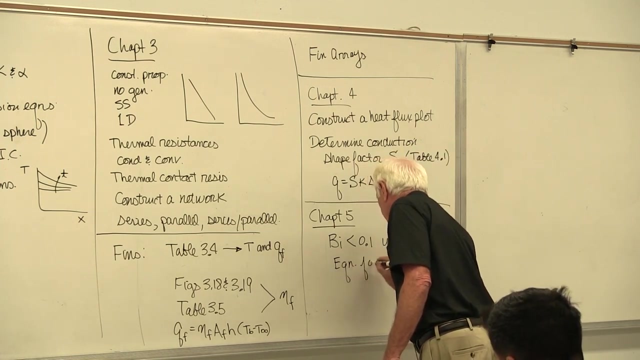 heat capacity. Don't make life difficult and use the equations. The more lengthy equations take this easy way out. B-O: less than one-tenth use lump heat capacity. There's an equation for that, For T, and an equation for Q. So two important equations. Check the B-O. 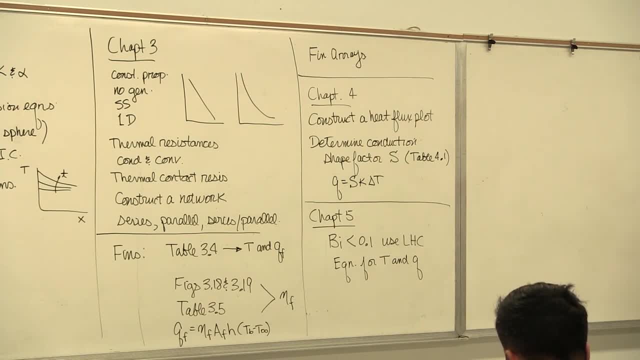 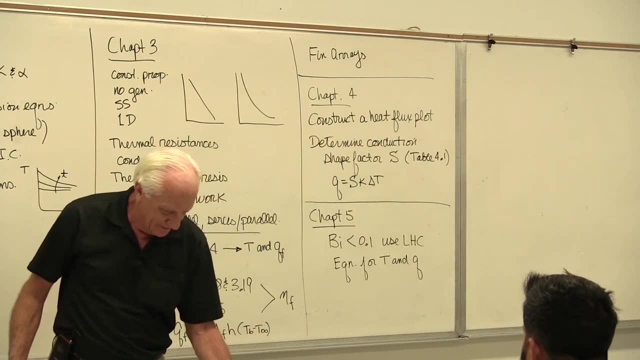 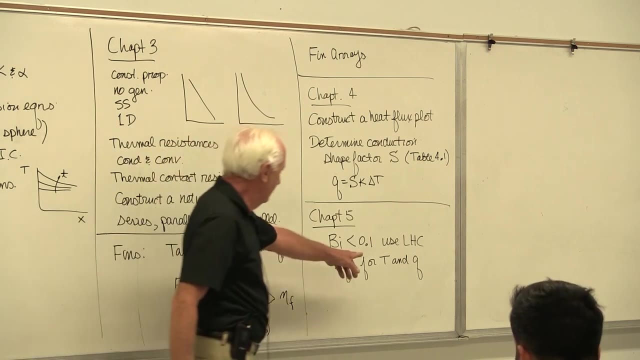 number Less than one-tenth. You want to find temperature? Use one equation. You want to find Q, Use the other equation. Equation: five, six, five, eight B. Five, six, five, eight B. Of course now. 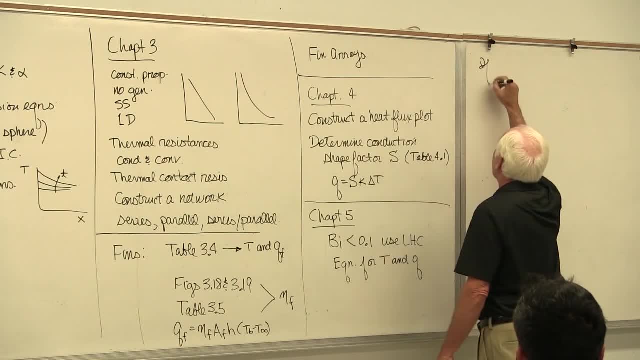 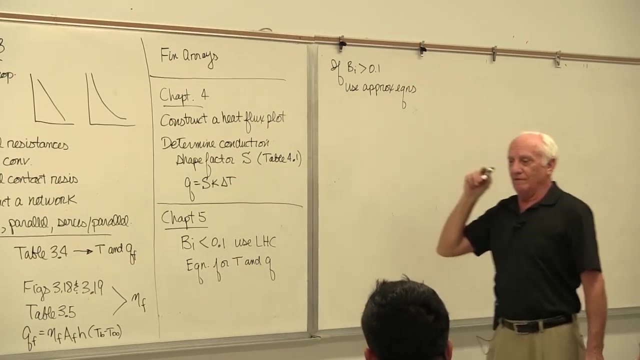 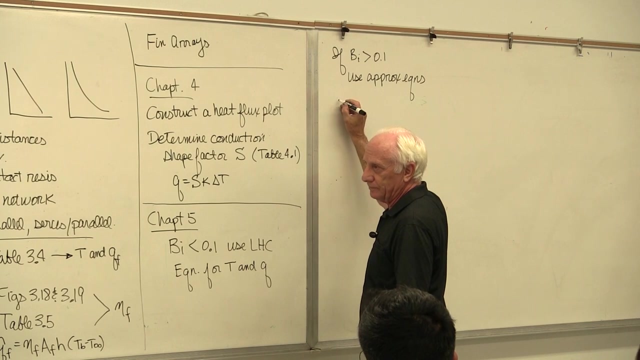 if the B-O is greater than one-tenth, use approximate equations. Now, there were a total of nine approximate equations, So here they are. One set of equations was for playing walls, Another one was for a long cylinder And the third, of course, was for a sphere. The three most 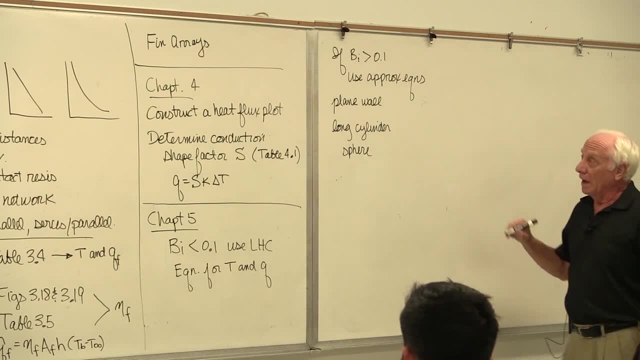 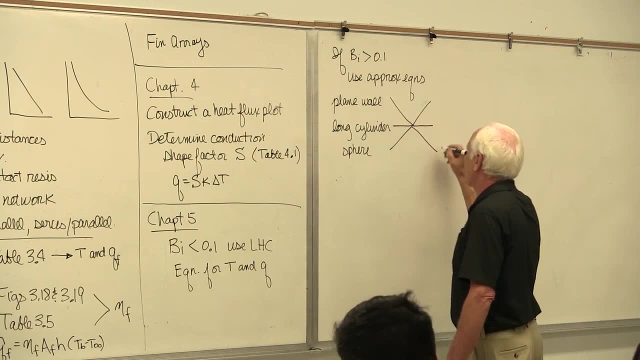 popular geometries. For each of those you can get three things. If you want the temperature at any value of X or the radius, there's a temperature. there's an equation for the temperature at any X value in the wall or any radius. 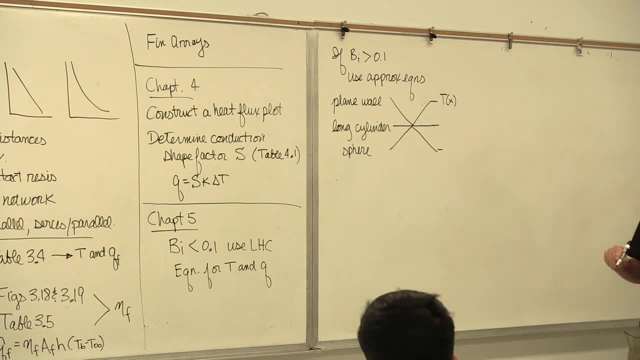 in the cylinder or sphere. There's also an equation for the temperature at the center of the wall or the center of the cylinder or the center of the sphere. There's also an equation for Q. It's capital Q in this chapter because it's in joules. 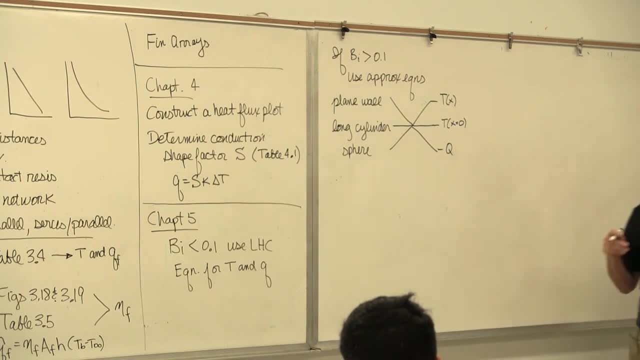 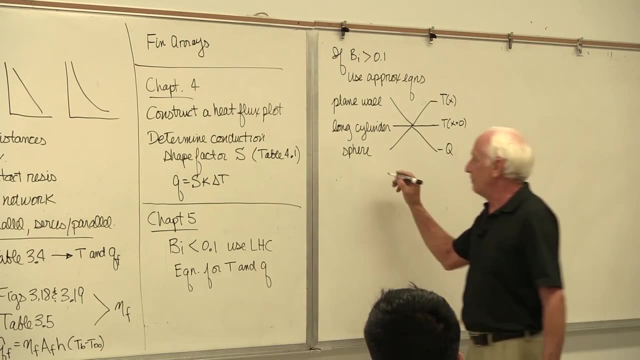 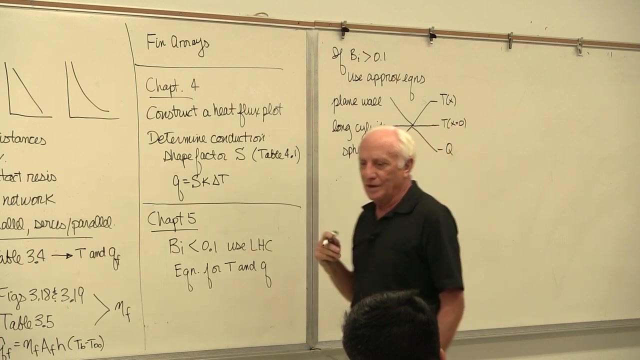 And that equation gives you the amount of energy transferred to or from that object in a certain time span. A total of nine equations. When you're done using those approximate equations, check the Fourier number. It should be greater than 0.2.. 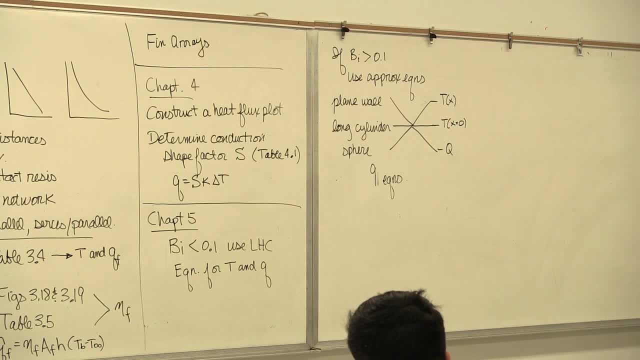 You check the Fourier number when you're done, It should be greater than 0.2.. And that ends that chapter. Okay, I'm going to put chapter 12 over here because I'll need some space for this. Okay, chapter 12.. 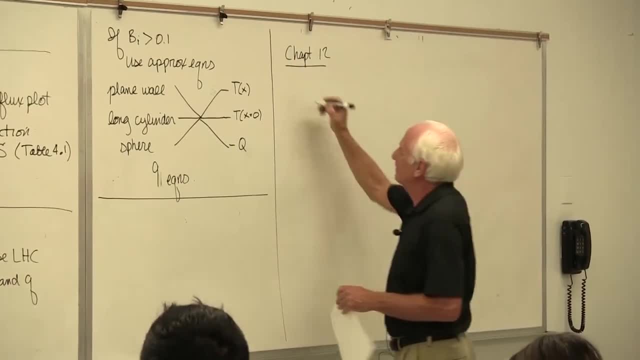 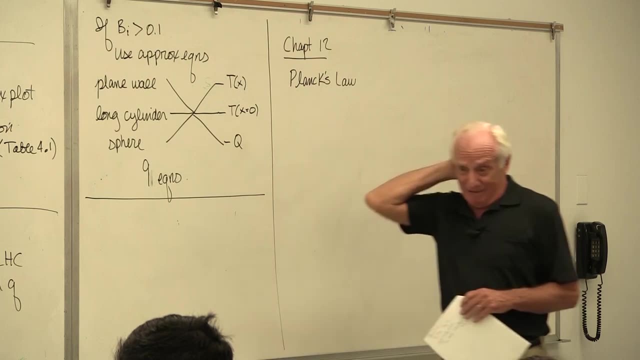 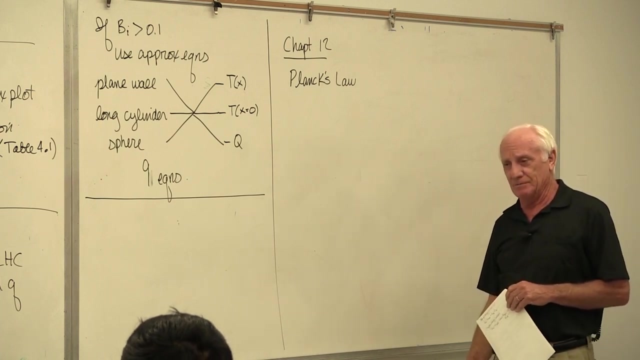 Alright, we'll start at the beginning. The first one: Planck's Law. It gave me a graph. It's an equation and also a graph of the spectral black body emissive power. E b, subscript, lambda, E b, lambda versus lambda. 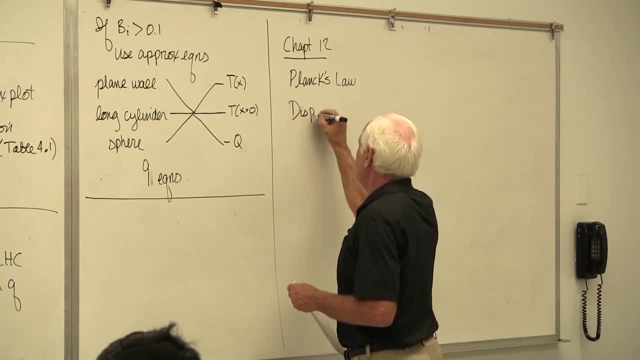 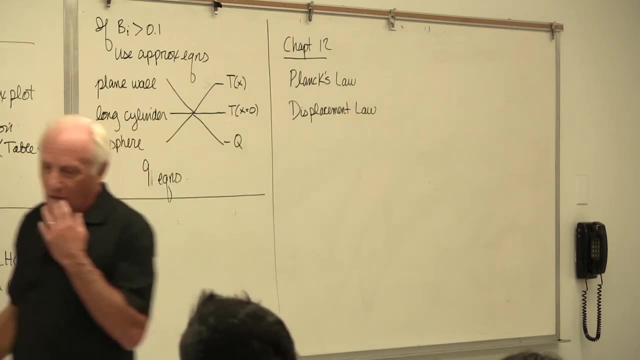 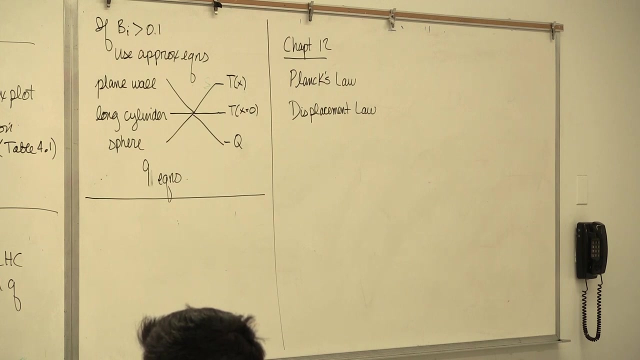 Displacement law And displacement law. Let's see chapter 12 here Real quick. Yeah, there it is Okay. I'm trying to see what that constant is. Lambda max t is 2898.. Lambda max t is 2898,. 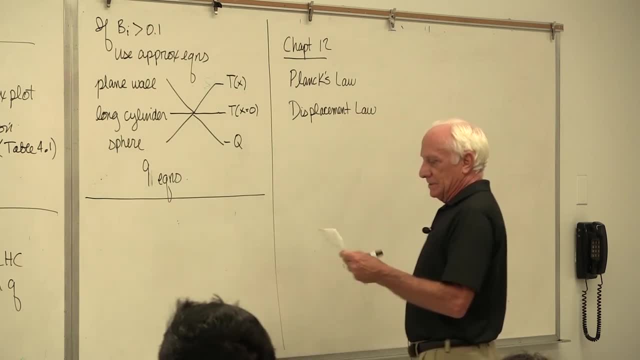 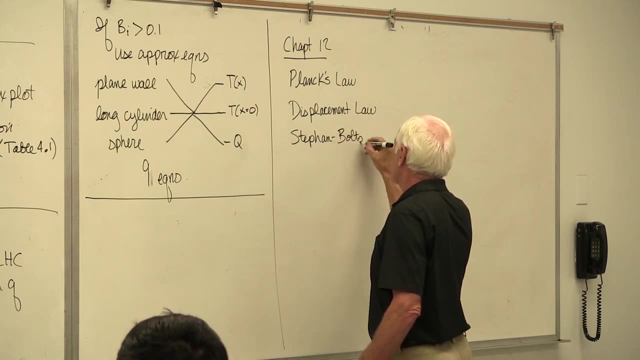 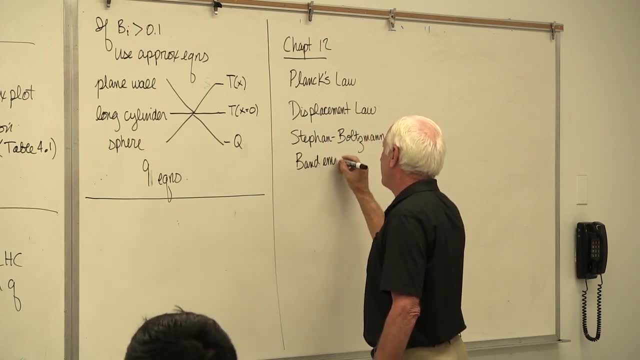 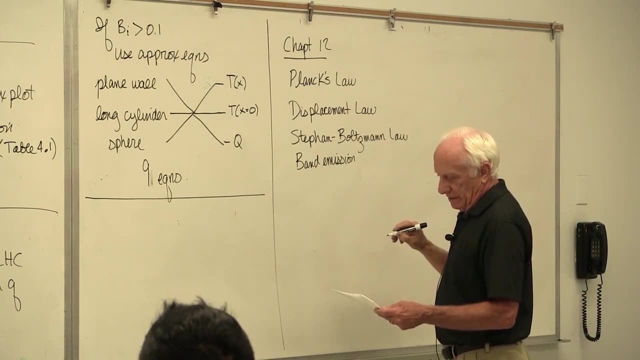 Band emission problems. Band emission problems: How much energy is emitted between certain wavelengths. That's called band emission. To do the band emission you've got to use the table for effort values, Table 12-2.. Table 12-2.. 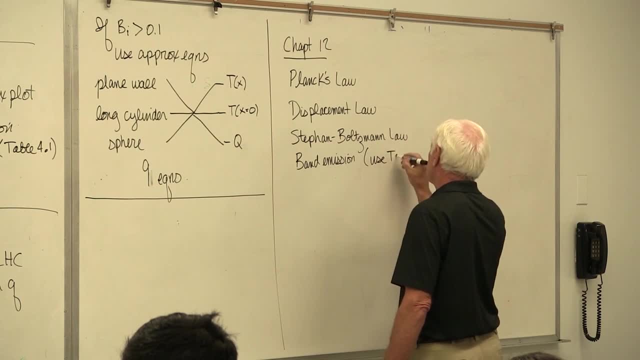 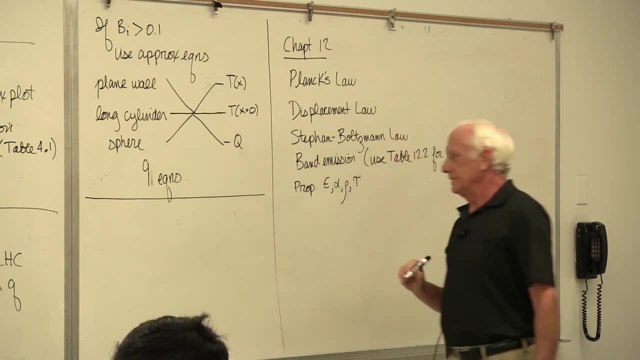 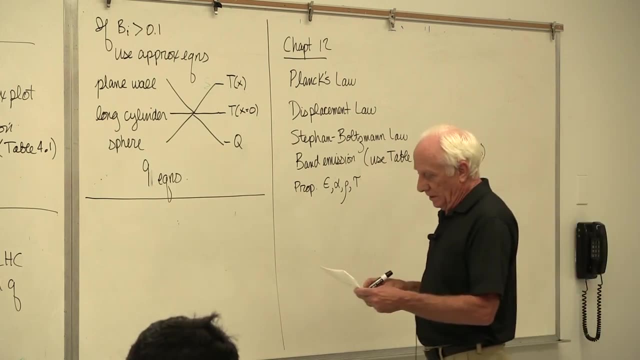 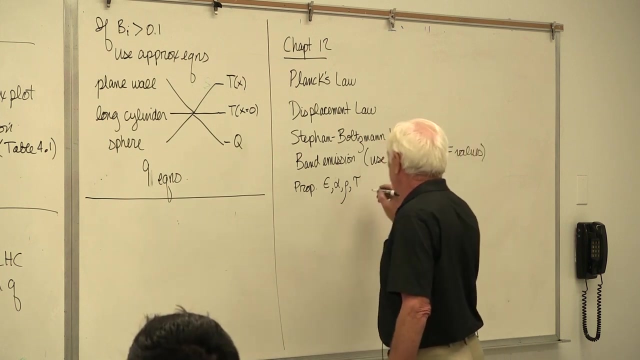 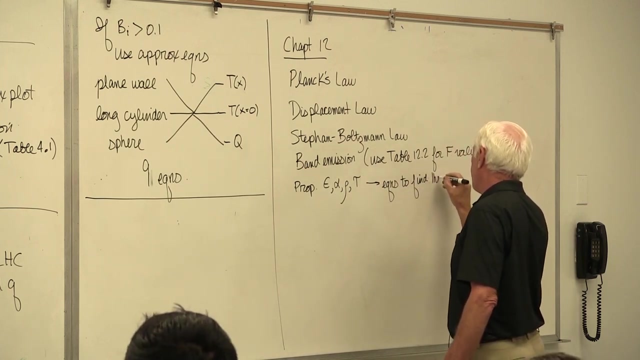 Alpha, Rho, T, Tau, Emissivity, Absorptivity, Reflectivity, Transmissivity, Dimensions, Equations to find these. Equations. to find these. Okay, Four equations in your notes, Equations to find those. 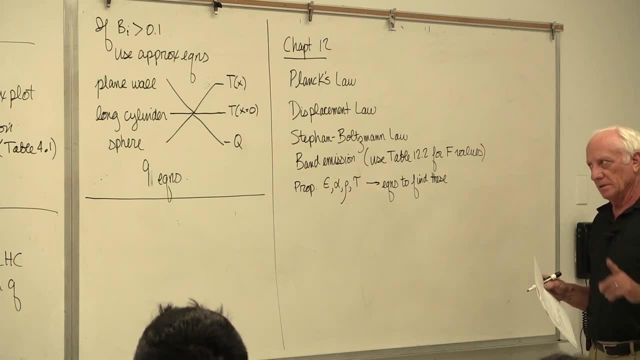 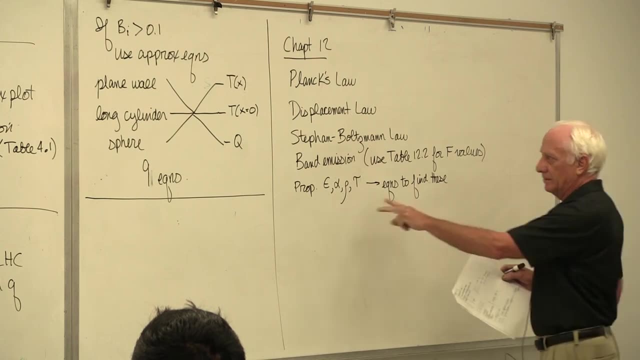 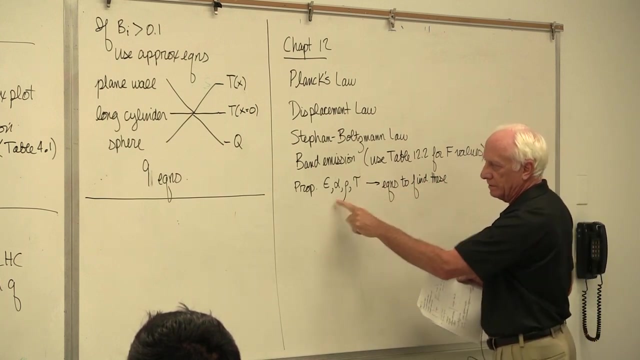 You can be given a graph of G versus lambda, Or you can be given a temperature of the surface. Two ways to combine the graphs of these guys with a graph of G, lambda versus lambda, Or a temperature, Or if the radiation comes from the sun. 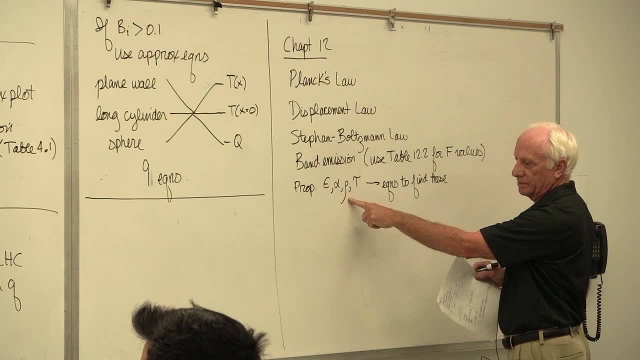 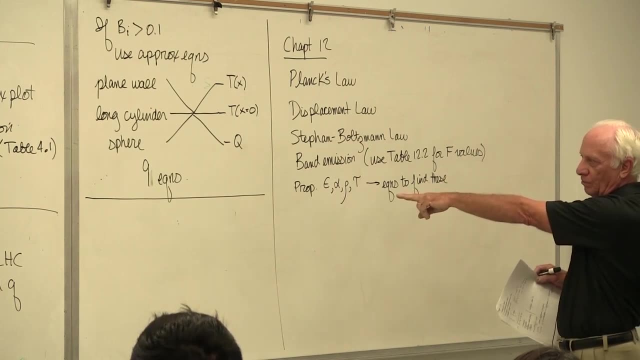 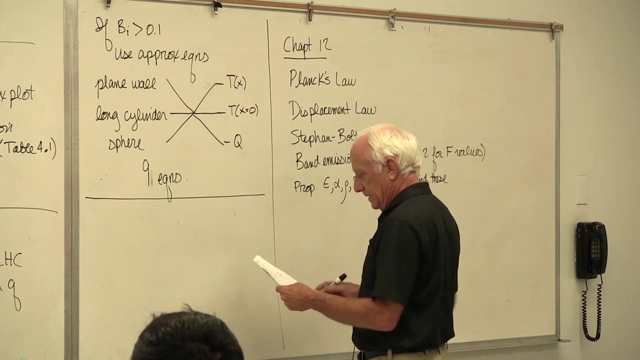 then it would be the temperature of the sun, Equivalent temperature of the sun Fifteen hundred. We worked three of those problems in class. You worked three for homework, Four for homework. We can use energy balance on a surface, Rho plus. 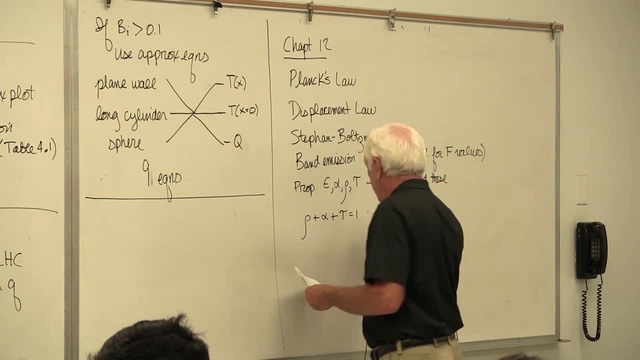 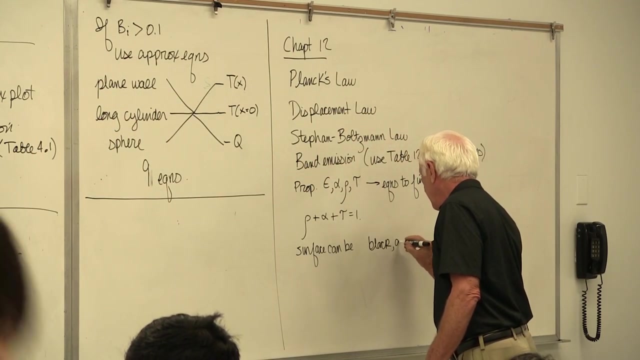 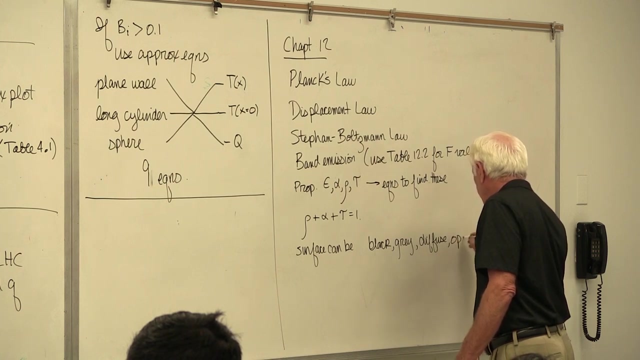 alpha plus tau equals one Energy balance on a surface. The surface can be diffused: Black, Gray, Diffuse, Opaque. There's a lot of language in chapter twelve, The language of radiated heat transfer. What do these words mean? 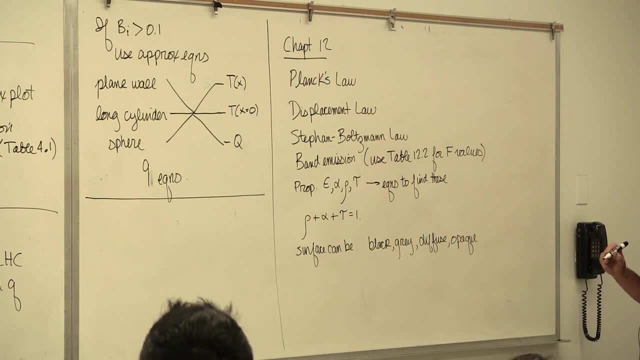 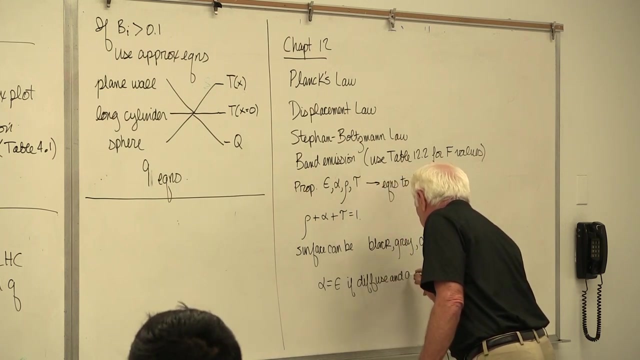 Opaque Tau equals zero Black Epsilon equals one Black Alpha equals one Alpha equals epsilon. If diffusing gray Alpha lambda equals epsilon lambda, If only diffused, It doesn't say gray, It just says a diffused surface. 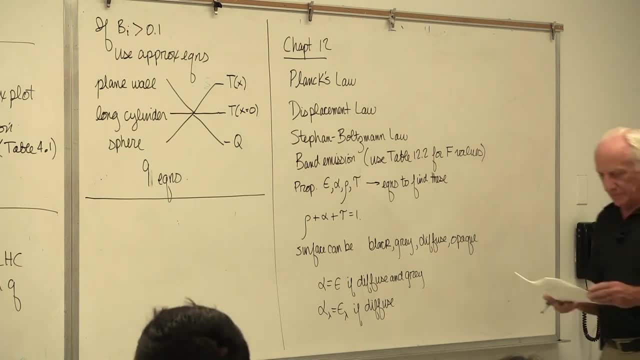 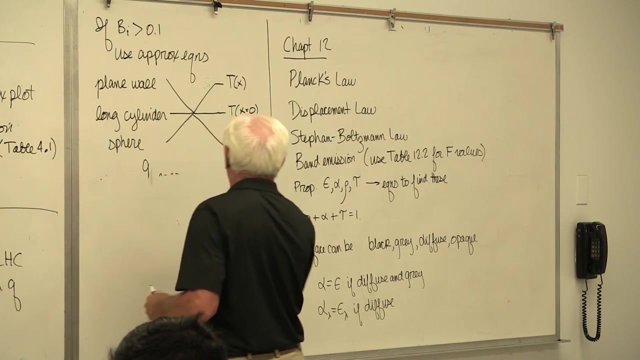 Those are called Kirchhoff's laws. Kirchhoff's laws. Okay, I'm going to put thirteen right next to twelve, I think, Okay. So Thirteen is again a very long chapter. It's the engineering applications of what you get in chapter twelve. 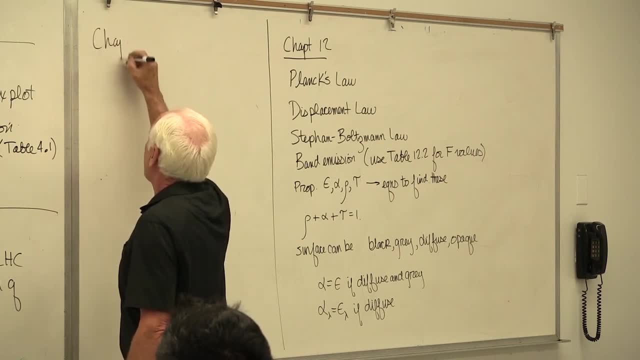 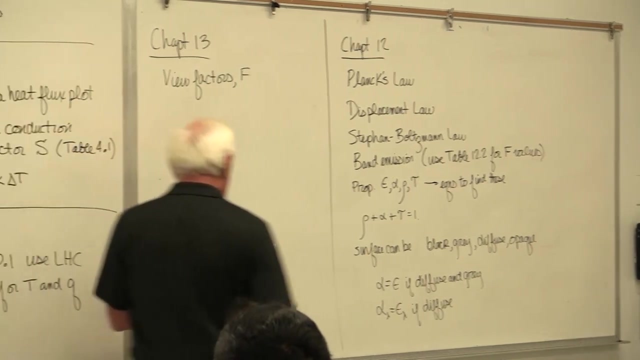 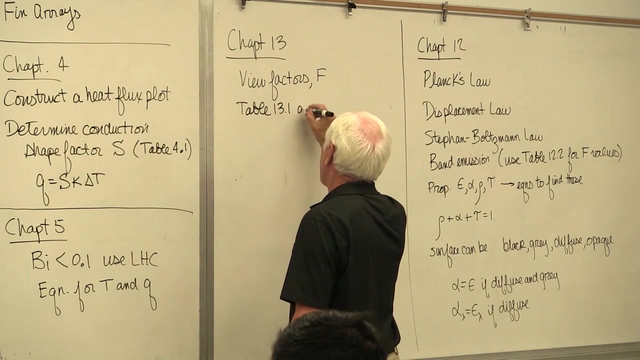 Chapter thirteen. We start off, of course, view factors. View factors. They need to. We could use table thirteen one and table thirteen two, Or we could also use figures Thirteen four, Thirteen five And thirteen six. They all give F values. 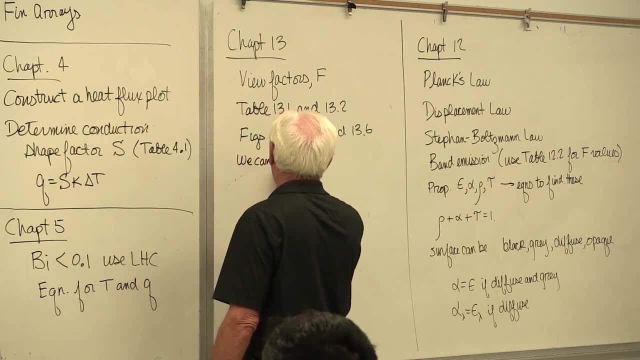 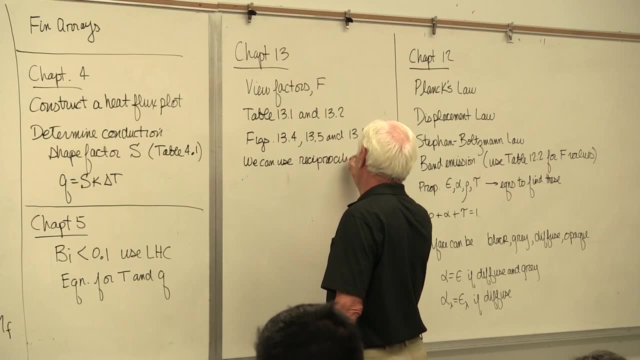 We could use table fifteen, Table fifteen, We could just go for a little bit. Table fifteen, Table 15.. Table 17.. Table 17.. Table 17.. Table 18.. Table 19.. Table 21.. Table 22.. 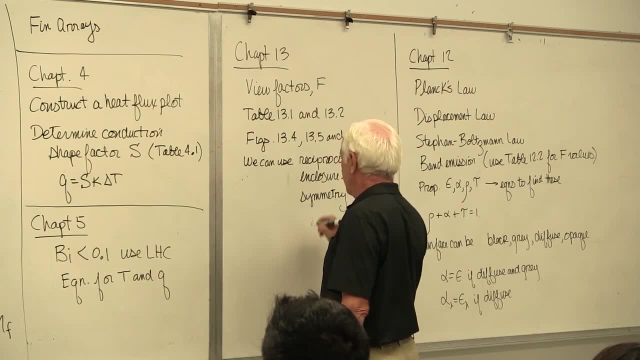 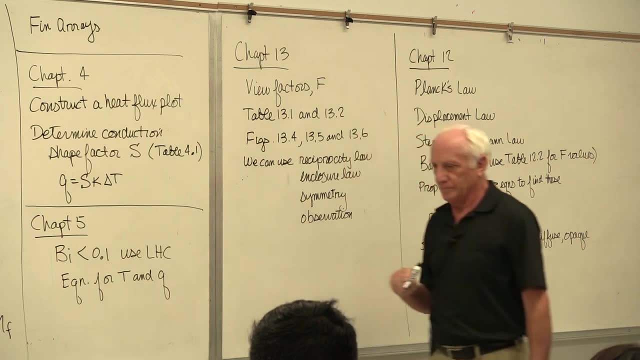 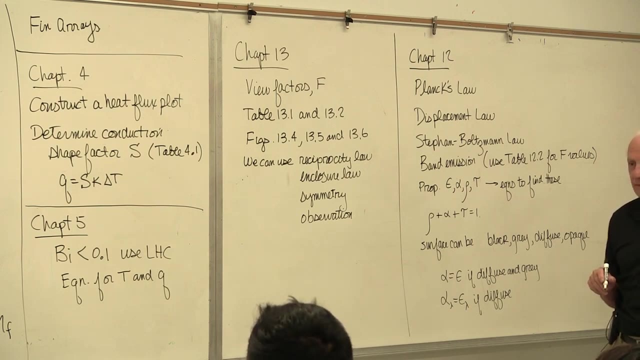 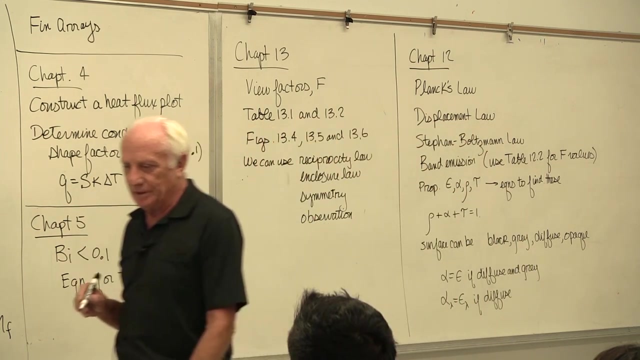 Table 23.. Table 24.. observation: immortal: inside a sphere, f1, 2 is 1, why reciprocity law: a 1, f1, 2 equal a, 2, f, 2, 1. enclosure law: f1: 1 plus f1, 2 plus f1, 3. 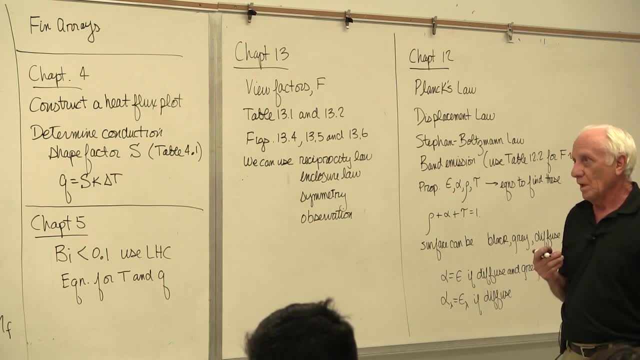 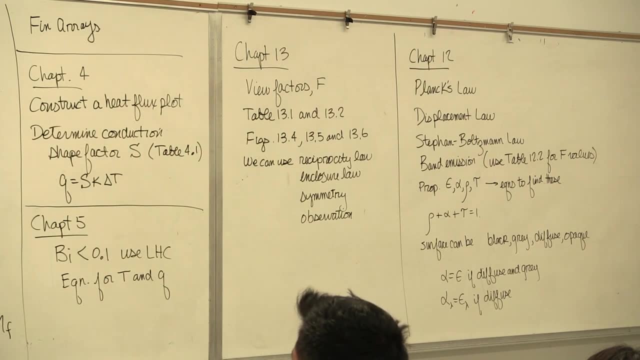 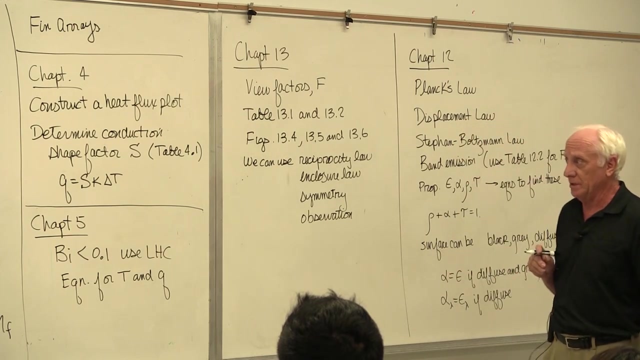 equal 1. if the surface is plain, f1: 1 is 0. if the surface is convex, f1: 1 is 0. if the surface is concave, f1: 1 is not 0. so is the surface plane convex or concave, to know? big hints, major hints. we use all the stuff here to get all these new. 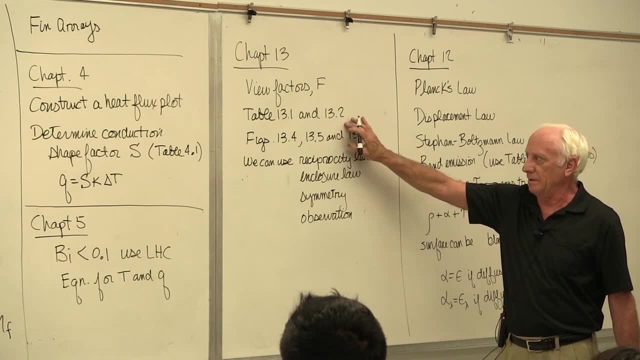 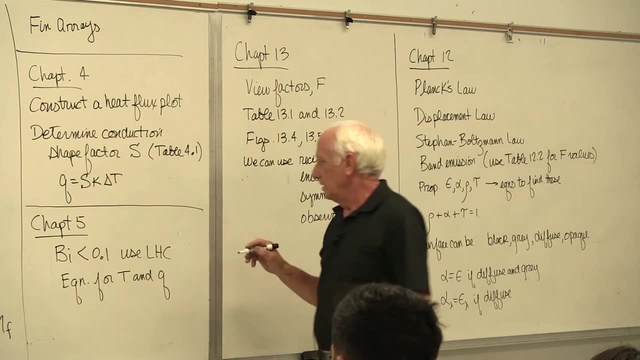 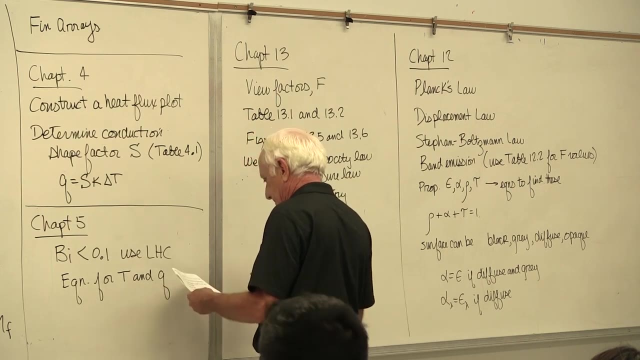 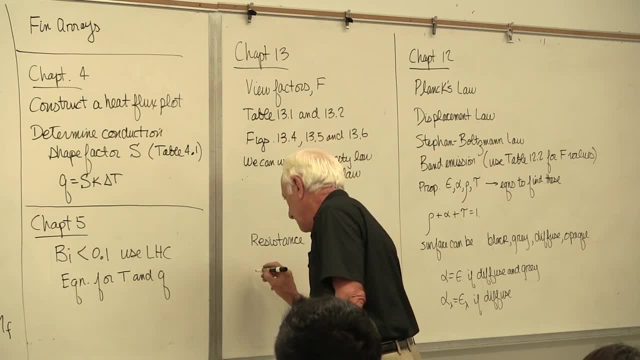 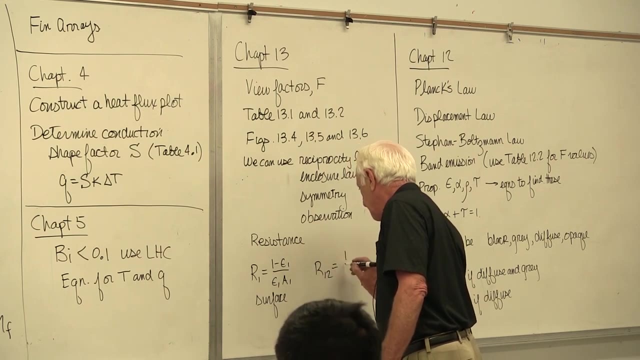 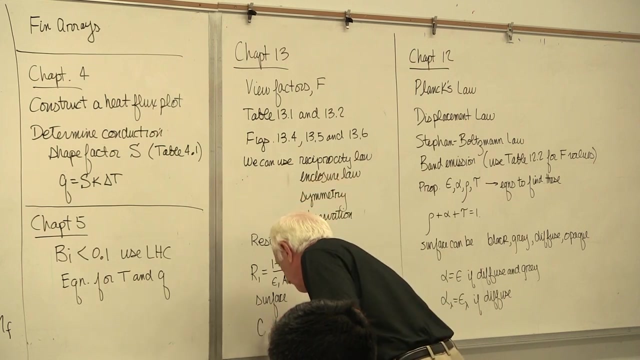 start out with. every surface in an enclosure has a surface resistance. So R1 equal 1 minus epsilon 1 over epsilon 1, A1.. Surface resistance- A space resistance. Every pair of surfaces in an enclosure has a space resistance A1,, F1, 2.. Space Construct the circuit. 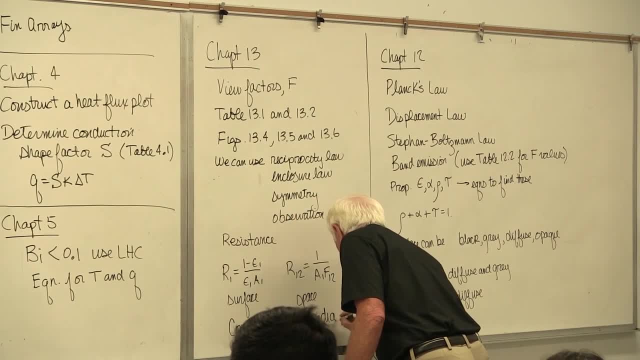 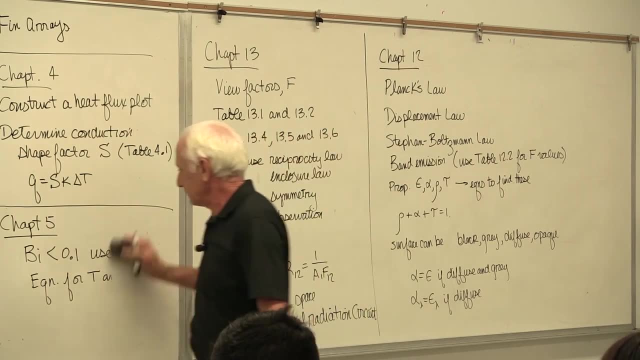 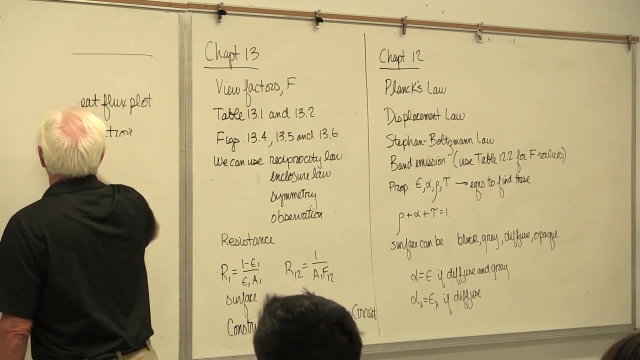 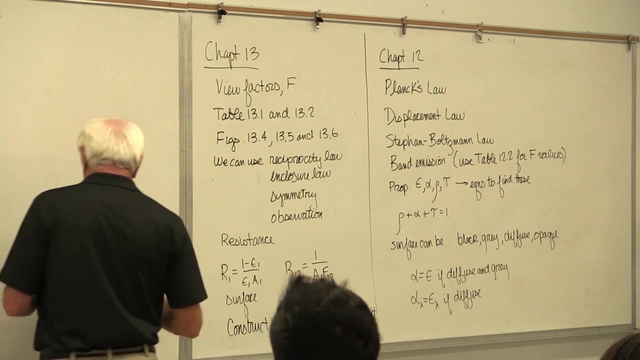 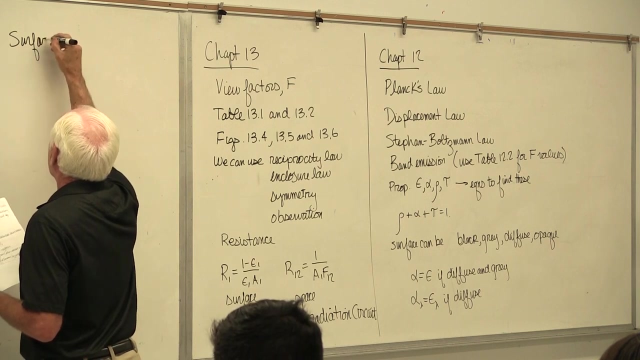 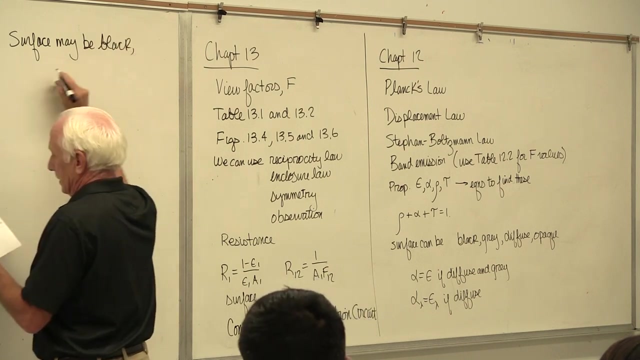 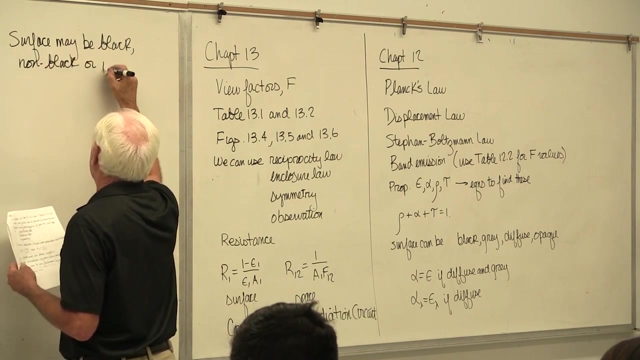 Okay, And again, it may be series. It may be series parallel, Just like we had in conduction, but now it's radiation Surface. Surface may be black, Of course, it may be non-black, It may be re-radiated, which? 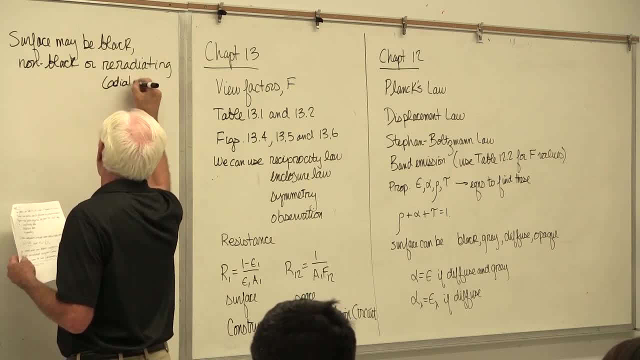 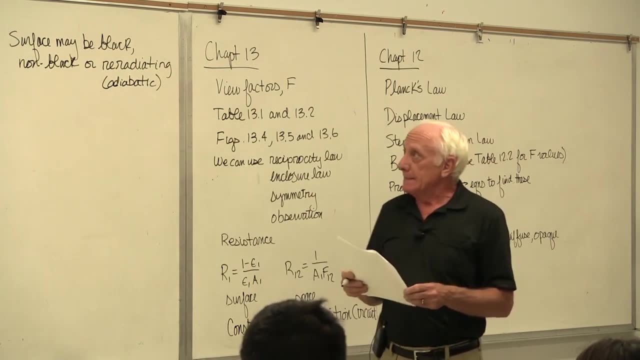 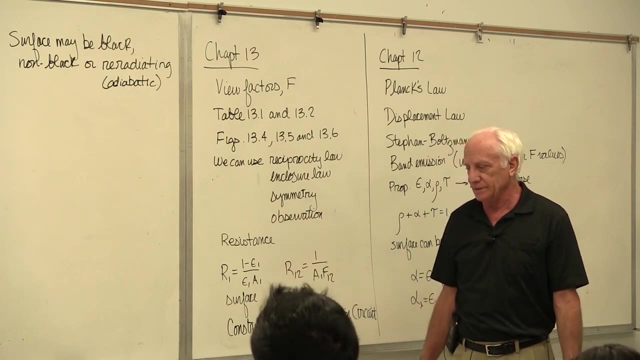 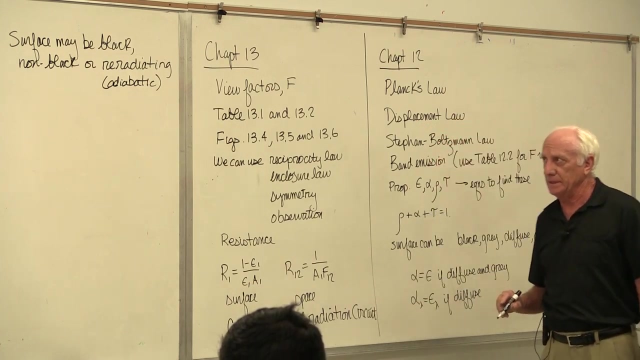 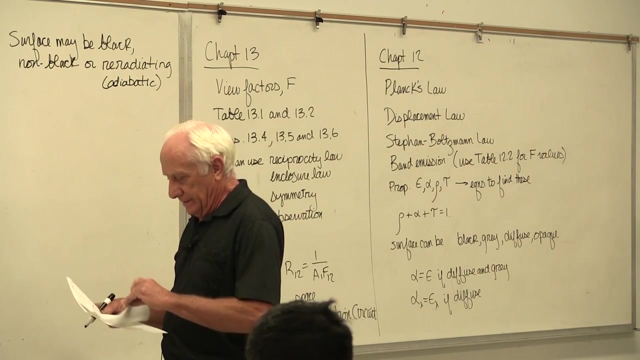 means adiabatic, Perfectly insulated. If it's black, R1 is 0.. 1 minus 1 divided by A1, 0.. If it's re-radiating, Q is equal to 0 because it's perfectly insulated or adiabatic. And then know how to use hypothetical surfaces. 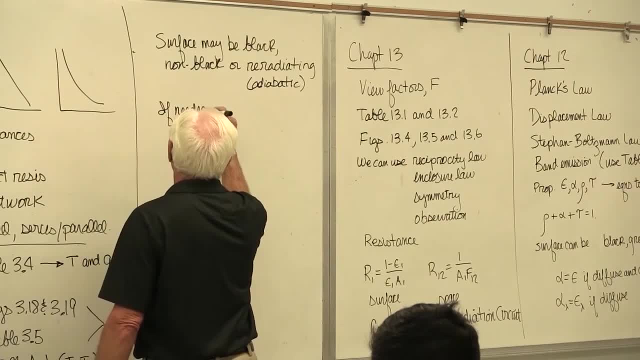 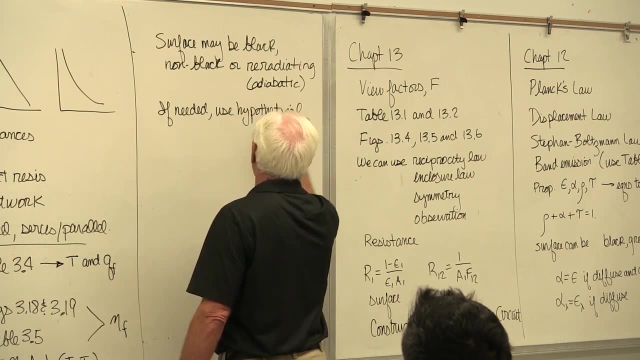 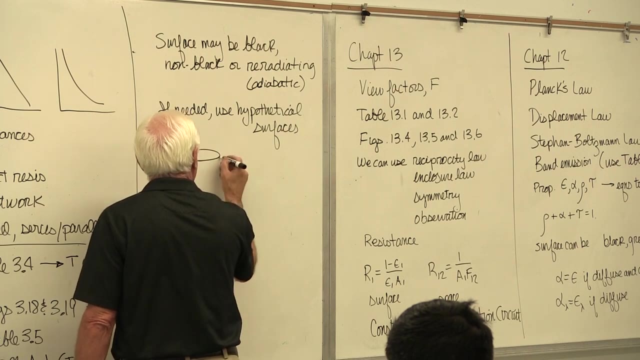 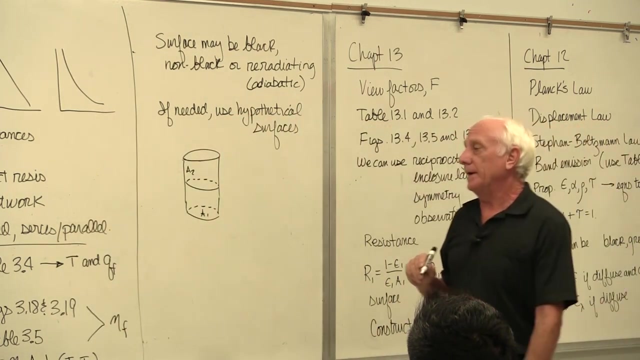 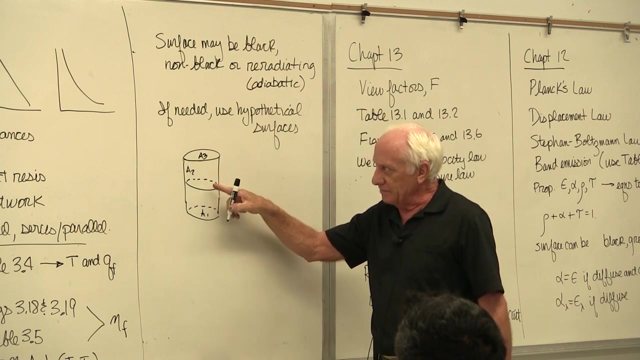 Okay, So surface A1.. Any example of that. I think we had maybe a fourth problem like this. This is surface A1.. The side wall here is A2.. Find F1, 2.. Okay, L rank. okay, I call this three. I'm gonna make a fictitious service right here. it's not. 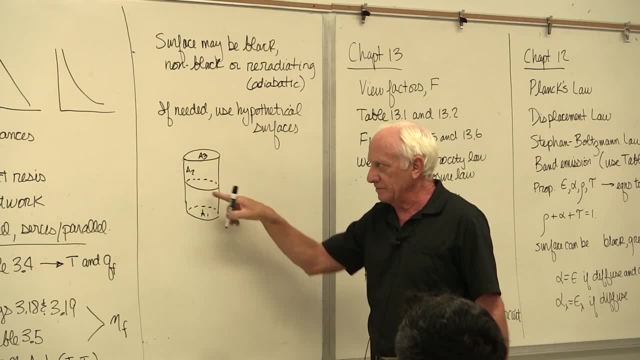 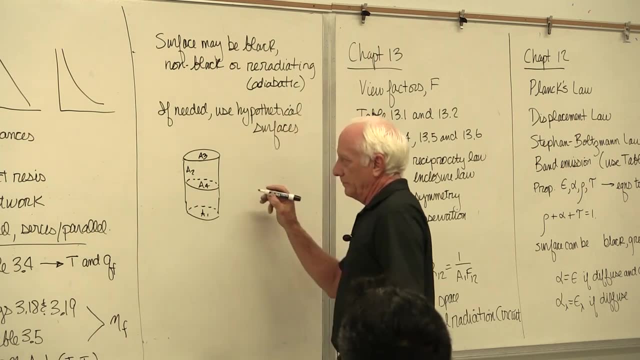 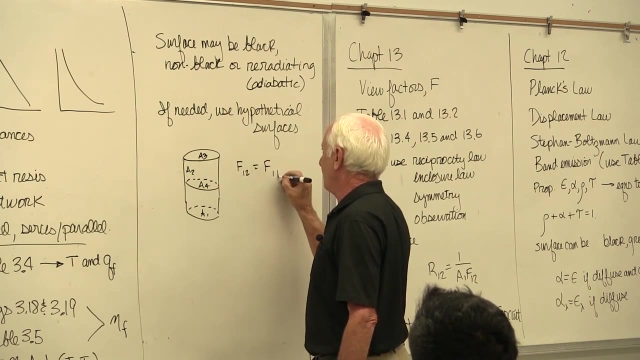 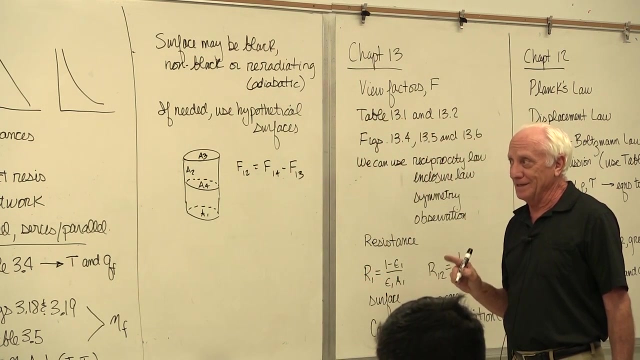 really there. this is empty inside, but I'll put a fictitious service right here and I'm gonna call that a four. so a one F wanted to equal F one to four minus F one, two, three. there it is. I can't solve that problem unless I put that. 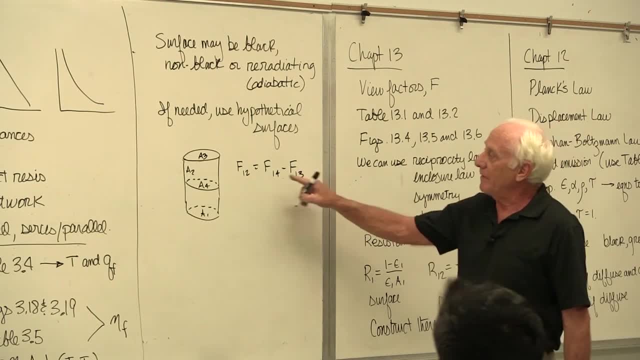 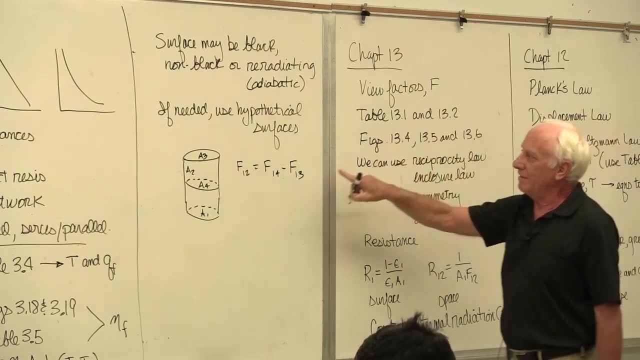 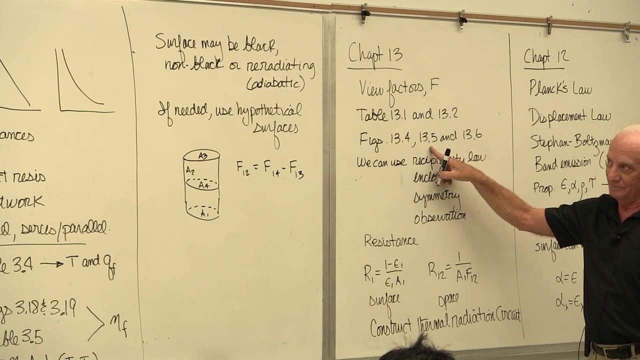 hypothetical surface a4 in there. where do I find F one four? oh, that's easy, right there. F one four. where do I find F one three? oh, that's easy, it's right there. got it done, deal. but I need to know how to use you have a proper. 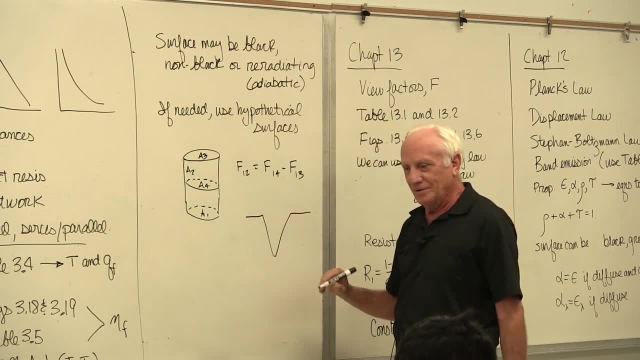 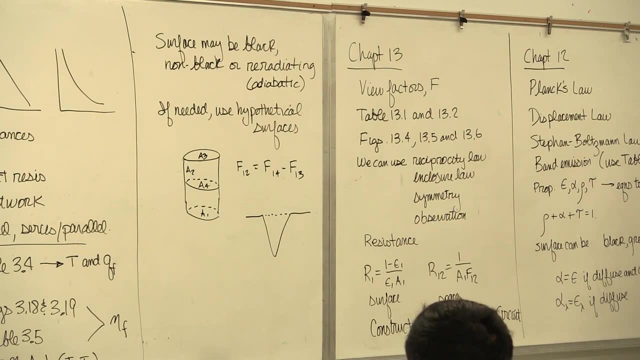 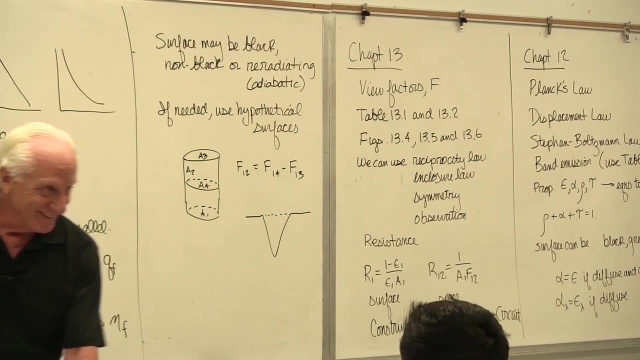 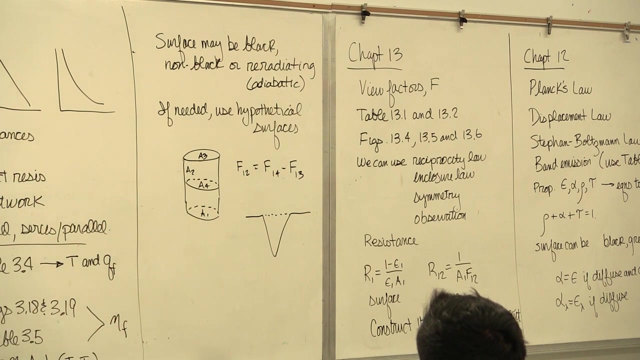 homework. a v-notch cut into a block. what did we do? we put a fictitious surface across there. we used it to get the view factors. if you need it, use it. okay. that wraps up a real, in a nutshell, eight week review. all right, I'll just go over again, in case you came in late last time, or? 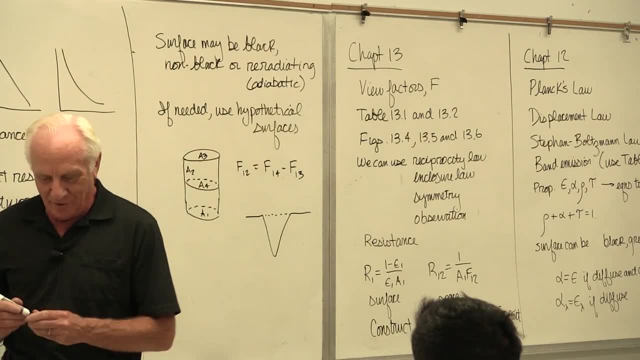 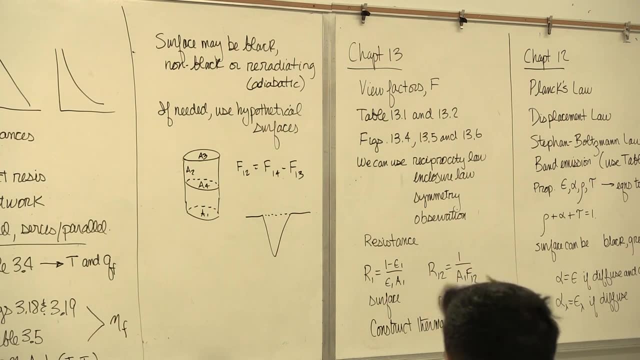 missed last time on the exam. we're looking at twenty point problems, five of them, four hundred points, five times the same length as your midterm problems, not double length or something like that. now they're the same. one problem, chapter eight, and internal flows. one problem, chapter seven. 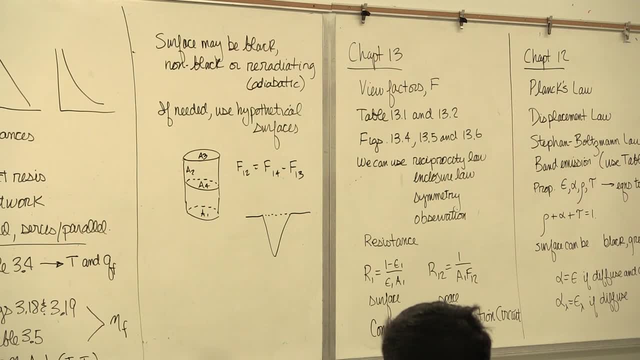 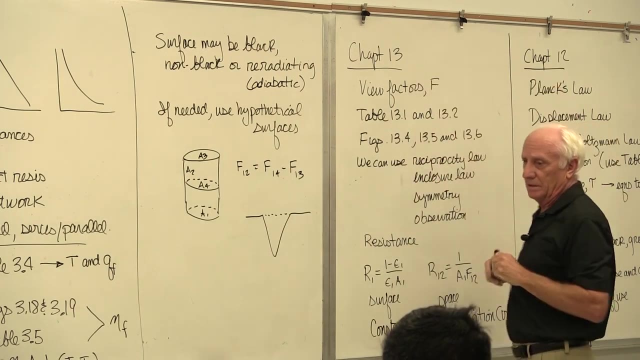 external flows. convection in chapter six is lumped into a boat. you've got chapter six is in parts of seven and eight, so of course six isn't into it, but specifically one on internal flow, one on external flows, one on radiation, chapter 12-13 combined, one on combo 12-13, one on 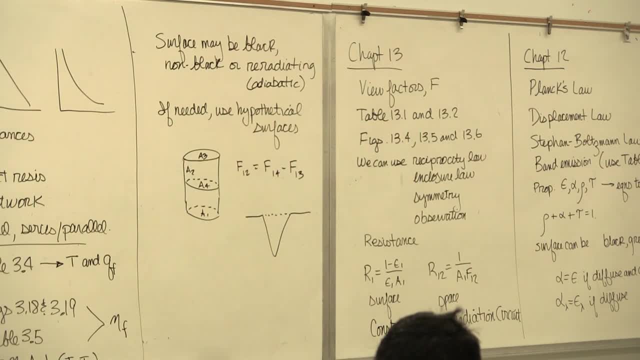 conduction, chapters 2,, 3,, 4,, 5, and one a chapter 1 type problem, a basic, low-level type problem with here they are, these guys right here. five equations right there, one like that. 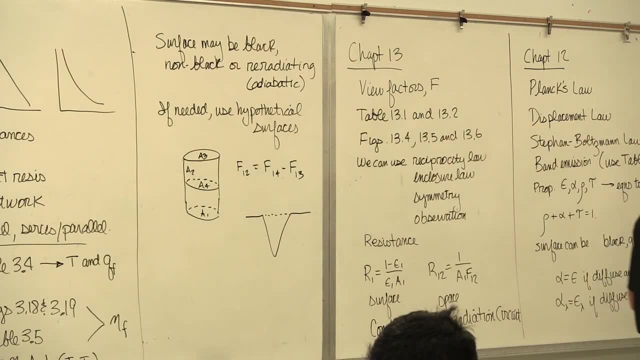 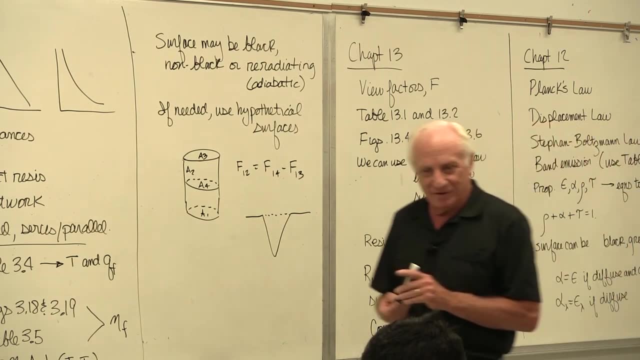 So you can bring in three sheets of paper equations on it, whatever you want to make. Example problems, homework problems, exam problems, I don't care. Both sides. ADAPT by 11, stapled together, stapled together. 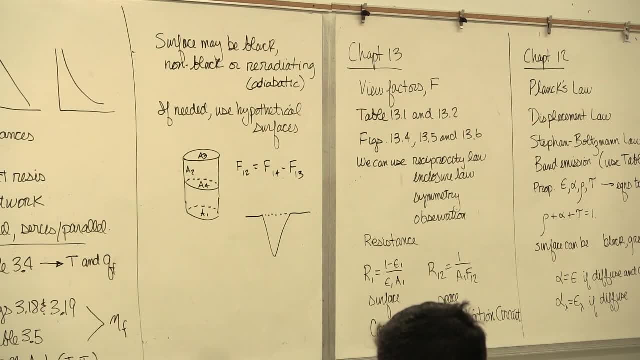 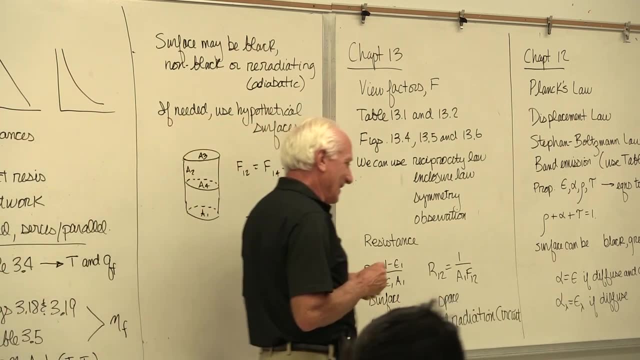 I'm going to give you the data package again, All right on Blackboard. next week's office hour. I'll just remind you: Monday 7-9,, Tuesday 9-11, and Wednesday 7-9, before our exam. 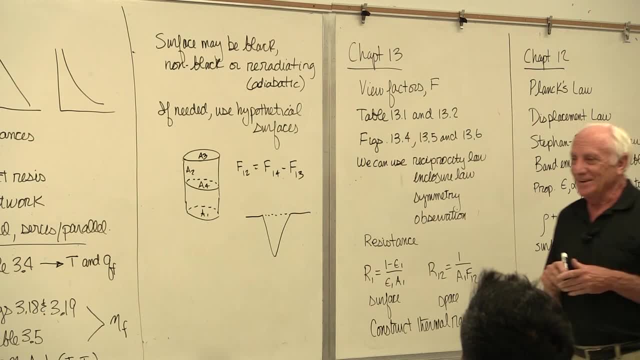 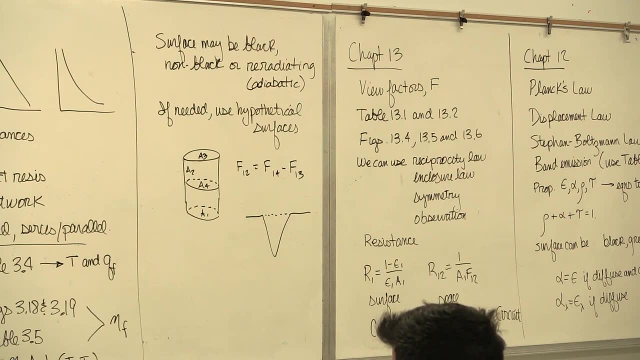 Wednesday at 9-10.. Okay, now a couple of other things this morning to do. Any questions on this or the exam? All right, I'm going to show you some interesting things from kind of everyday life. and that's what makes heat transfer such a fun course- is that there's so much stuff in the real world. 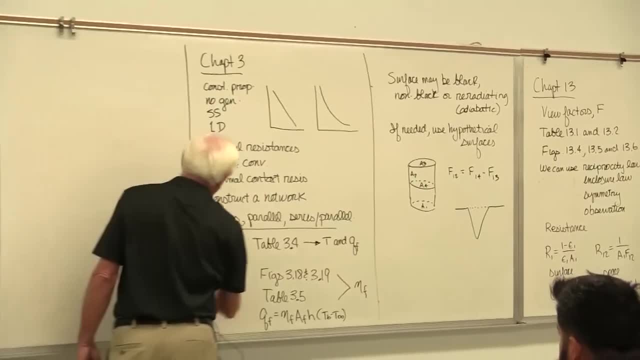 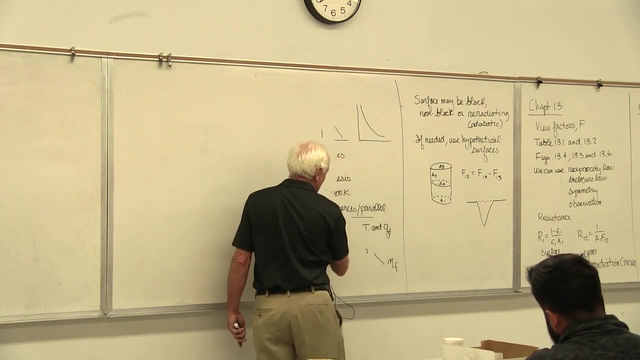 that we live in every day. That relates directly to heat transfer. It makes it mean more to us. I've talked about toasters in the past. you know how do you heat the toast: radiation. You want to heat the toast by convection. 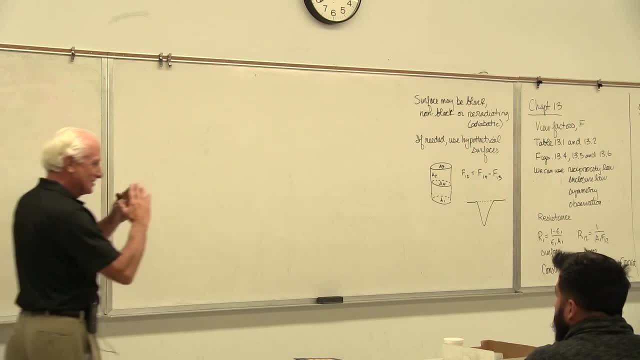 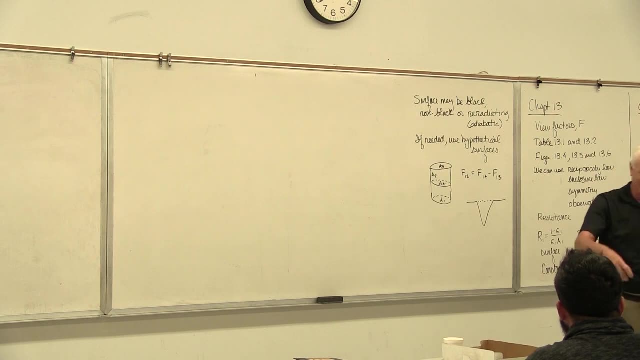 I hope not. You go camping. you can buy these things at the camping store. they're little metal frames like this and you can put the bread on a slice of bread each side of it, and you put it over the fire and the heat from the fire makes it go. 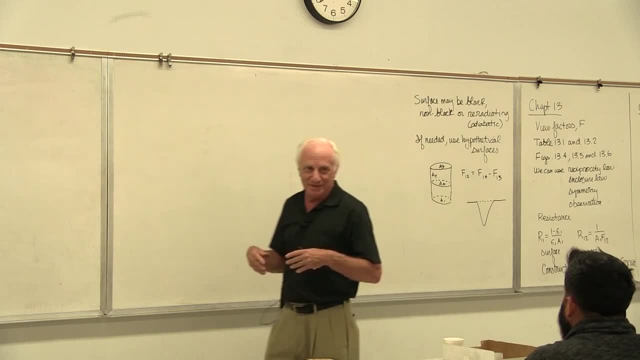 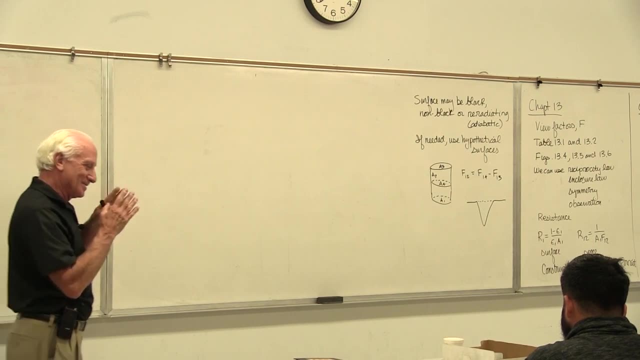 And you can heat the toast. What it ends up making is a very dry piece of bread. you take and break it in half. it's so dry. No, the purpose of toast is to make the outside crispy kind of, and the inside still soft. 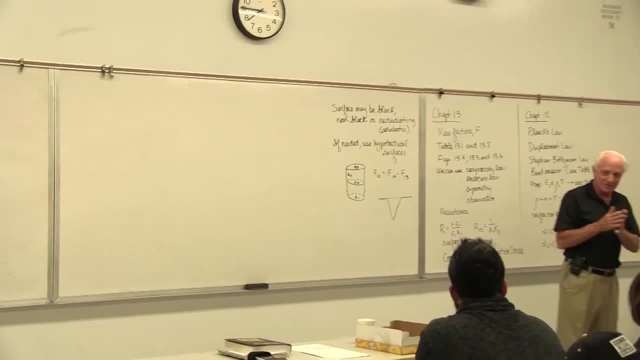 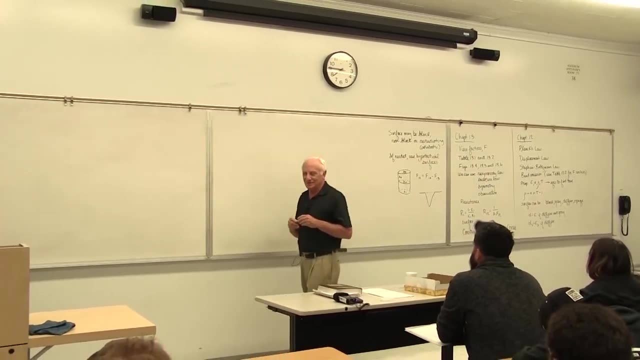 So radiation does that. it affects the surface of the toast. When the surface gets brown, take it out of the toaster. So a toaster works on radiation And you can go through the kitchen, you can go through the hot water heater in the garage. 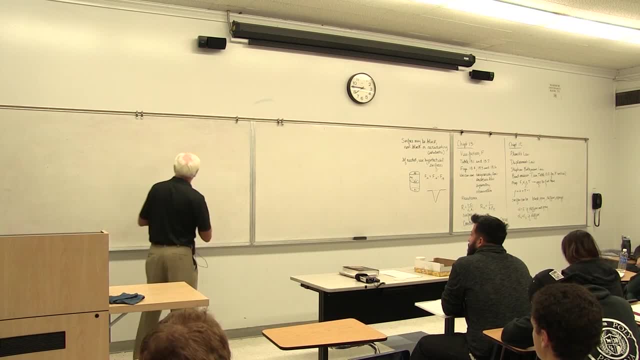 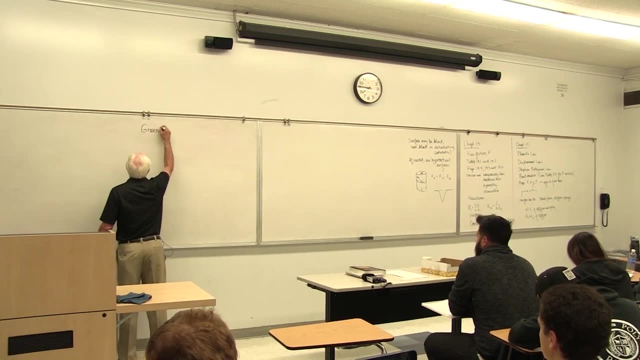 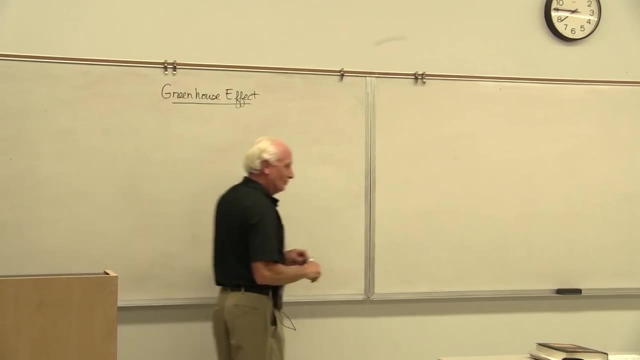 you can do all that kind of stuff. One thing you can do too as an example: let's call it the greenhouse effect. It's very popular now with CO2,, but when I'm talking about the earth, we'll get more lower. 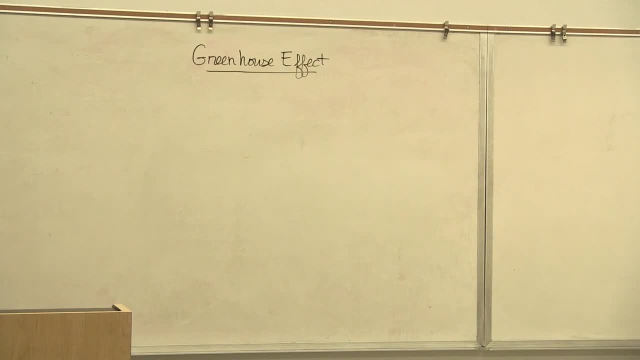 levels. We'll talk about your car. Of course, the name came from what? guess what? The greenhouse. Because what's a greenhouse supposed to do? Well, the purpose of the greenhouse, one of the purposes in a colder climate, or cool. 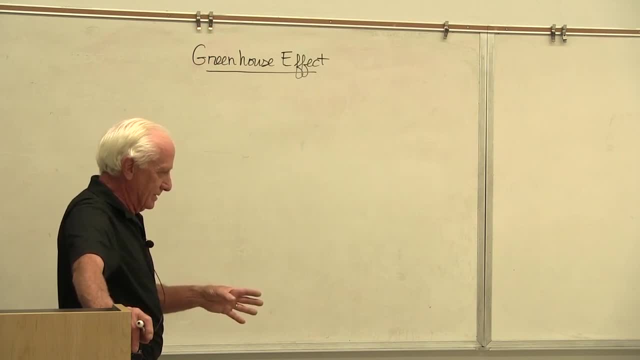 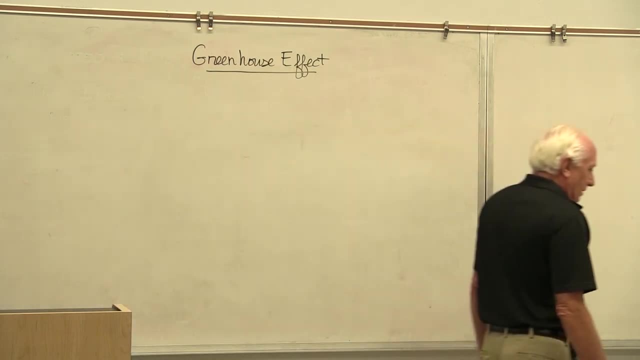 evenings. you've got growing things inside there, growing green things, and they're not going to expose those low outside temperatures which may kill them or ruin the fruit, And you want to make sure sun gets in there. That's the whole purpose. 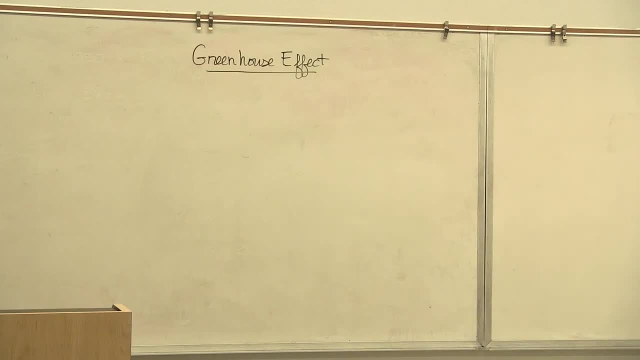 Green leaves, love sun. So, okay, you've got to let light come through. You can put glass or plastic, but let's just say glass in the greenhouse. You want the sun to come in. Okay, Now here is the windshield of your car. 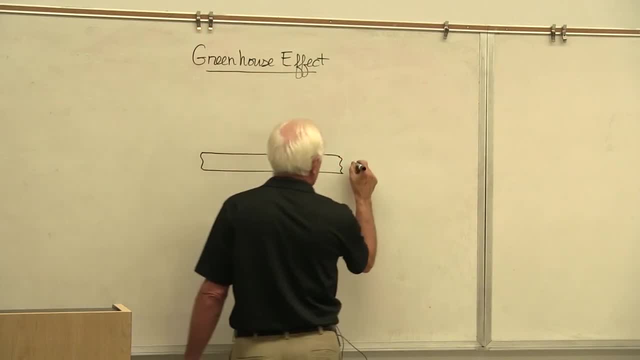 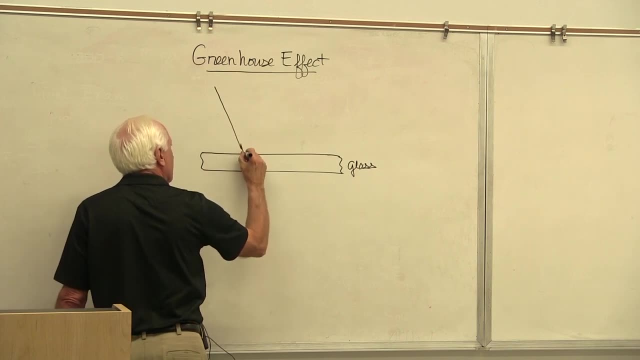 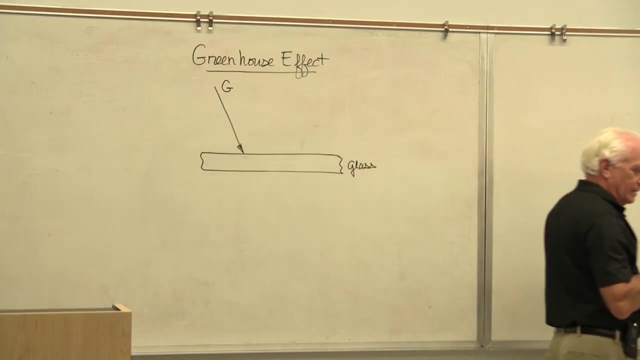 It's very similar to a greenhouse. This is glass. What happens is the irradiation, don't forget. irradiation is G, It stands for the incoming radiation is what comes in. What's J? J is the radiosity, It's what goes out. 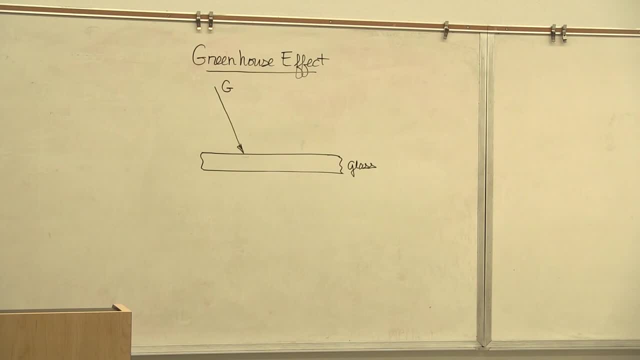 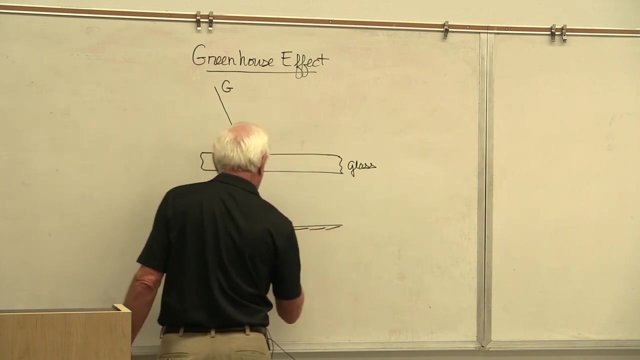 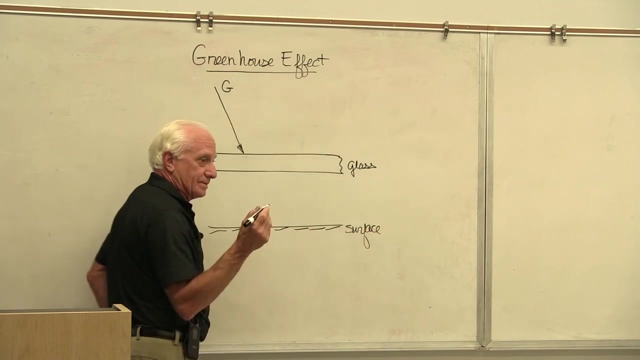 Okay, What's E stand for Emissive power? It's how much energy is being emitted as a function of the body's temperature. Okay, Radiation comes in. Here is the surface. It's glass. The sun's light comes in through the glass. 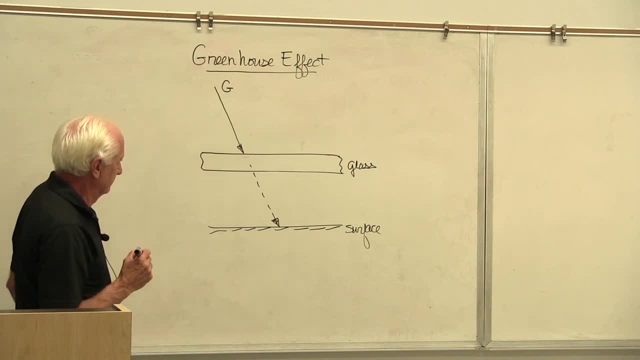 Strikes the surface, The surface gets hot. Let's say, you know, you've got your. oh yeah, I've got to have a black interior. Okay, That can be very bad. It depends on where you live. maybe I want a black interior. 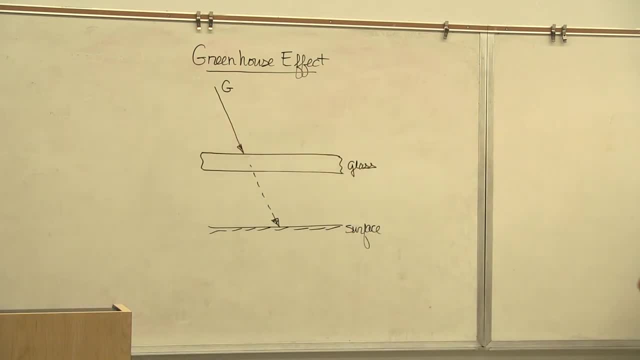 Okay, So this is a black upholstery, Or maybe it's a black dashboard. Take your choice. This stuff gets hot. Sometimes you can't touch the steering wheel, I guarantee it. It gets so hot. When it gets hot, it starts to emit heat. 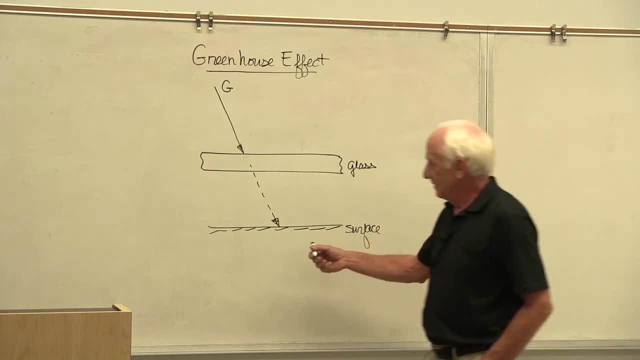 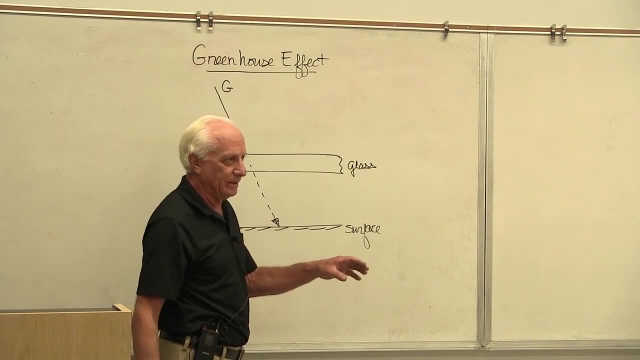 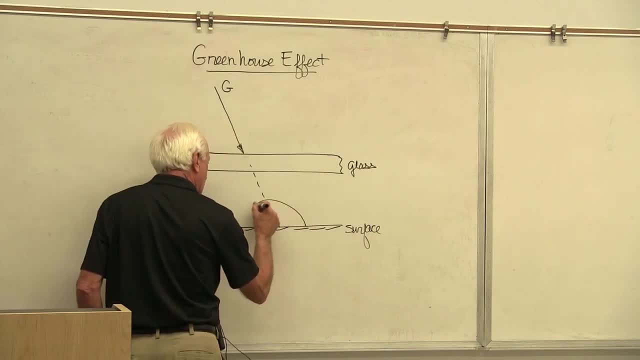 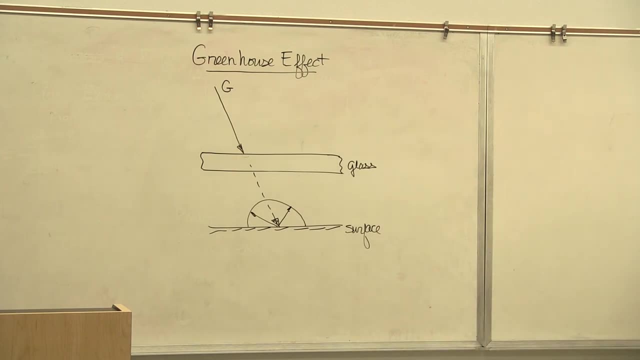 It gets hot. It gets hot. When it gets hot it starts to emit back out again because of its temperature. So we had a problem for homework in Chapter 12, which was a transmissivity of plain and tinted glass. 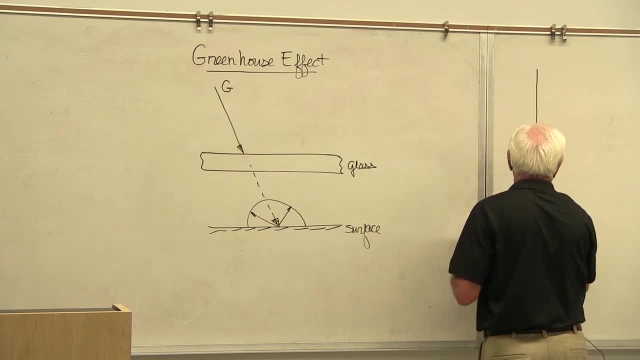 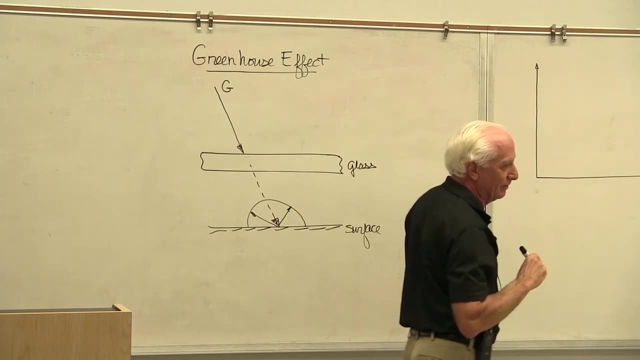 So I'll put that back up here again. Here's a transmissivity of plain window glass, and normally windshields are plain window glass. Well, the side of the back could be tinted, not the front windshield window glass. 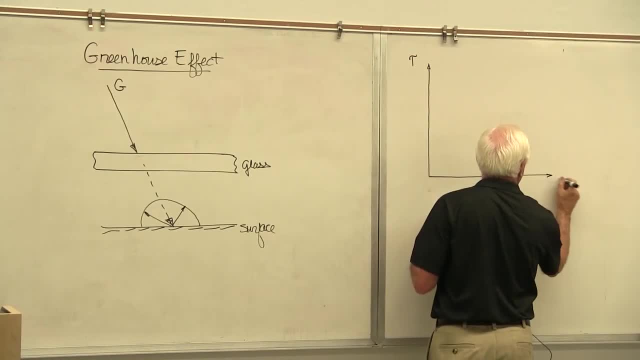 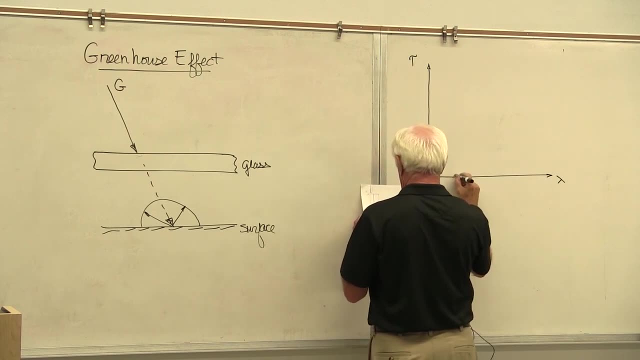 So this is transmissivity. This is a function of wavelength lambda in microns. The wavelength at 0.3,. this is out of the homework problem we have- it goes up to 2.5.. The transmissivity is really high for plain window glass in that range. 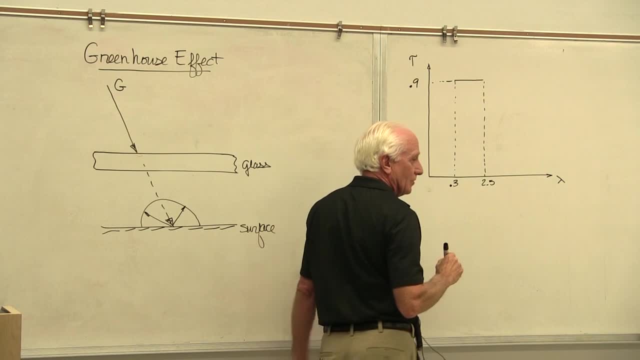 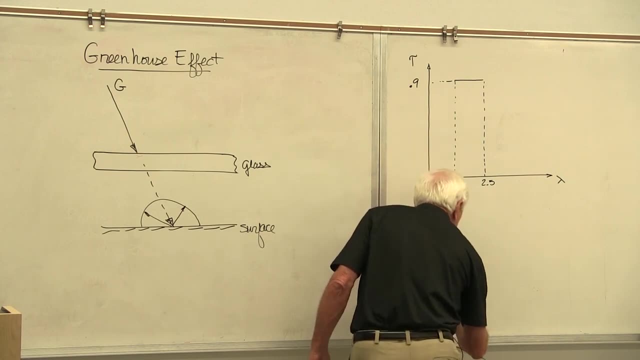 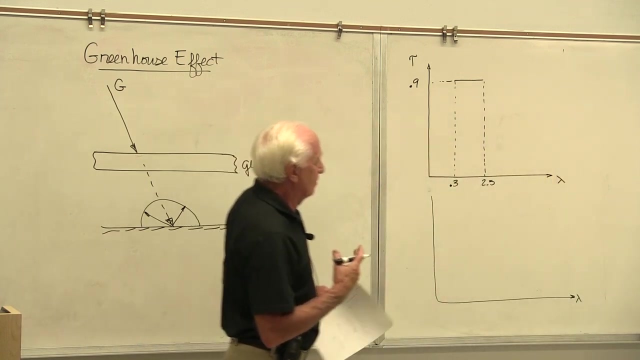 It's over 9 tenths. 9 tenths there, over 9 tenths. Now, what hits the glass? The incident radiation or the irradiation from the sun? How does that look? Well, it's proportional to a Planck's law curve. 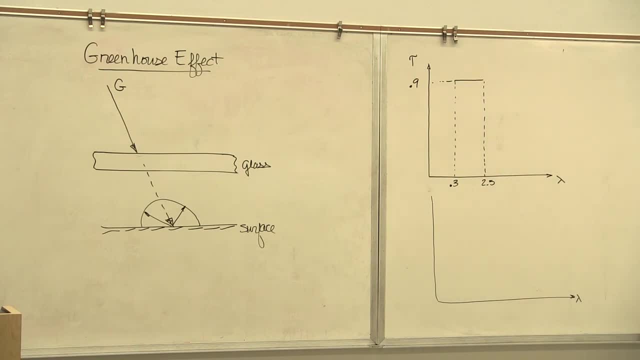 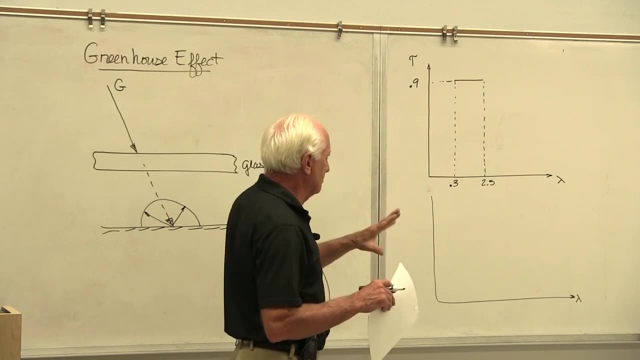 You know the sun radiating 5,800 Kelvin, but then it has to go through the atmosphere. so what hits the surface of the Earth? There's no less than that, But the wavelengths are similar, it's just their magnitude gets diminished. 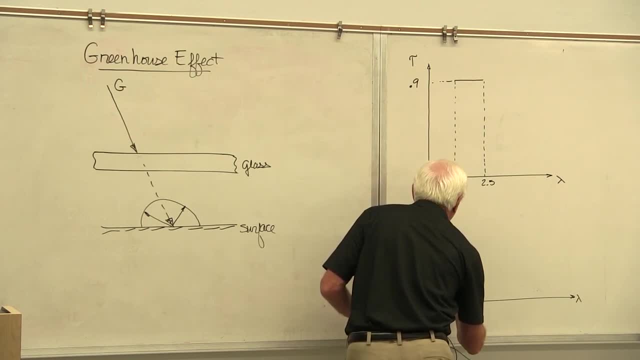 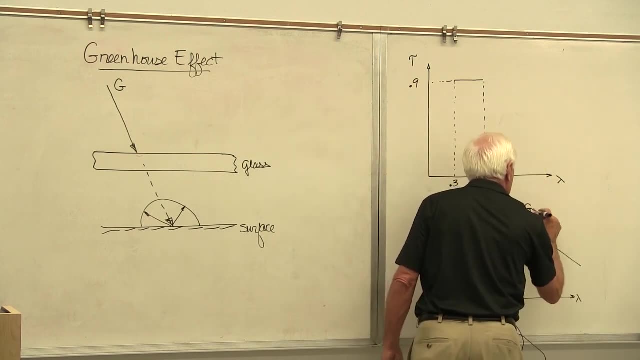 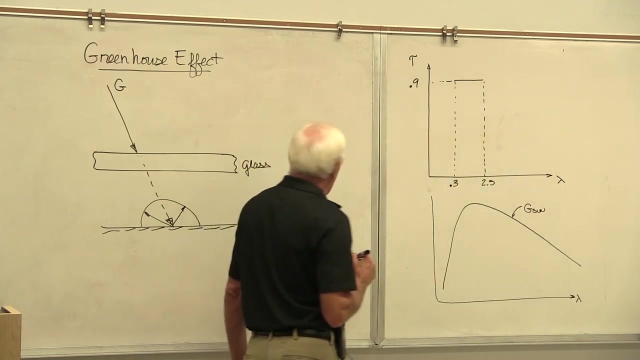 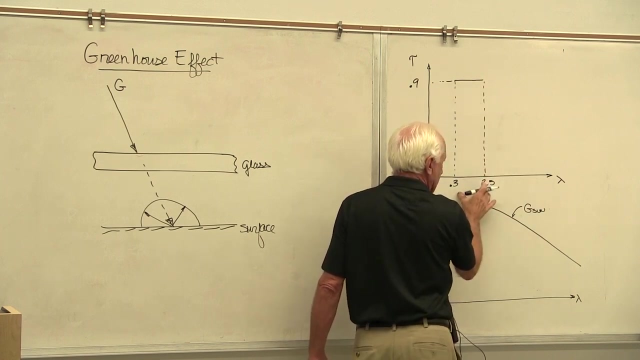 So here's what comes through. This is the G from the sun. This is G from the sun. And then, if I look at what comes from the sun, what gets through here? oh yeah, a lot of radiation gets through here. 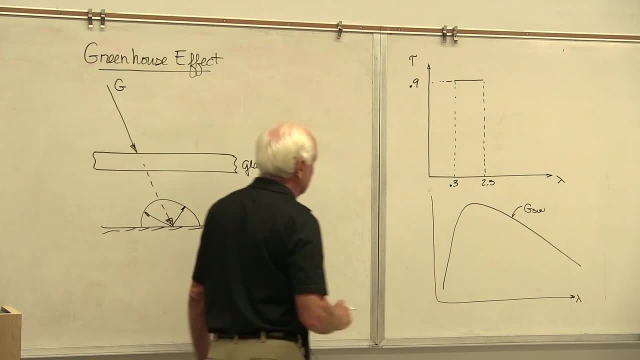 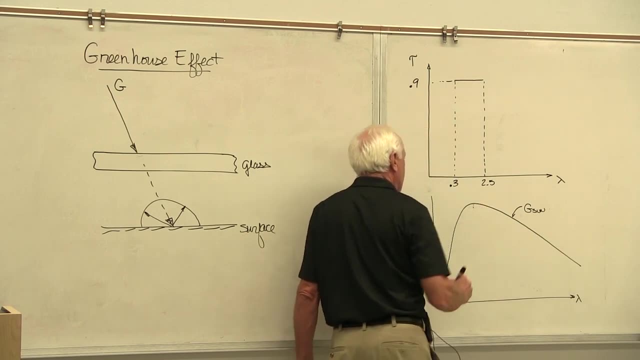 It gets through here from the sun to the glass. in those wavelength ranges of the glass, Where does this guy peak? Oh, he peaks at about 0.5 microns to 0.5, so my curve should be shifted this way more. 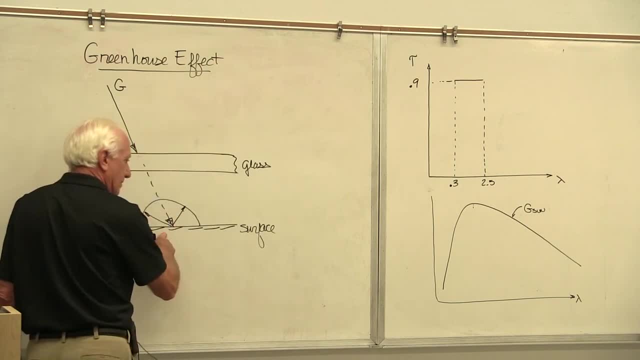 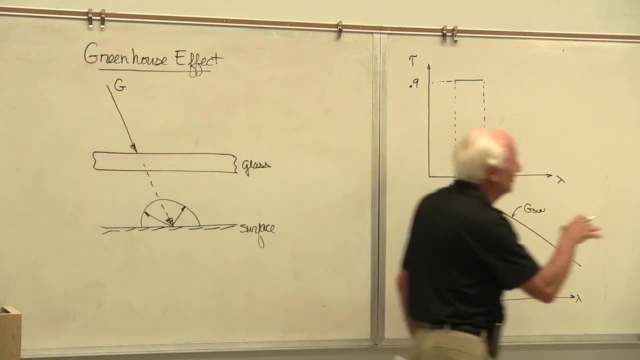 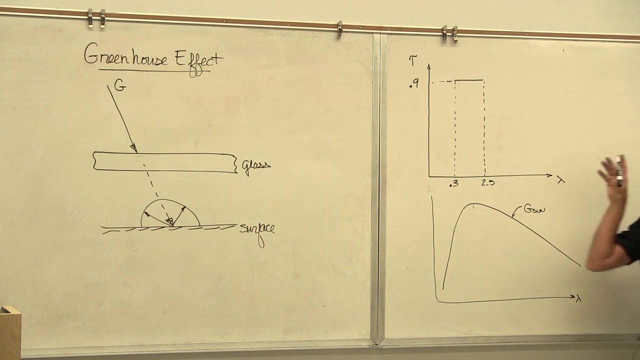 but that's okay. Now, when the black surface gets hot in your car, it even is similar to a black surface, So you can look at the shape of the curve over here in Planck's law And now pick out the temperature on those family of temperature curves. that says about: 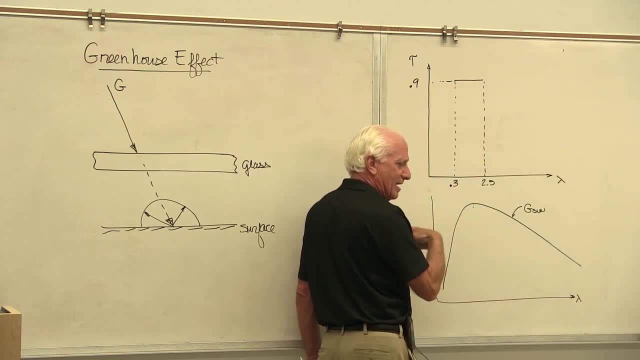 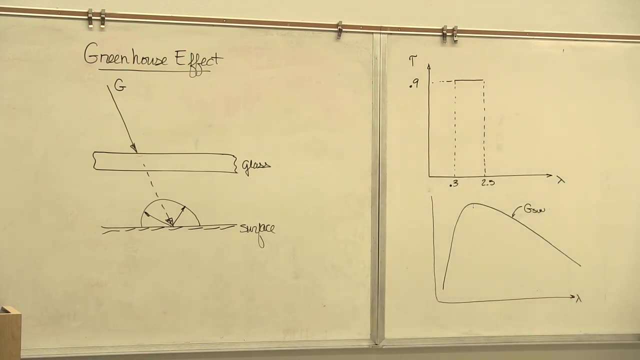 300 Kelvin, because it's about 300 Kelvin in your car, or a little higher. now Use the displacement law to figure out where the peak emission occurs at 300.. It's approximately. lambda max T is 3,000.. This guy is 300.. 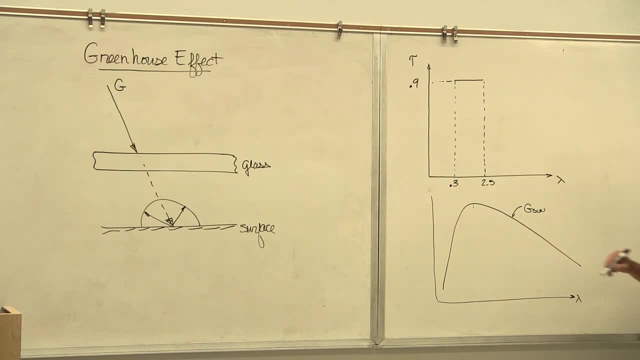 Okay. So what's the temperature? It's about 10 microns. Ooh, 10 microns. Two and a half here, 10 microns Out here There's 10 microns. That's the peak. 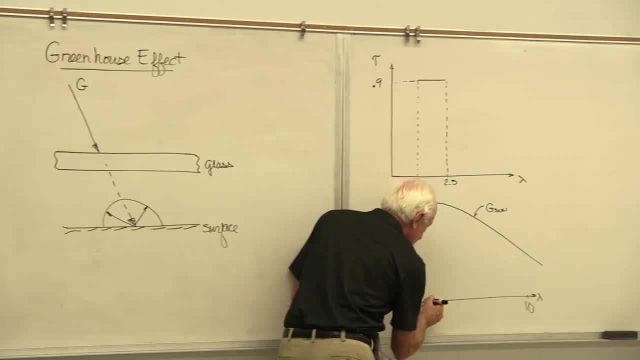 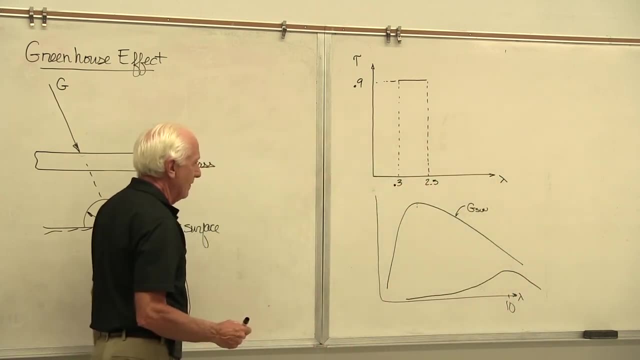 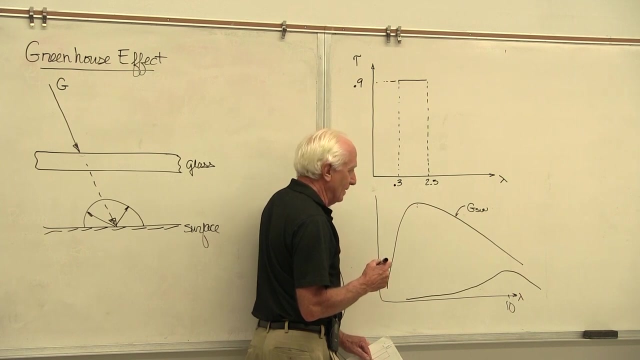 So here's where it is. It looks like that. Now look at the transmissivity, where most of the energy, the radiating energy, leaving the black upholstery or the black dashboard. Look where it is up here. I'll tell you where it is. 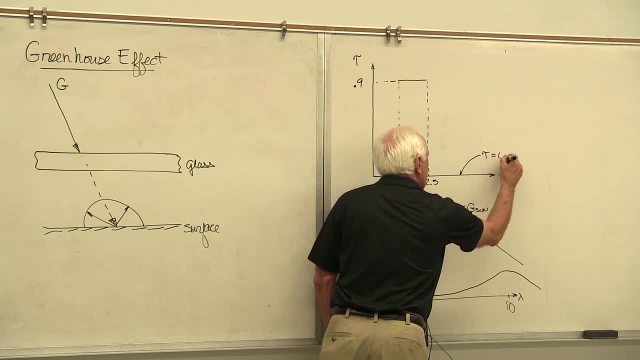 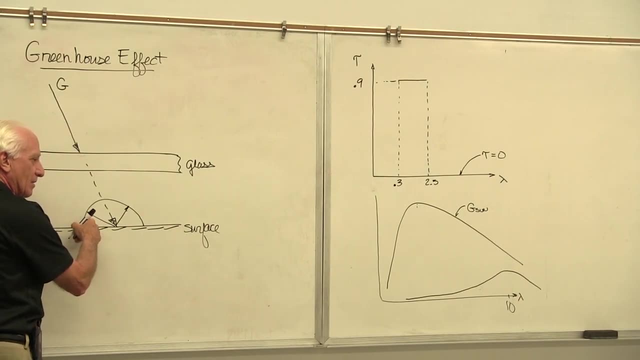 It's up here. I'll tell you where it is. It's in the region where tau is zero. When the radiation leaves that black upholstery, it sees a brick wall. It can't get out, It's trapped. So it hits here. 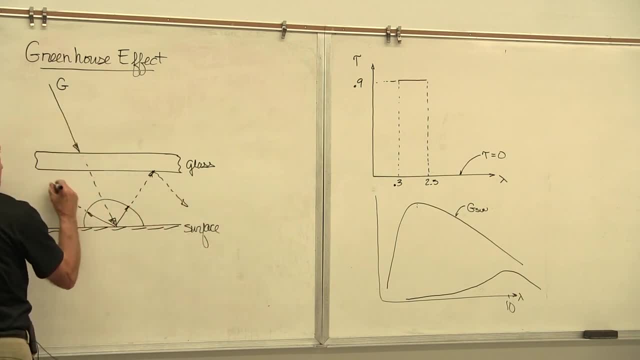 It bounces off. It goes down here, It bounces off. It goes up here, It bounces off. This is a brick wall to that radiation. What happens when we get inside the car? It gets hotter and hotter and hotter the longer it sits in the sun. 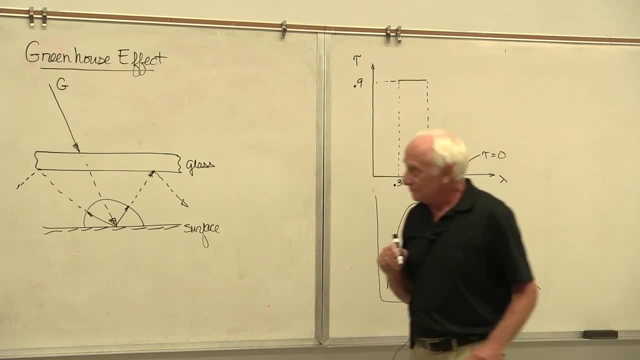 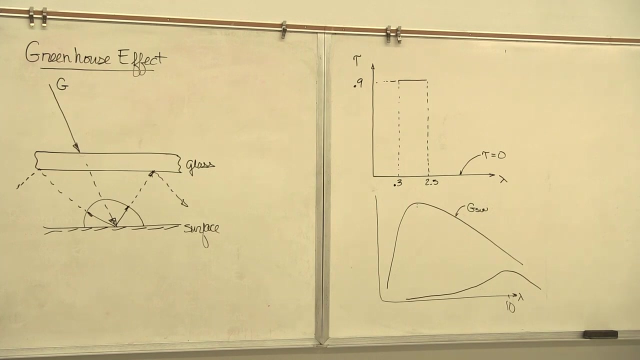 And why is that? Well, it's explained by Chapter 13,, which most normal folks don't take in education. So they understand that we're a greenhouse, but they really don't understand why it operates like that. And it's explained by the wavelength sensitivity of the incident radiation or the irradiation. 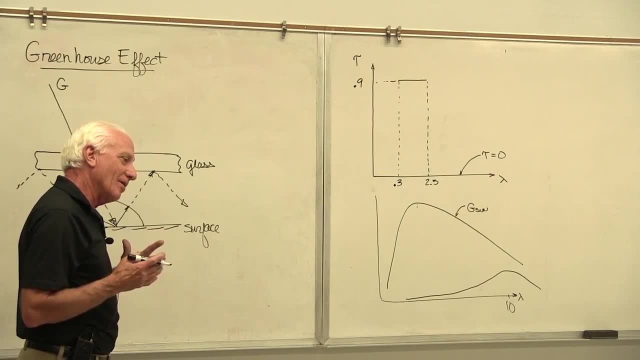 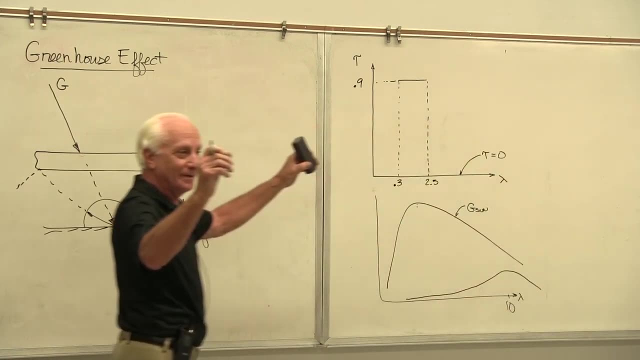 Now one way to get around that have your car getting hot is now To go out to a auto supply store and buy one of these little window deals you put in your front window, Especially if you live in Phoenix or Las Vegas or Tucson. 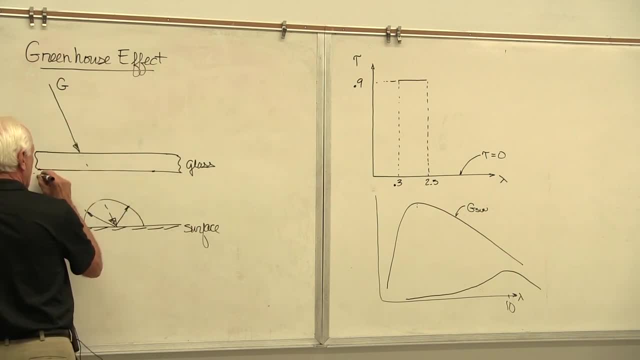 And that thing sits close to the window on your dashboard, typically up to the visors. Being an aluminized surface, it's a good reflector. It doesn't absorb. It reflits. Don't buy a black one, There's two there. 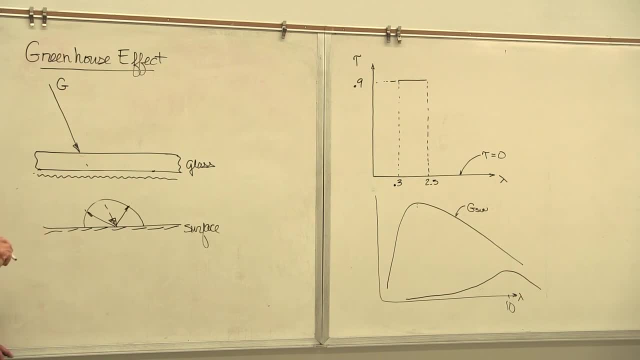 You know black and silver. Buy the silver one. Buy the silver one, Because the whole purpose is, when this radiation comes through, guess what? Bam, It goes back out again. Are the wavelengths changed? No, It's just reflected. incident. 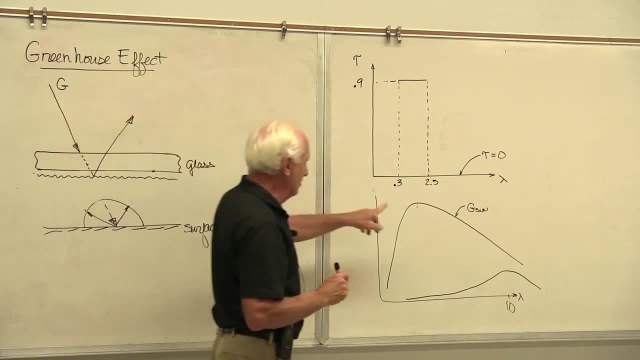 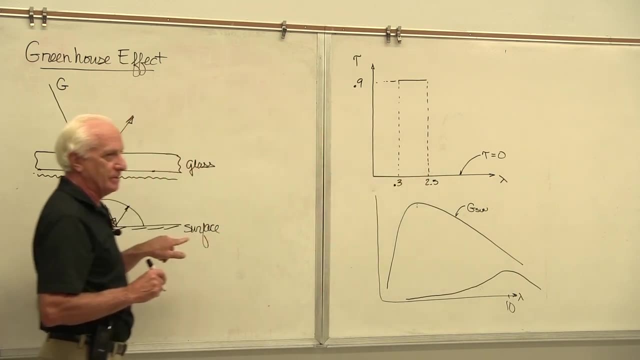 It's wavelengths aren't changed, So what goes out Looks like this shape curve, which means most of it gets back out to your glass, not to your black upholstery or dashboard. Yeah, That's why you put those guys in here. 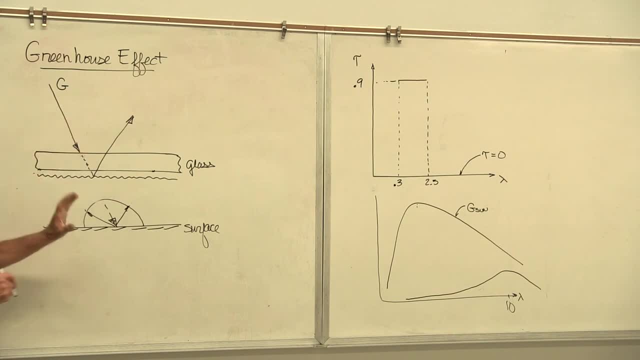 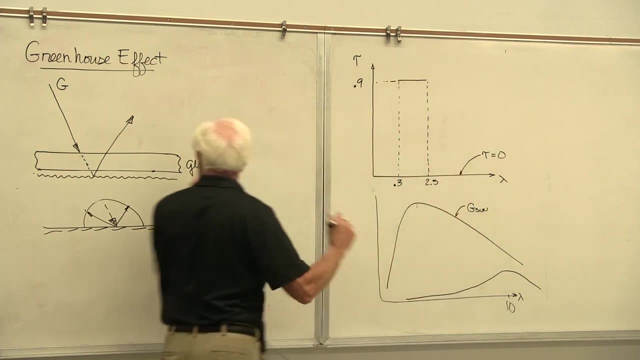 It takes the incoming radiation and throws it back out. And because the wavelengths are roughly the same and there's high transmissivity, or high transmissivity here, the outgoing radiation gets through to that This radiation. it doesn't get to the glass. 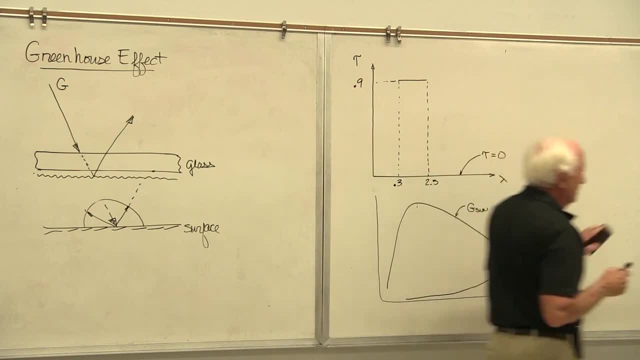 It sees a brick wall Can't get out All right. So that's the greenhouse effect on your car. Well, it works for your home too. You know same thing with your home, So certain wavelengths can escape. 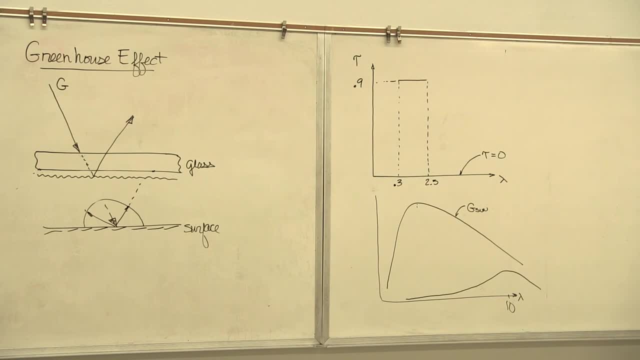 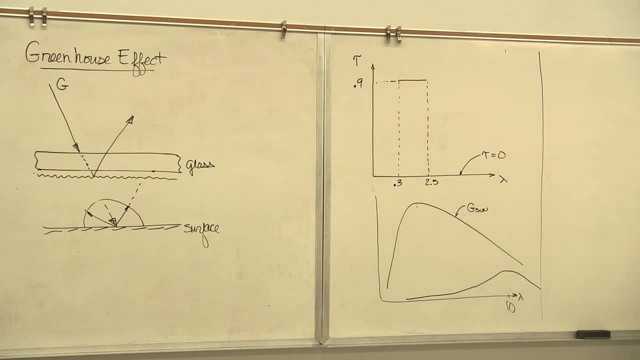 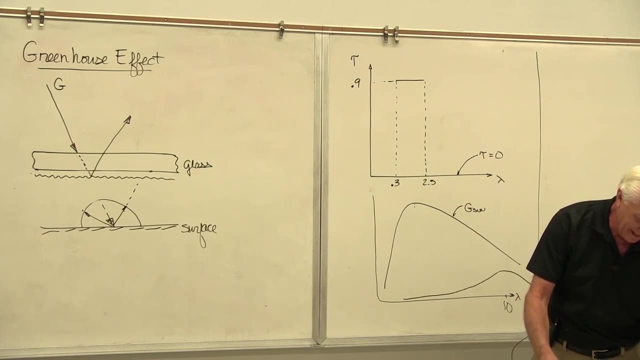 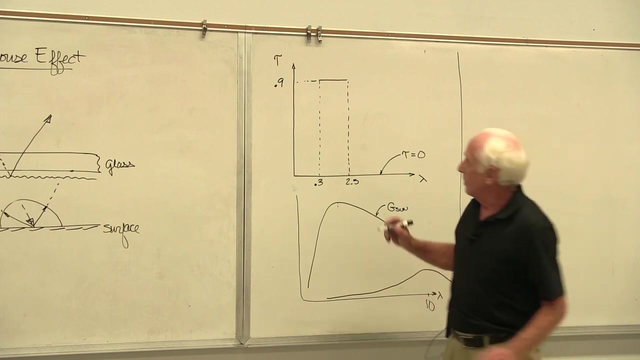 You can't get out of your car. You can't get out of your car. So you take certain wavelengths, cannot escape. Now you take, let's say you've got a fireplace, Okay, And you say, well, how does this fireplace work? 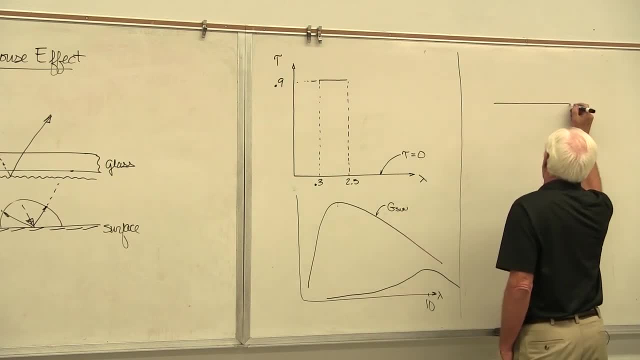 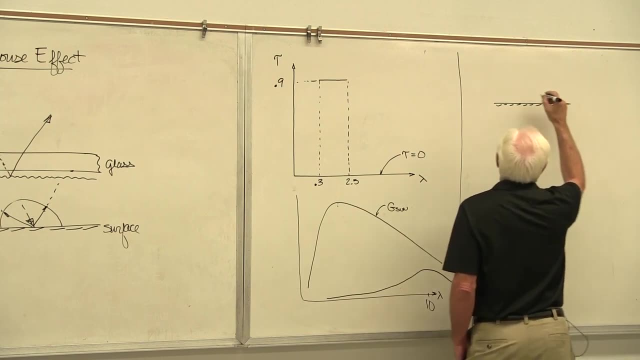 Well, let's go back in history and look at: I mean you go up and you go camping at a mammoth or a big bear or whatever you want to do, Tuolumne Meadows, And you know it's starting to get dark. 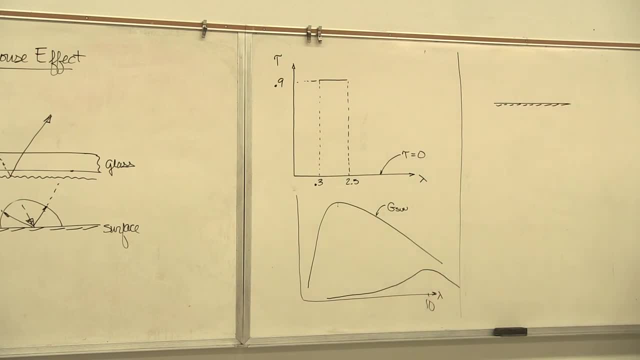 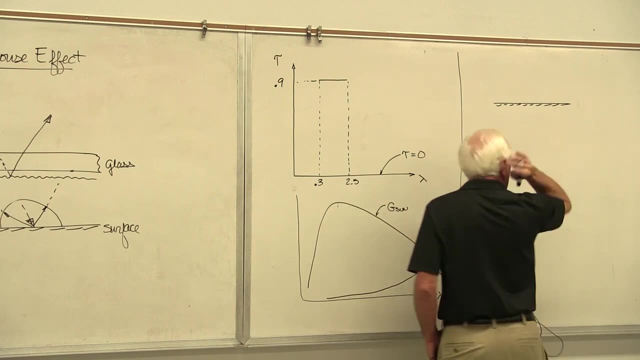 You think we better build a fire. It's going to be dark And it will be dark. the temperatures might drop down below 40s tonight. So you go out and you gather some firewood- maybe it's pine, maybe it's willow, whatever it is- and you put the logs in here and you build this big fire and everybody stands around and says, oh, that feels great, I'm getting warm. 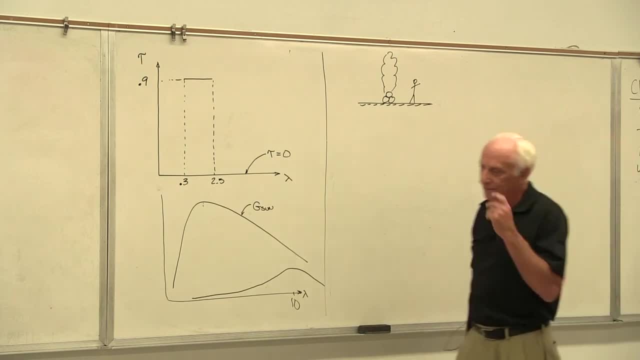 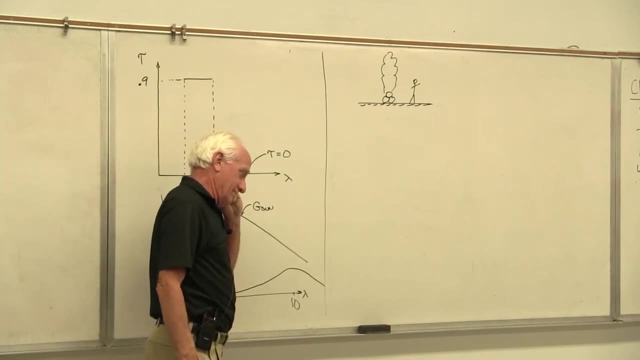 Before I jump in my sleeping bag, I'm going to get warm. Okay, yeah, I'm sure. And then the fire starts to burn down. in an hour and a half I'm going to say, hey Joe, no more fire. Go out and get more firewood. 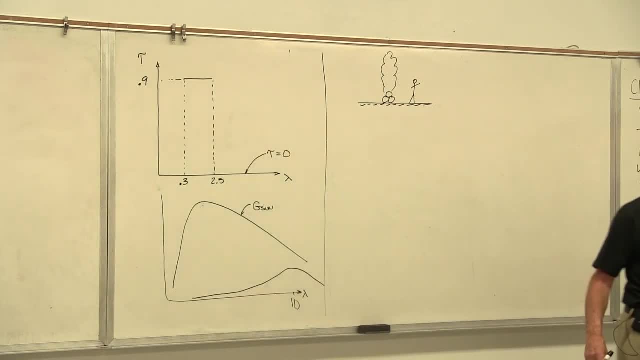 And Joe says, yeah, it's dark out there, I guess He goes up and gets more wood. He goes up and gets more wood. He's back in places again. 1045, oh, the fire's out again. All right, one, two, three jump in the bag. Okay, I'm kind of warm. Maybe I'll stay warm. 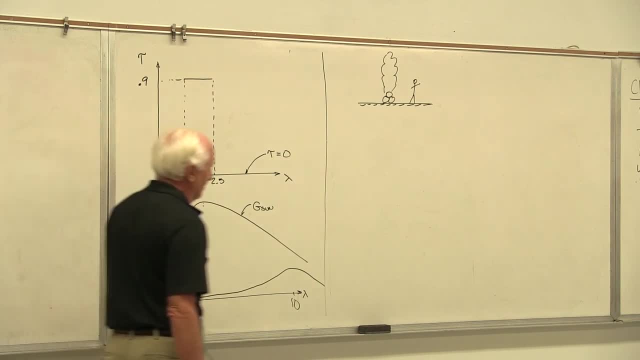 4 am. I don't think. I don't think that worked too good. I'm freezing now. Well, yeah, So what happens is? the problem is he's got a great fire. It's a fire that's six, seven foot tall. It looks beautiful if you want to build big fires. So it's going to go out in about an hour and a half or two hours. Well, they don't understand M-C's and P-Delta-T. They don't understand the storage of energy. 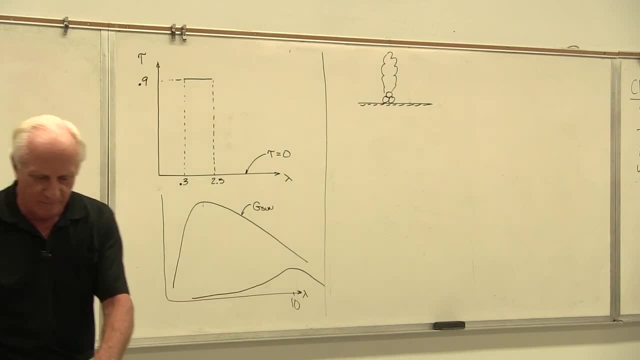 Then one guy says: you know what? I'm going to go out there and push some of these big granite boulders. Come here, Henry, help me. Push these boulders over on the fire. Oh yeah, getting smart now. 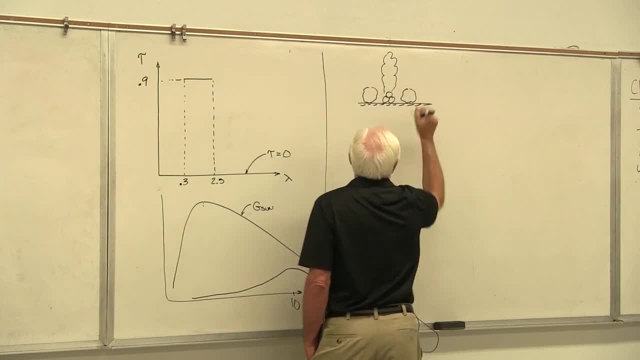 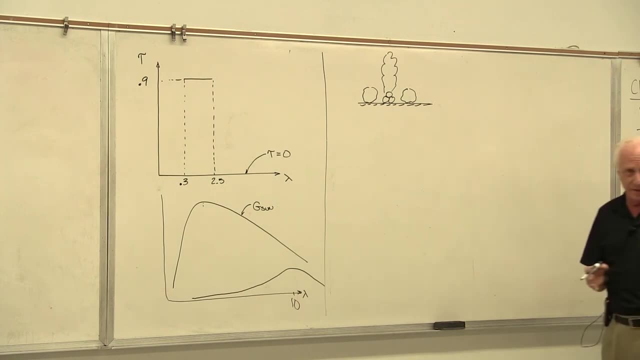 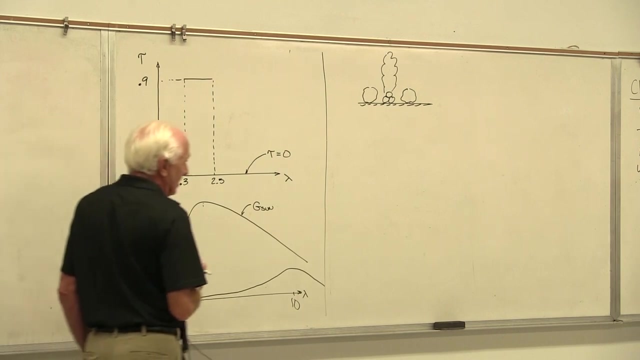 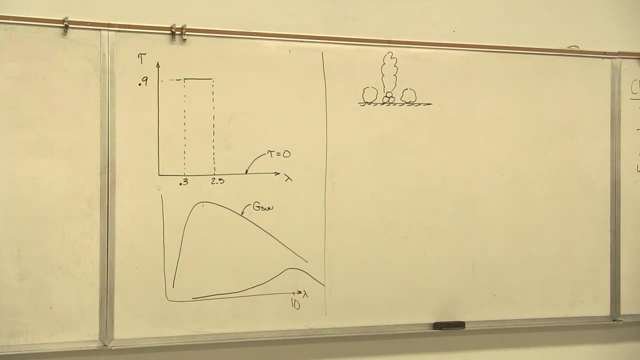 So they put this big boulder around the fire and this boulder and they enclose the fire in those boulders. They're not to sit on, although you can do that too. They're not chairs, okay, They're energy storage media. That's what they are. And when that fire's blazing like that, it gets those big granite rocks hot and I guarantee you M-C's and P, what's M Row times the volume, What's row for granite? It's big, It's heavy Row is big. 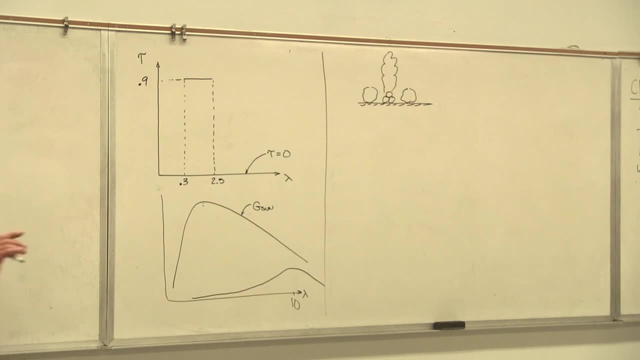 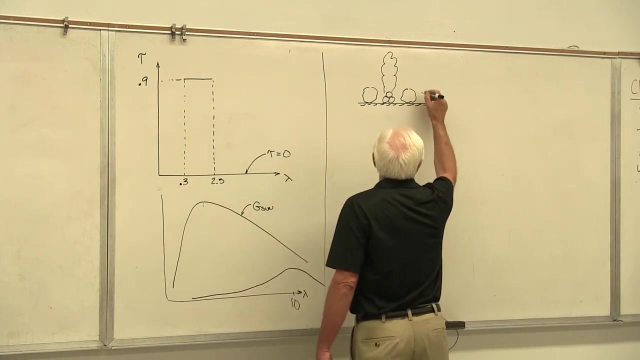 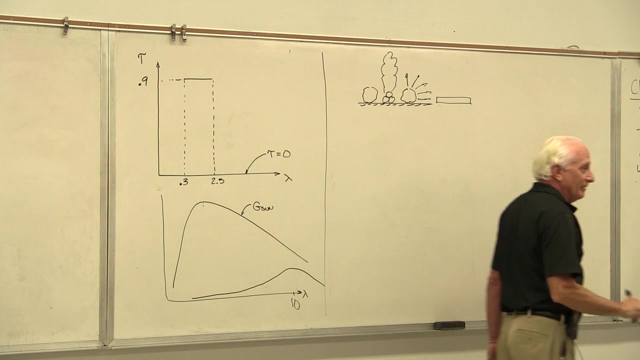 M-C for granite it's big. Multiply two numbers together. what do you get A big storage, thermal energy storage media. That thing is meant to store thermal energy. The point is this fire is supposed to get those granite rocks so hot that those rocks will be radiating heat all night long, long after that fire is out. and you're laying here close to it feeling the effects of that heat from thermal radiation. 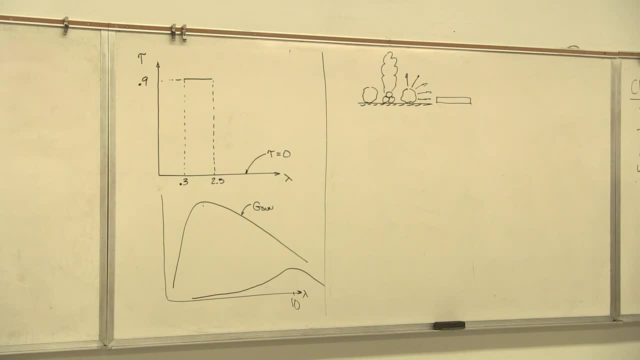 Not from convection heat transfer, Not from heat transfer. You don't want smoke in your sleeping bag, No, You want heat, and that comes from radiation. So the idea is, and if you've got a big granite wall like this, oh, that's great. 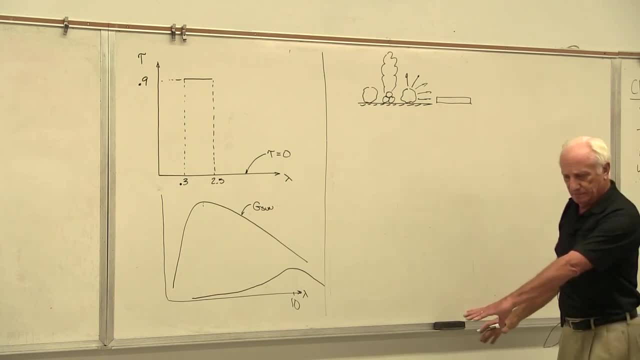 You find a granite wall six, eight foot tall, build a fire against it. that fire gets that whole granite wall hot and you're sleeping out there. oh, you'll be in pretty good shape all night long because that granite wall will radiate heat back down to your sleeping bag. 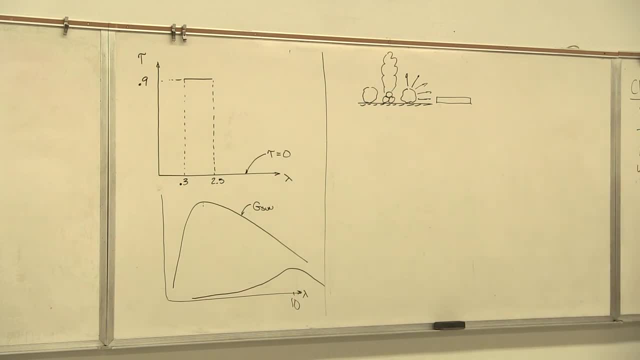 Oh yeah, these guys know how to exist in these conditions like this. Then the guy says: you know what I'd love to camp out? I'm going to try and do that in my house because I love to build a fire like that. 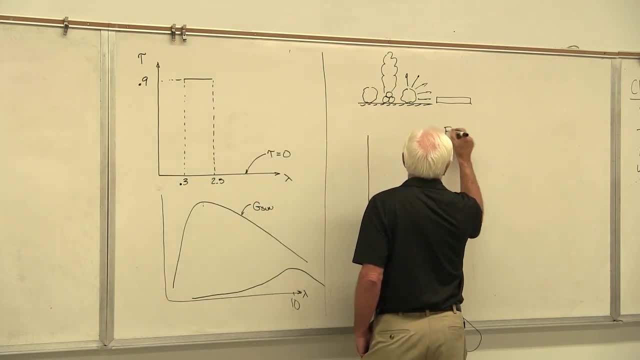 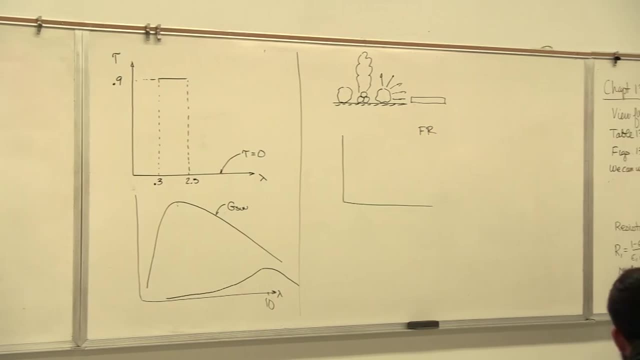 So here's your family room And the guy says, okay, I'm going to try and build a fire in there, I'll put a hole in the middle of the room and I'll put some rocks around it. No, that won't work. 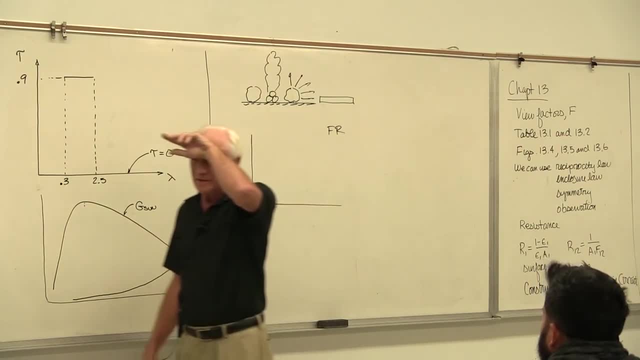 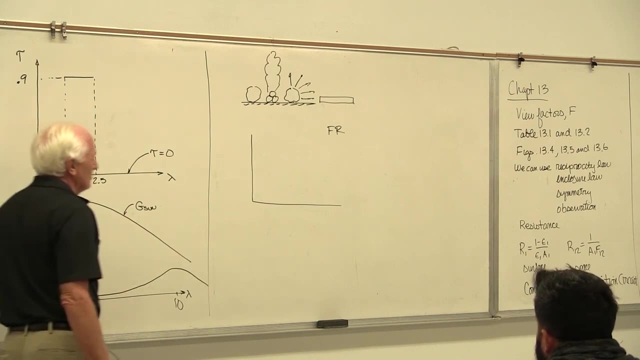 It gets really smoky in there. Things smell bad. for months You've ruined the grapes and the upholstery and the furniture Carpet has all got soot on it. No, that's not going to do that. The guy says, okay, all right, I'll build a box here then. 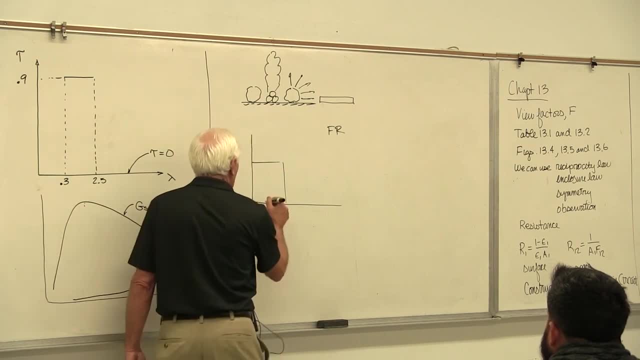 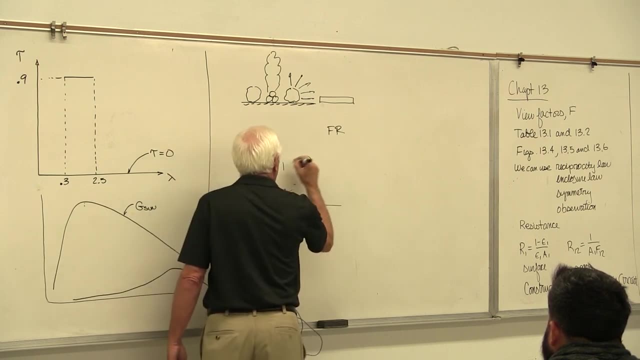 All right, I'll build a box- There's my box, all right, And I'm going to fill my fire in a box and then I'll open this so that the fire blazes and it goes up. I don't think so. 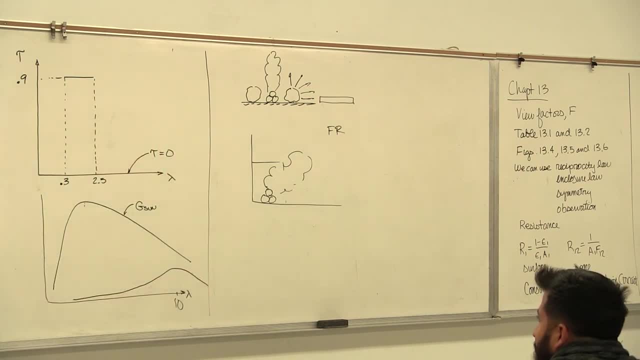 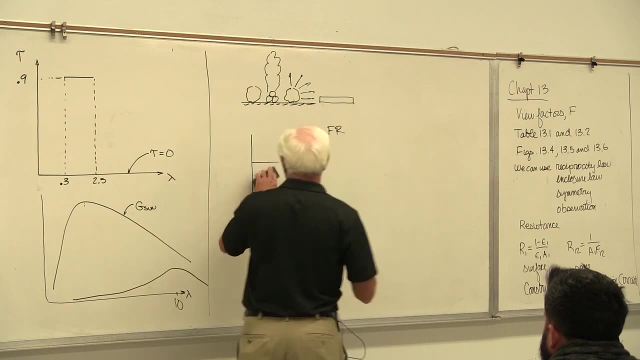 You'd be choking to death in no time. There's no place for the smoke to get out. The guy says, oh, I forgot, That's right, I can't do that. I think what I'll do: I'll punch a hole in the roof. 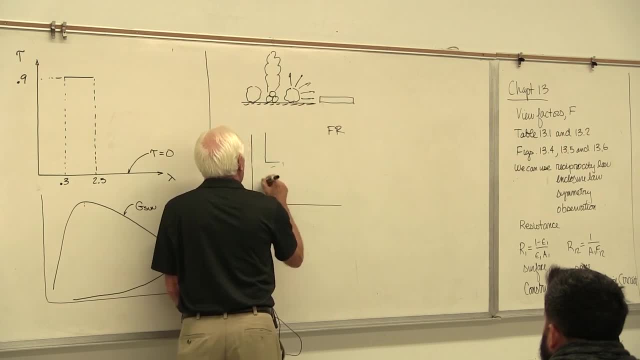 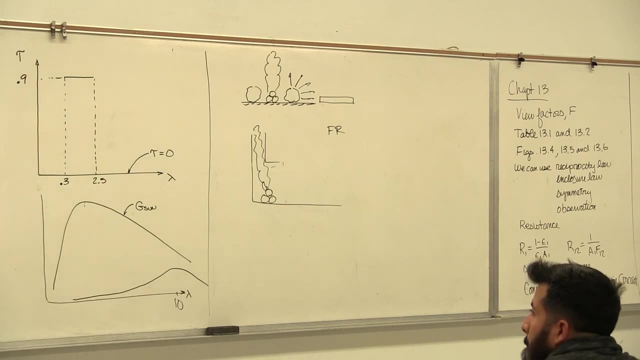 Well, maybe that's going to be a nut, But okay, I'll punch a hole in the roof And now all this stuff here goes out there. Wait a minute. now You're burning wood with a lot of energy and you're going to throw all that energy out the roof into the air around your house. 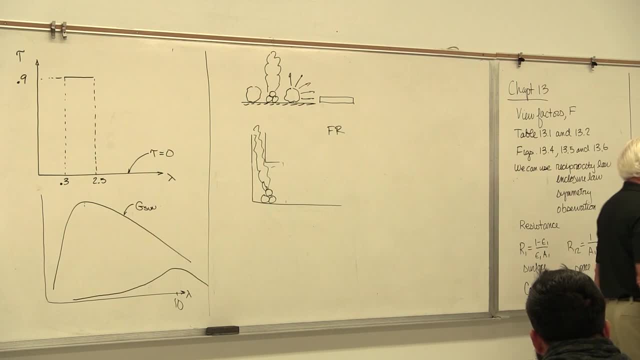 What's the point of the fire? then What's the point of the fire? He says: I love to look at a fire in the evening. It makes me feel relaxed and I love to see a fire. Yeah, yeah, yeah. 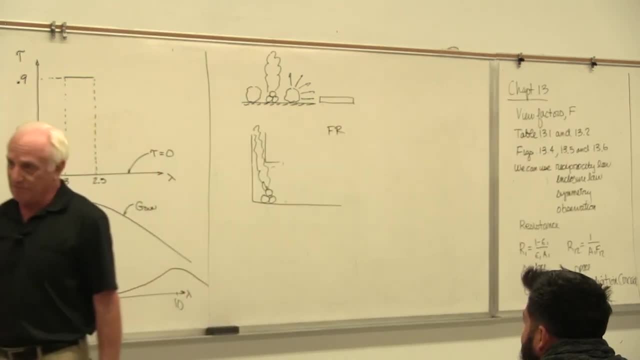 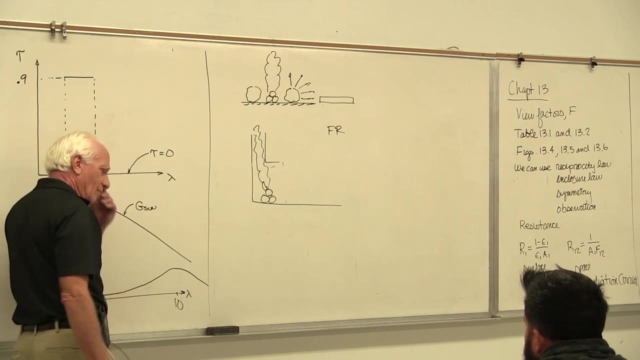 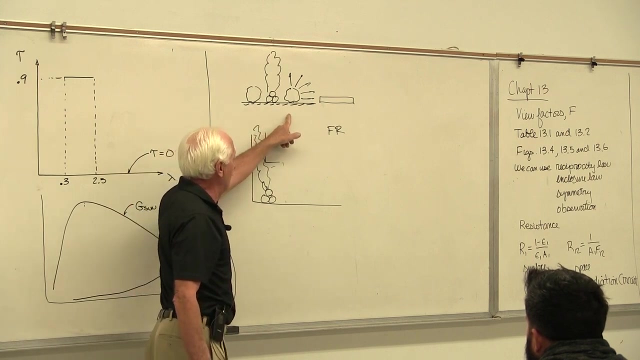 You don't live in Minnesota. You live in Minnesota. They say I have to have a fire or this house gets real cold. And I'm like okay. So the guy says you know what, When I went camping I put big rocks around my fire pit here. 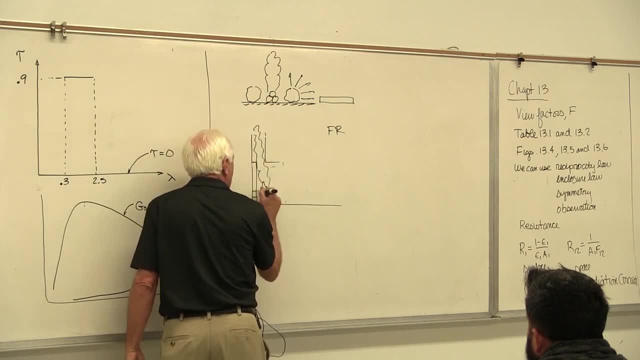 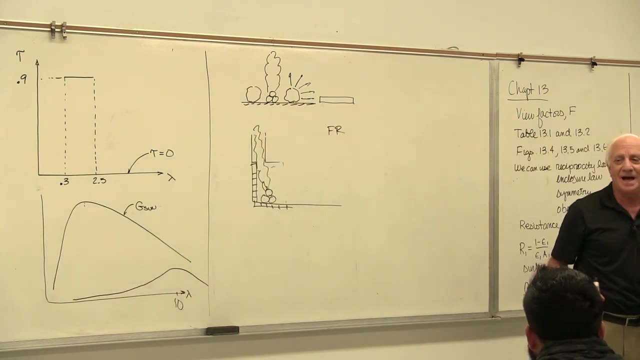 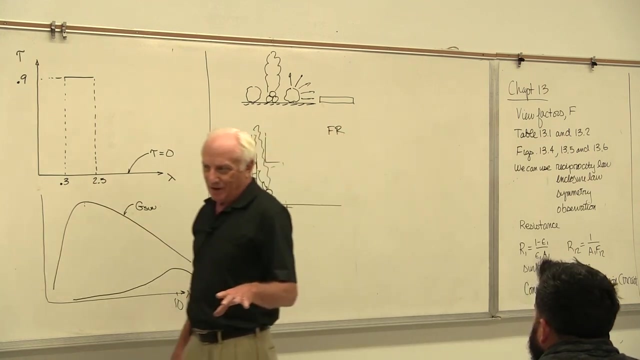 I'm going to put fire brick in my fireplace And that's like something to store heat. Now you got it. Now you got it. The whole point of a fireplace is to have a flame for a while To heat up that fire brick. so when the flame goes out, the fire brick is still very warm. 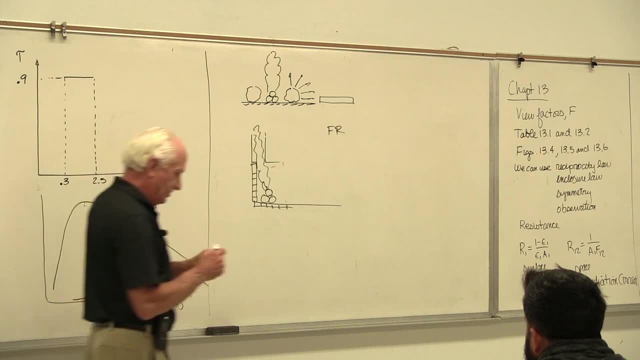 I've got one block wall in my backyard. It faces due west on the sunsets. It's got a pretty good sunset- the old trees. that wall faces west sunset And I walked up to that wall in the evening after the sun went down and put my hand on that wall and stood by it. 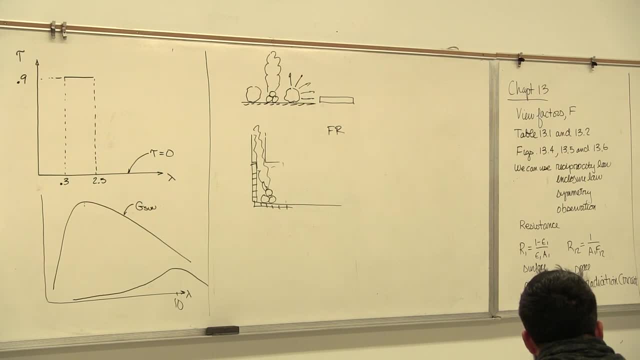 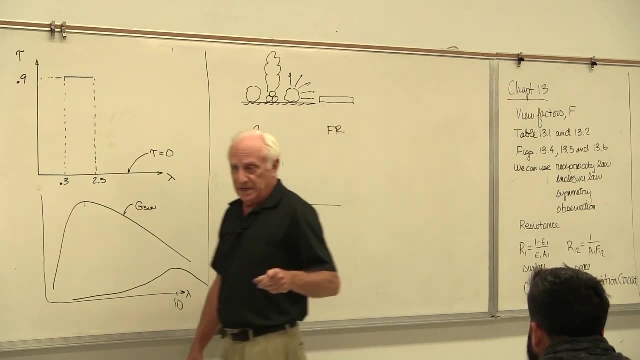 Boy, I could feel the heat coming out of that wall and my body here and my hand. It was radiating heat to my body Because that cinder block wall was storing heat from the sun, hitting it at 90 degrees close to sunset. 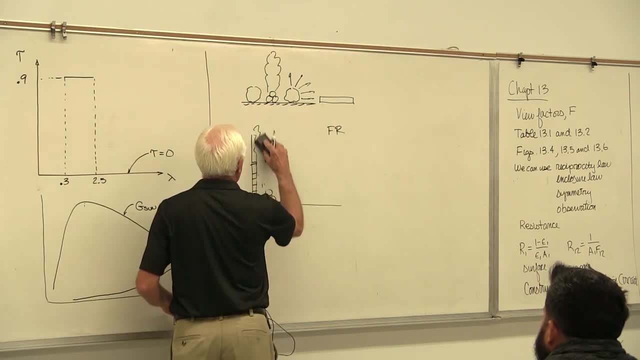 Same thing here. The fire goes out. See, oh gee, that's not too bad. No, it's not too bad, Because now this is all cinders at the bottom, Now this thing is radiating heat to the carpet, to the sofa, to the walls, and that room stays warm. 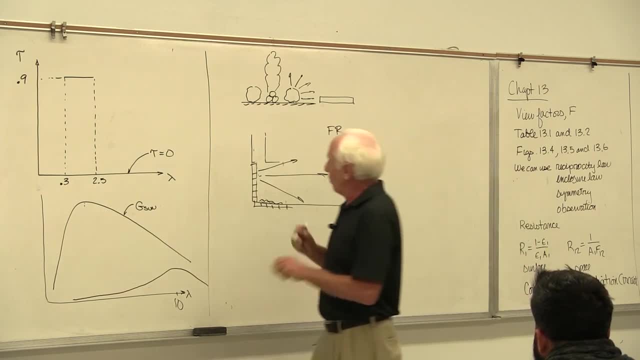 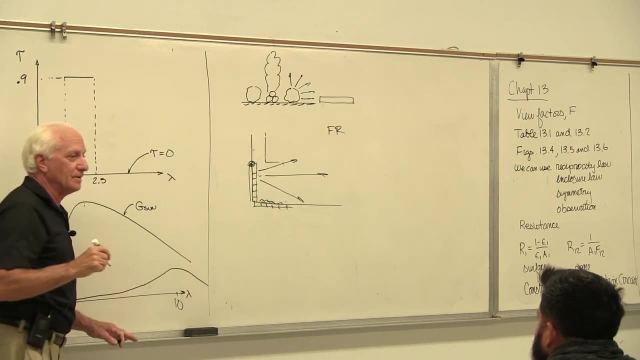 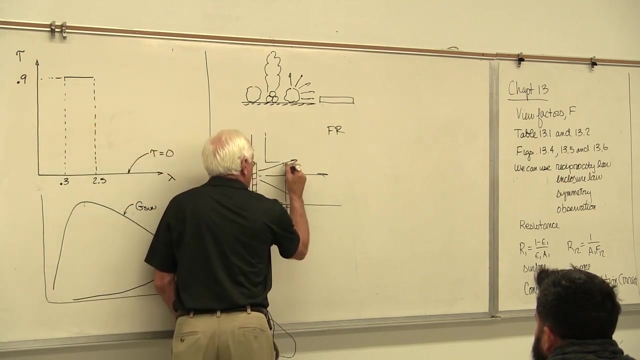 Okay, There's even some homes in Big Bear. They put water pipes behind here with a valve up here and they preheat their water for the hot water heater from the fire brick on the back side. Okay, Some people put here glass pane with a little air blower and they blow cold air. 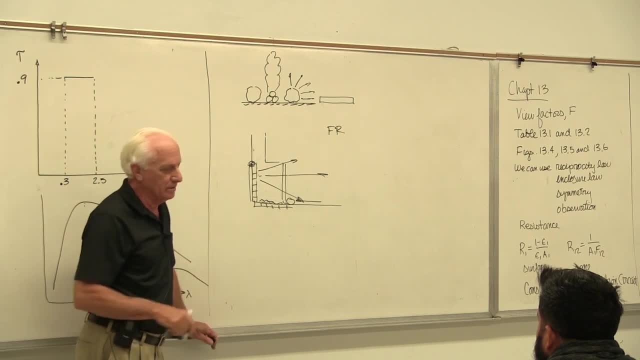 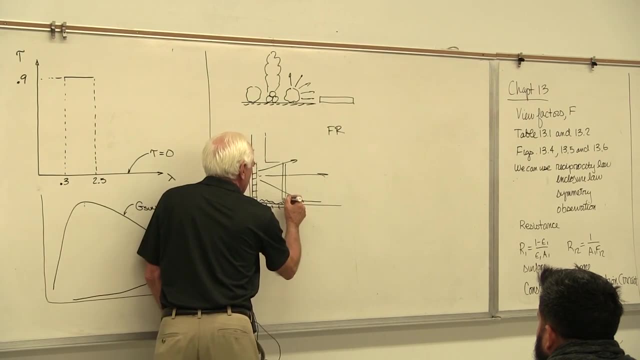 Where does the cold air come from? The floor? That's the coldest air down there. Baby. have a little air blower here. plug in the wall, Cold air comes in. It gets heated by the glass pane here. comes out the top, blows in the room, heats the room that way too. 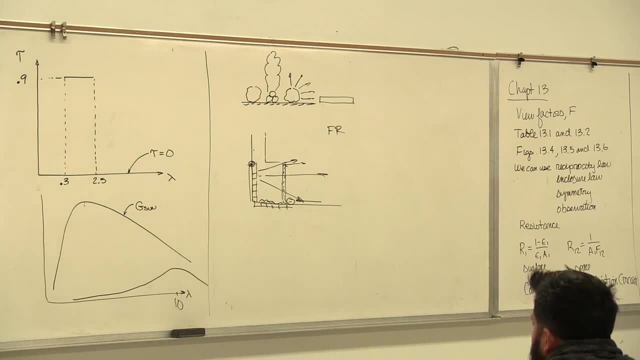 There's all kinds of ways to conserve energy that way. So yeah, that's the purpose of the fireplace. The real purpose is to heat an energy storage material. so when the fire goes out, the heat will keep coming in the room for a long time after that fire goes out. 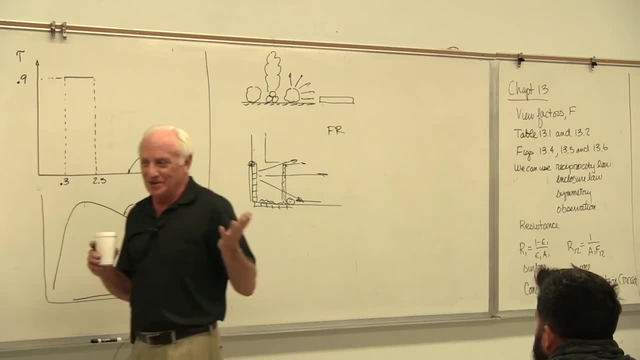 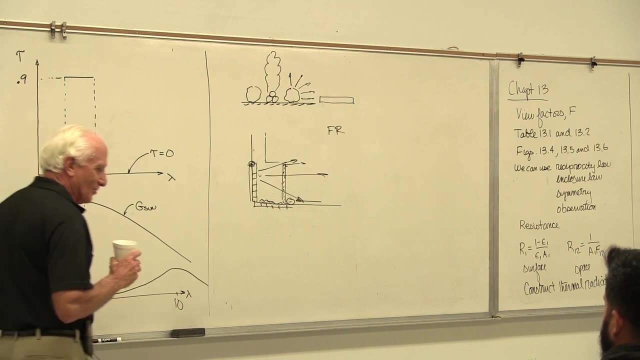 Okay, So these are just stories to tell you about why heat transfer is such an interesting subject. You can relate it to so much in your industry. You can relate it to so much in your everyday, daily life. It just makes it that much more meaningful as a course. 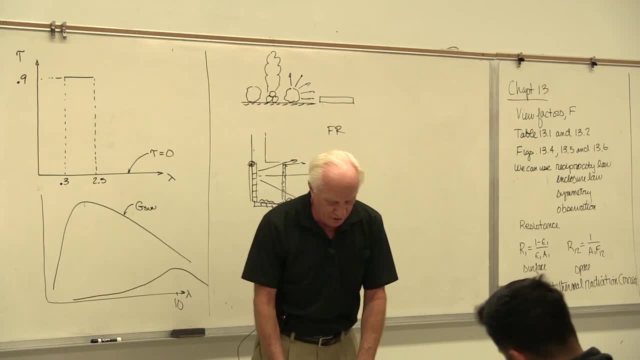 We're going to stop here and do a course evaluation. If you need to, you can use the back side of the farm for any comments you want to make And then, if you want to take that back to me when you're done, I'd appreciate that. Thank you, Bye-bye, Bye-bye, Bye-bye, Bye-bye.